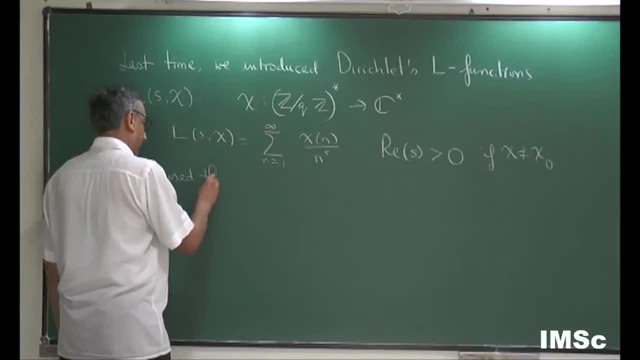 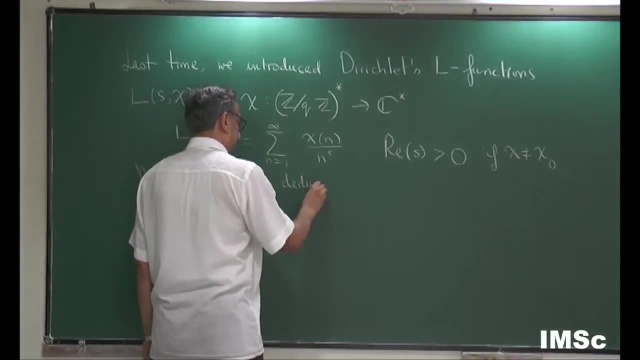 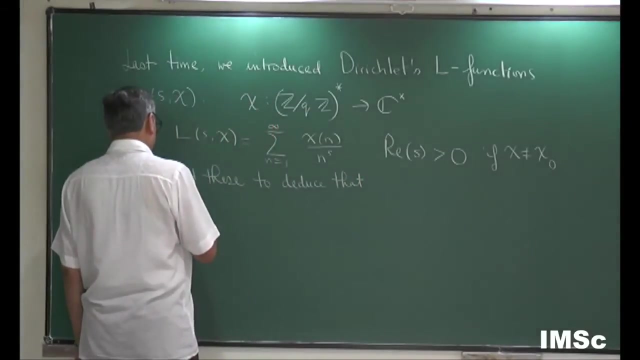 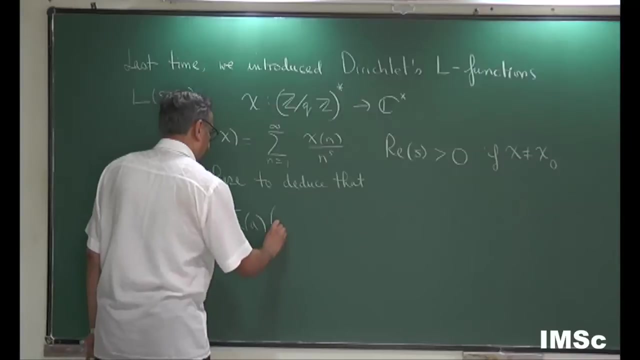 We use these to deduce that if I take the combination summation chi bar of a minus L' of s chi over ls chi Um, OK, If Subm the 1960.. you I ds sum wh i我就ados def Mst. 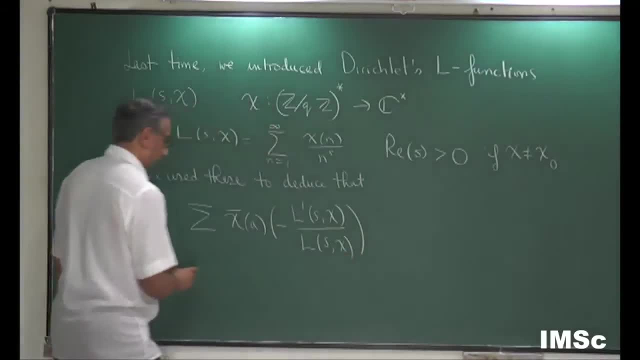 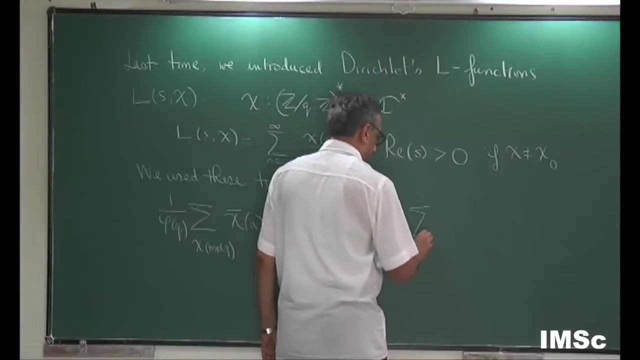 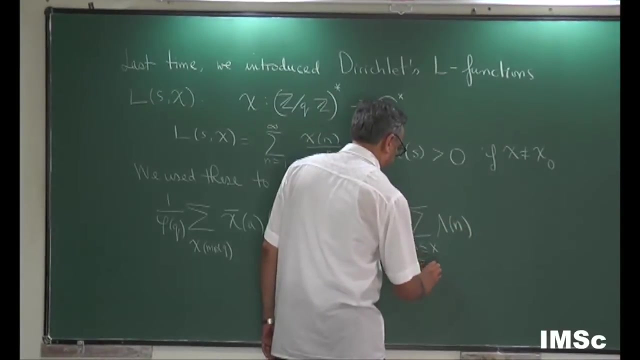 If I take this combination and sum over the characters chi mod q- so when I write this I'm talking about the characters, the character group of this thing- and when I divide by phi of q, we got that this is equal to summation: n less than x lambda of n. n congruent to a. 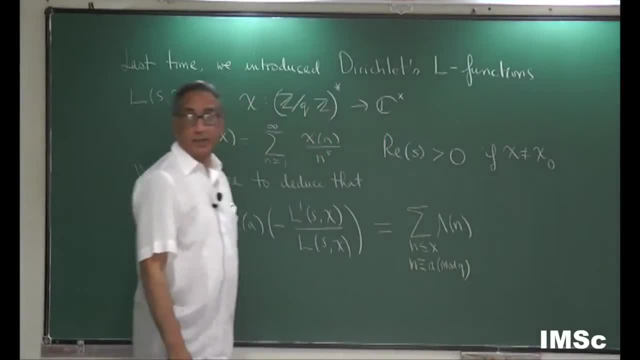 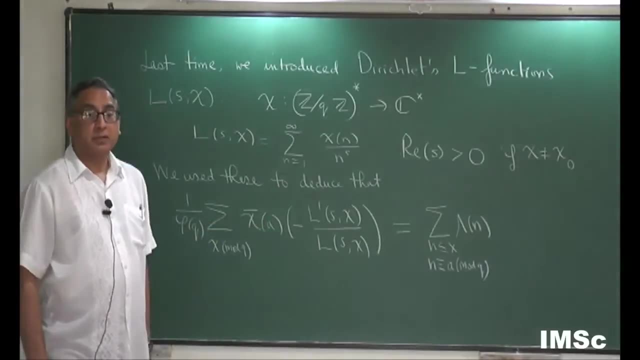 mod q. This is what we got last time. So on the right hand side we have essentially primes in the progression, a mod q, and the left hand side we have this chi mod q. So on the right hand side we have essentially primes in the progression, a mod q, and the left hand side we have this chi mod q. 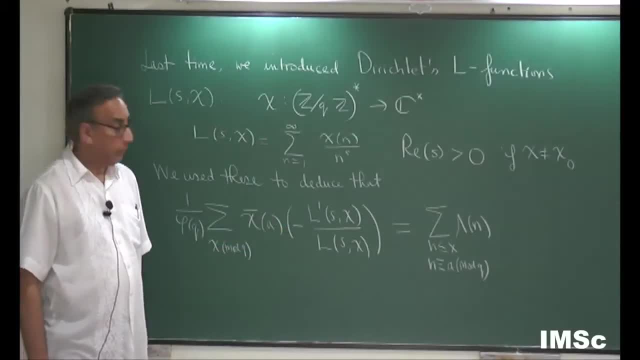 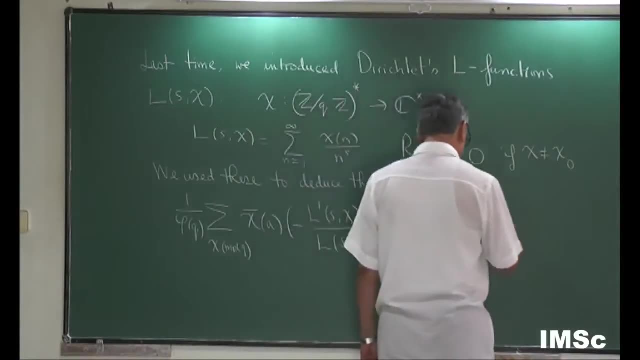 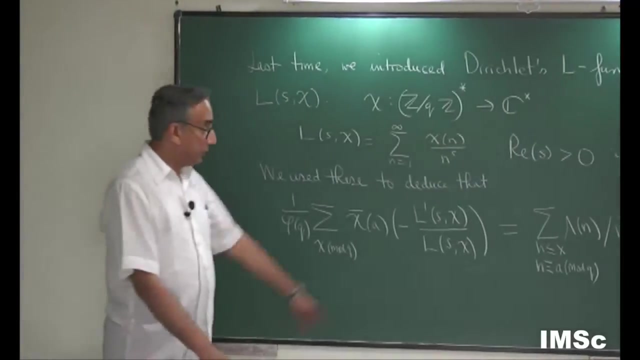 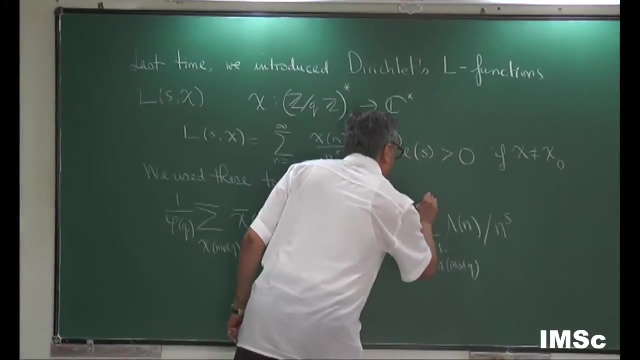 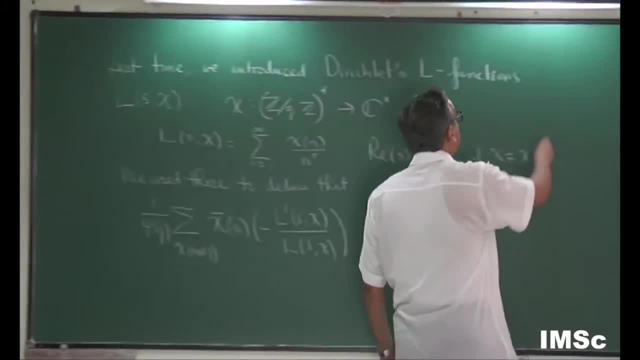 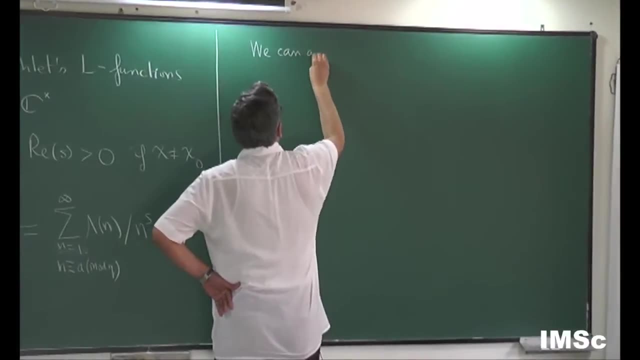 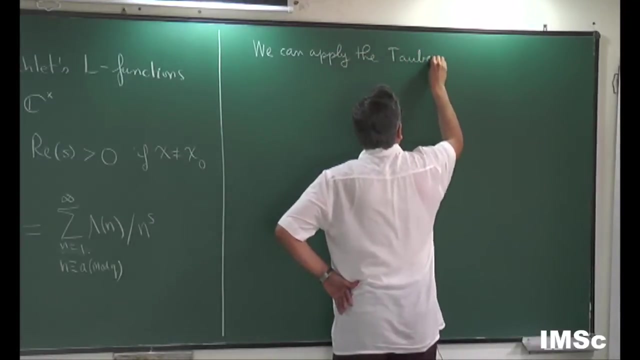 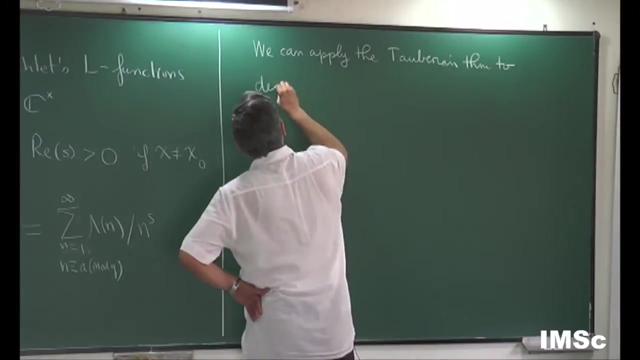 like to now deduce. we can apply the Tauberian theorem to deduce, deduce what deduce something about the partial sums. so the Tauberian theorem tells me if you have a Dirichlet series with non-negative coefficients, or even it doesn't. 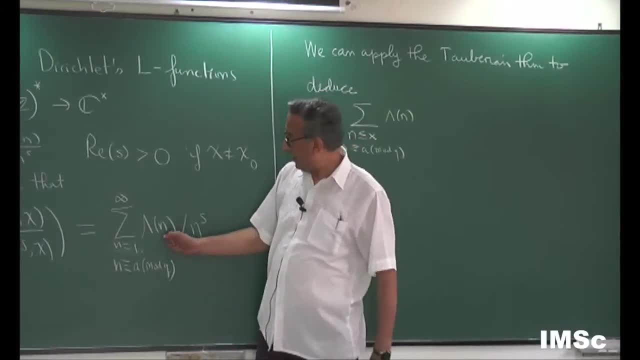 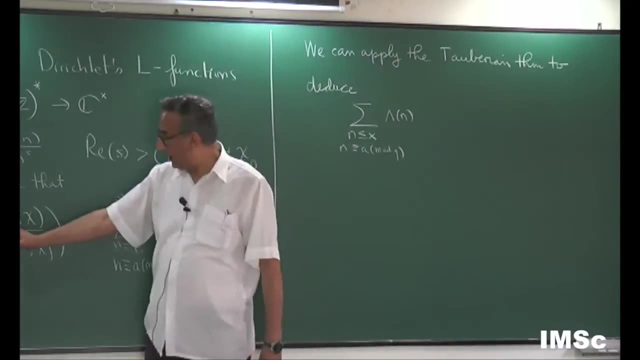 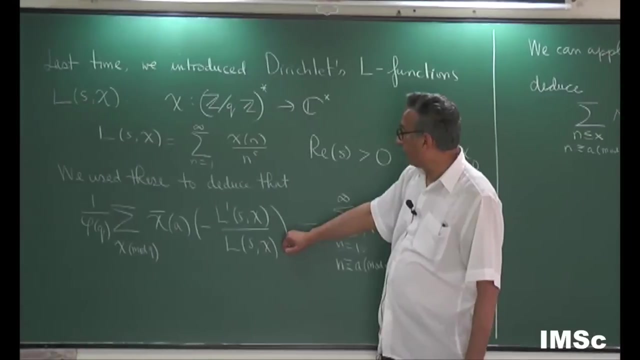 matter complex coefficients. we went through that discussion with some suitable properties that This Dirichlet series now is the same as this Dirichlet series. from this Dirichlet series we deduce that this has analytic continuation for real part of S greater or equal to 1, with 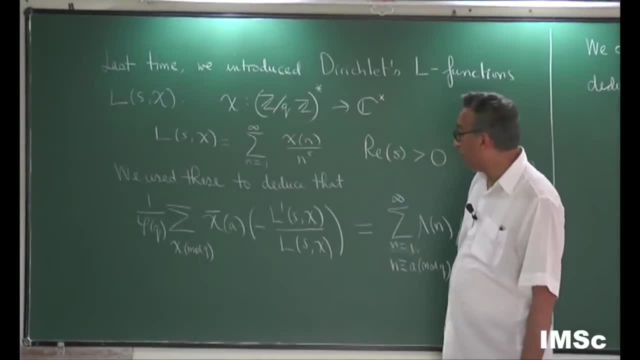 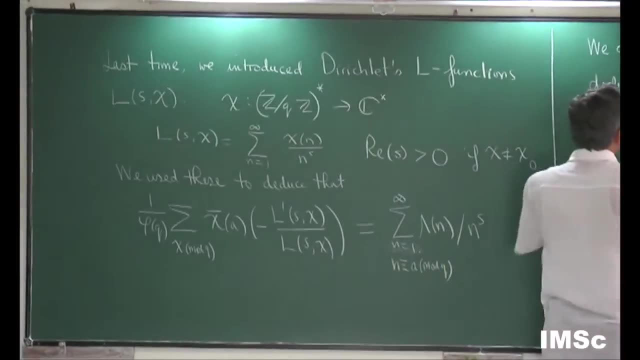 a simple pole at S equals 1, with residue 1 over 5 Q, except we need to know that these guys don't vanish on the line. real part of S equals 1,. okay, So we can apply the Tauberian theorem to deduce this. 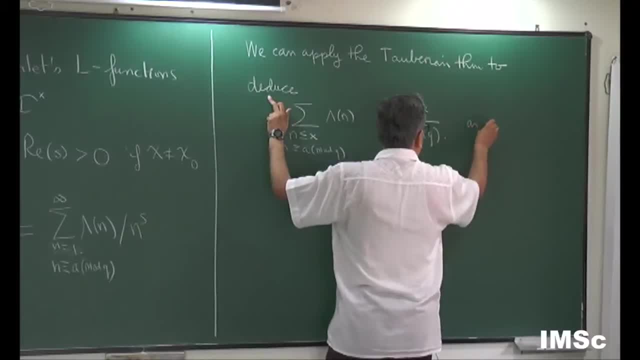 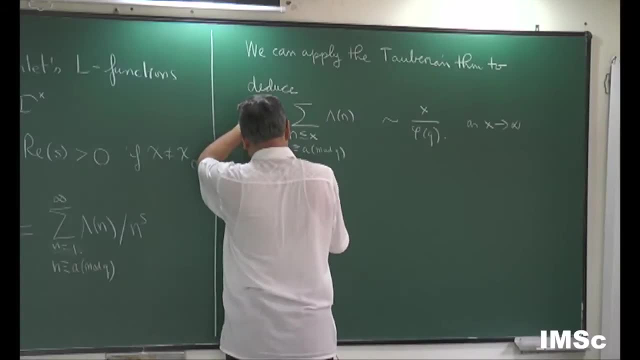 Okay, So I'm going to do a little bit of this. we need to know that. you know I'm going to do a little bit of this, I'm going to go over here. So we need to know that this Dirichlet L function has X, tends to infinity, provided the Dirichlet. 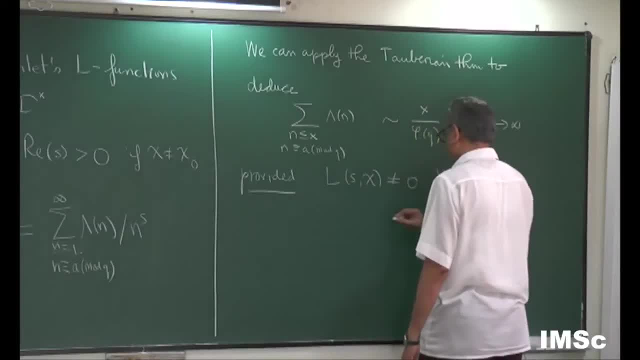 L function is not 0 for all. chi for real part S equal to 1.. So we need, we need this, We need the non-vanishing. So we know that for chi equal to chi naught, That's not true. 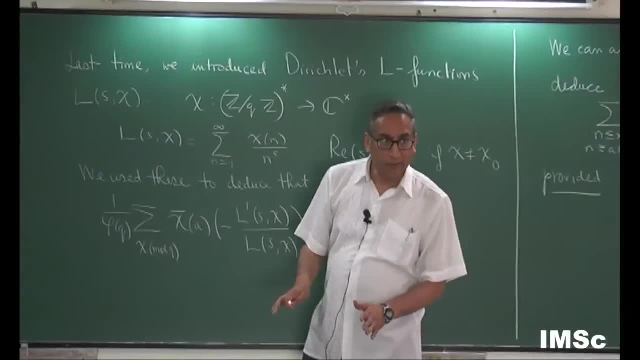 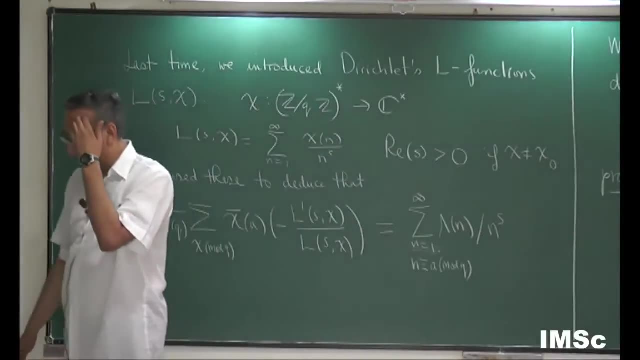 This is not true. really, the zeta function that we know, we've already proved that it has no zeros on real s equals 1, but now we need to prove that for the other characters there are no zeros on the line real s equals 1,. that's what we need to prove. 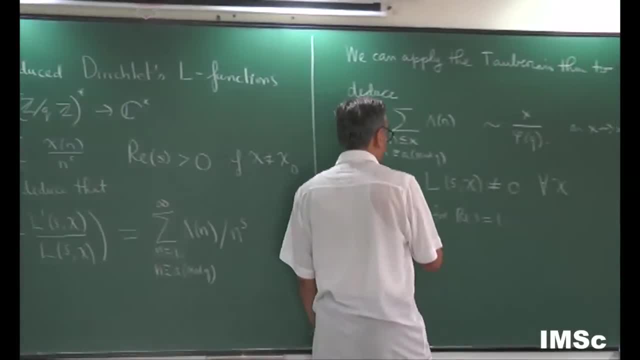 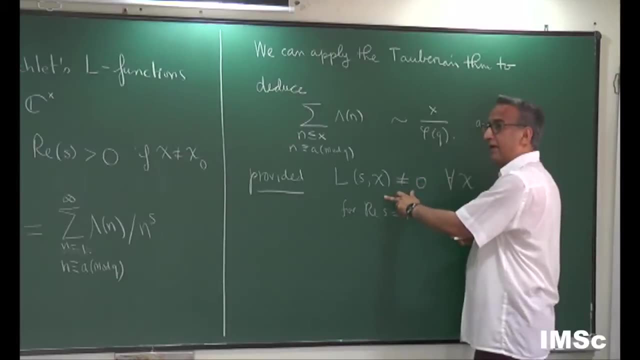 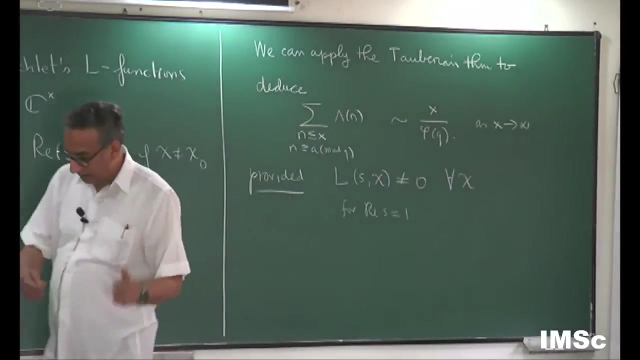 So this is the critical part of the proof. somehow a theorem of this type of primes in arithmetic progression translates itself to some sort of non-vanishing of an L function. and that's what this kind of symmetry between non-vanishings of L functions and asymptotic. 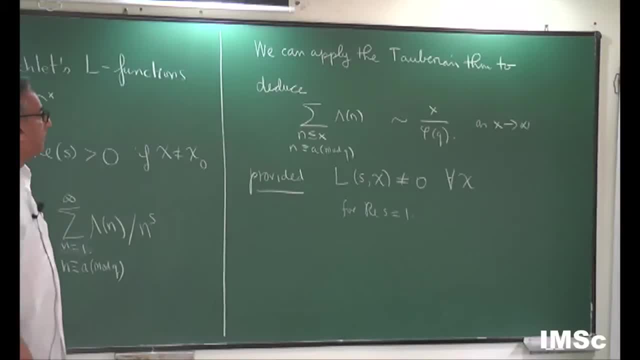 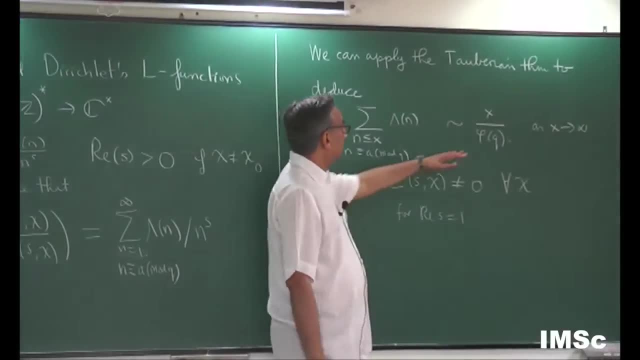 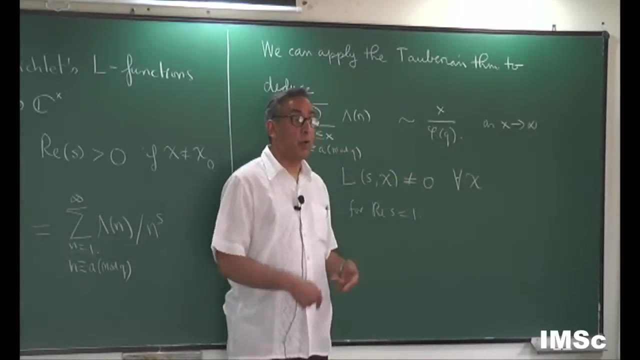 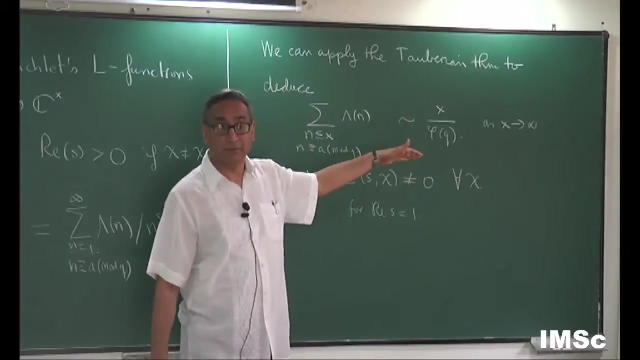 statements are common in number theory, So this is what we need to discuss today. Everybody okay that this is essentially the prime number theorem in arithmetic progressions, Because the contribution from squares, cubes and etc. is small, And so the main thing is really coming from the primes and not prime powers. 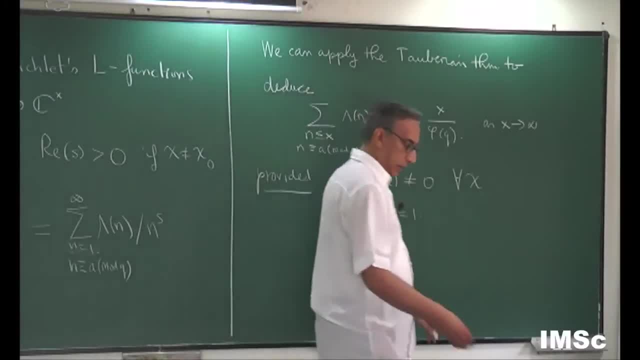 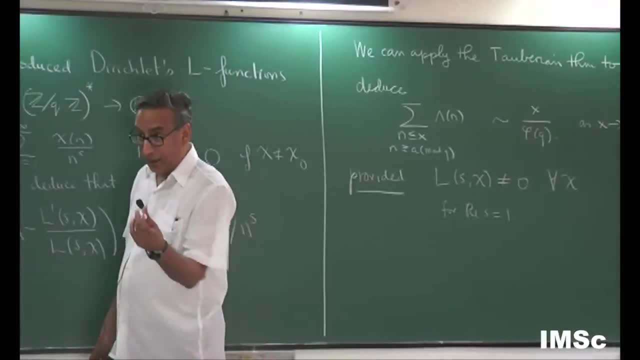 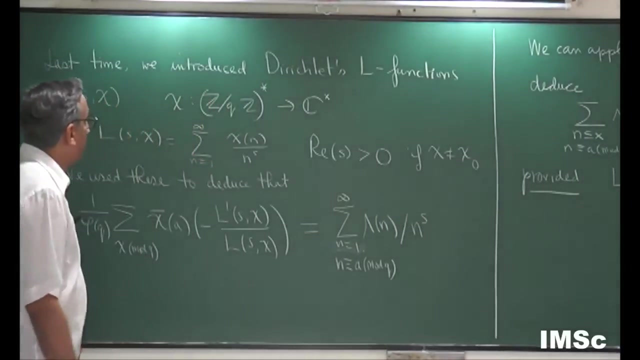 Everybody okay with that? Yeah, okay, All right. so now this non-vanishing result. as I mentioned last time, Dirichlet had a tough time doing that In 1837, he took a couple of years onwards and did it really in a very complicated way. 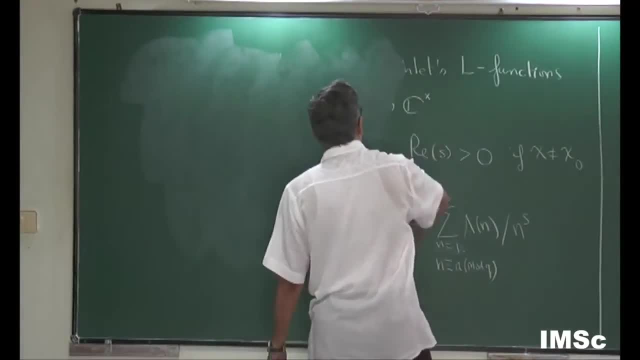 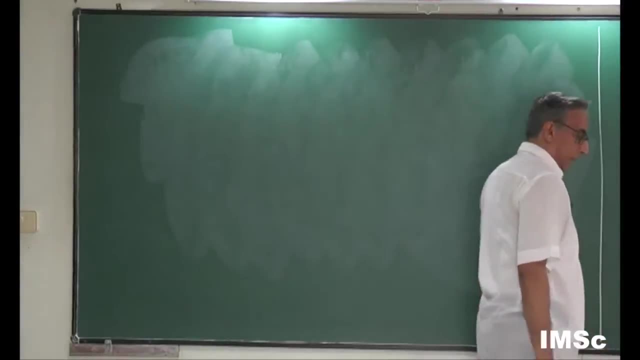 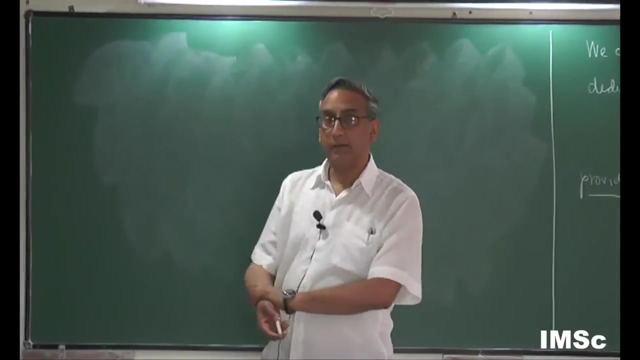 Of course, as I mentioned many, many times, I'm sorry. I'm sorry. It's not necessarily the result that we're after, but rather the proof. We're trying to look for methods, So Dirichlet's efforts in trying to show that these L functions didn't vanish, of course. 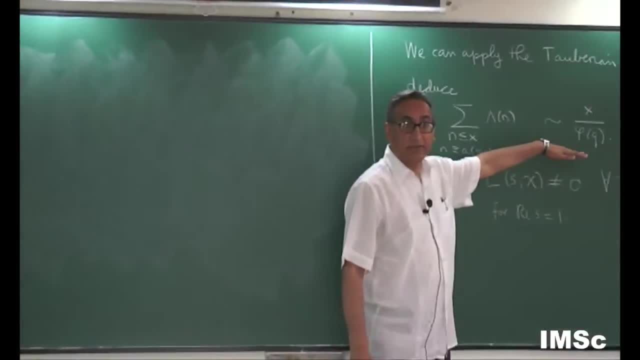 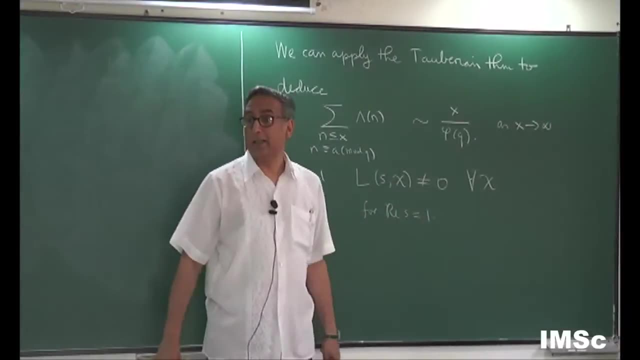 he was not after the asymptotic formula, He was only after the infinitude. And for that you don't need all this tight information. It suffices to know L1 chi is not zero, because he was only showing a very weak state. 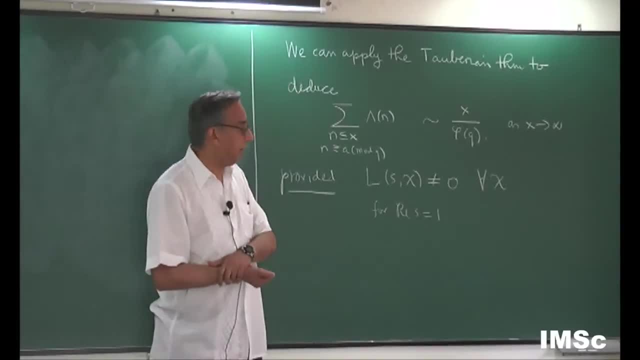 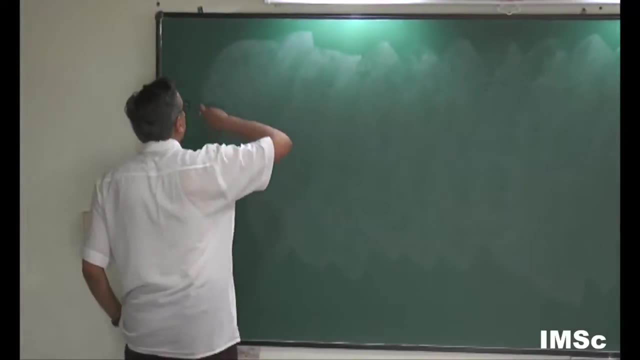 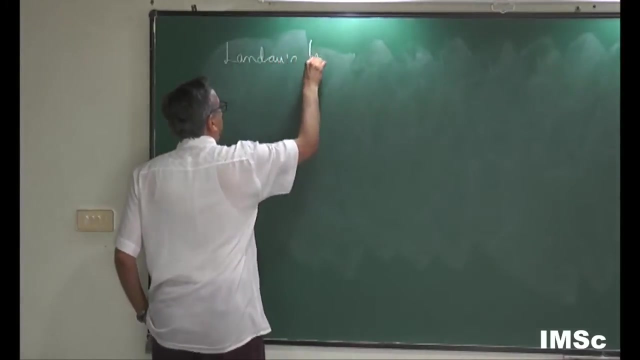 He was basically showing the divergence of a certain series. Okay, so the easiest way of handling this problem is using what's called Landau's Lemma, a very important lemma in mathematics, in number theory in particular. And it's a very important lemma. 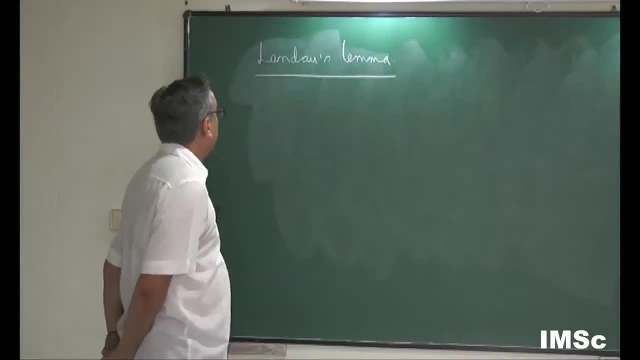 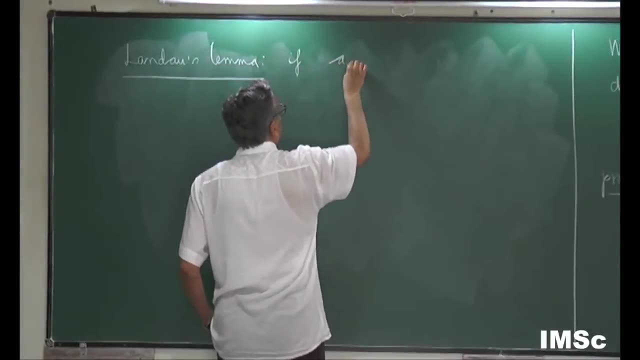 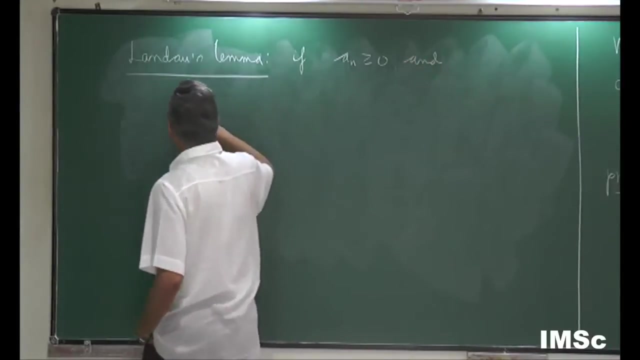 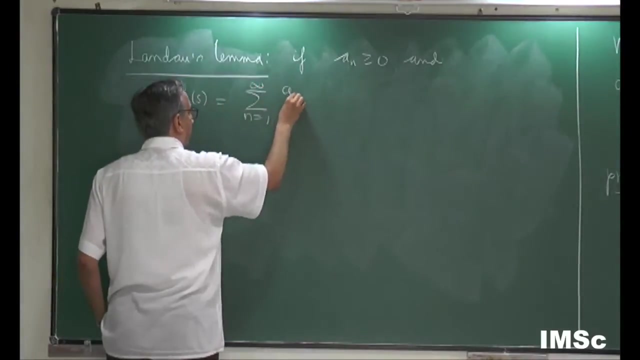 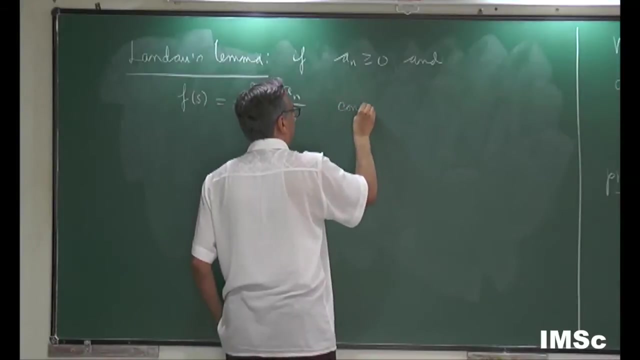 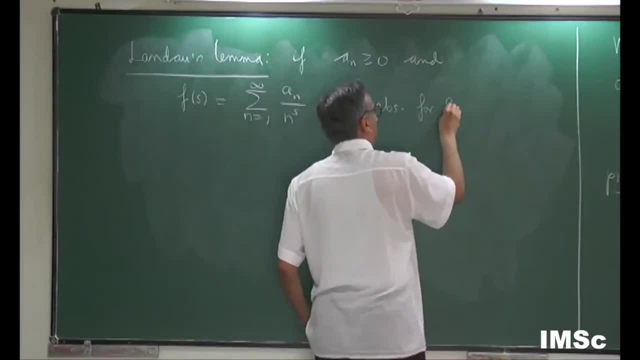 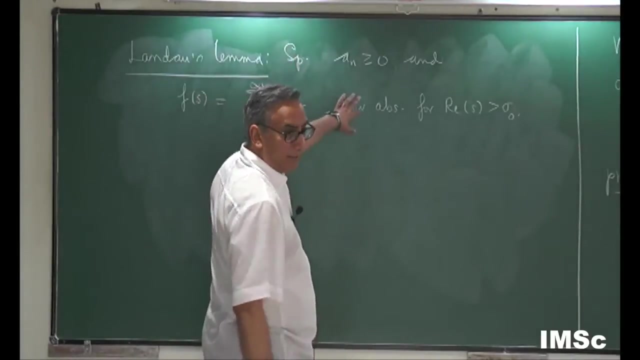 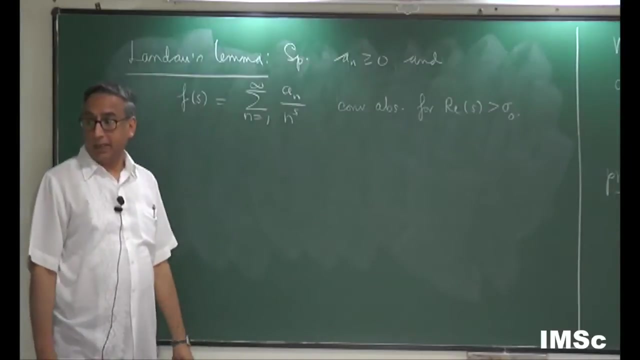 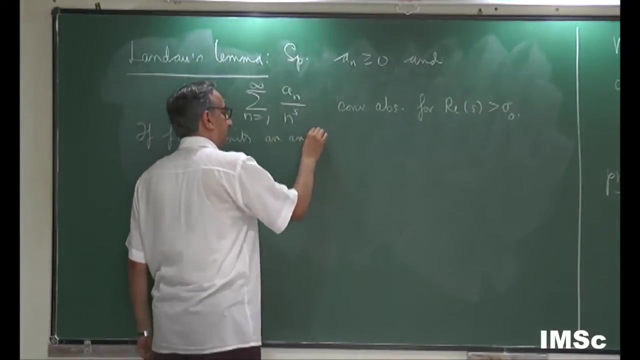 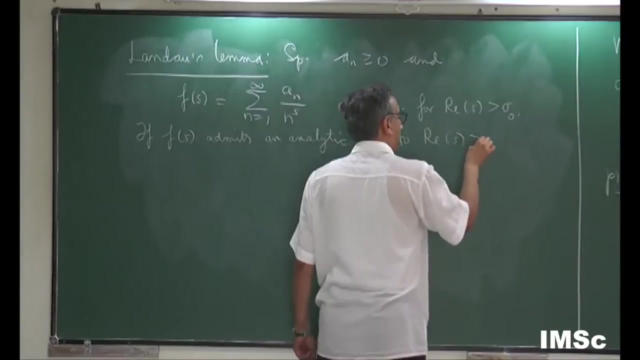 So maybe I shouldn't say if I should say: suppose, suppose that the A sub n's are non-negative numbers and that this Dirichlet series converges absolutely for real part S bigger than sigma, naught, Okay, Okay, Okay. So if F of S admits an analytic continuation to real part S bigger than or equal to sigma, 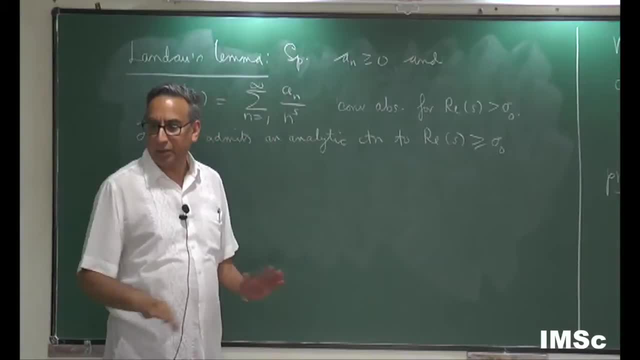 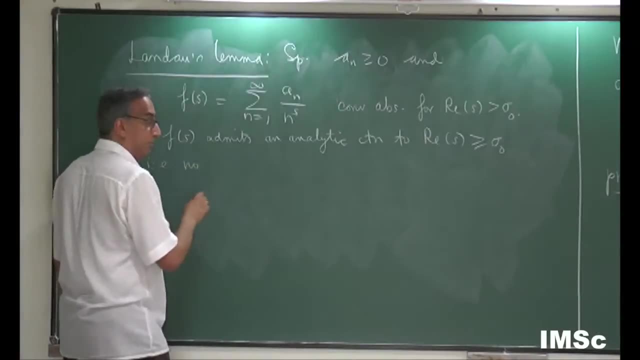 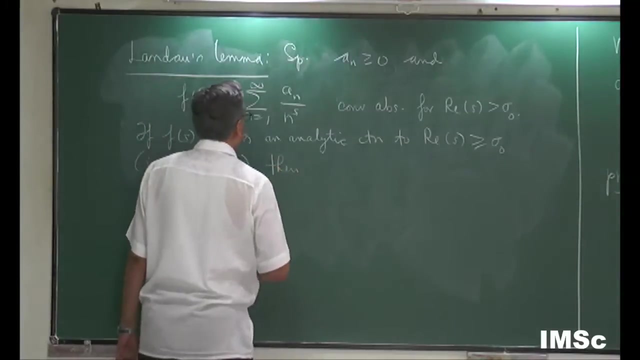 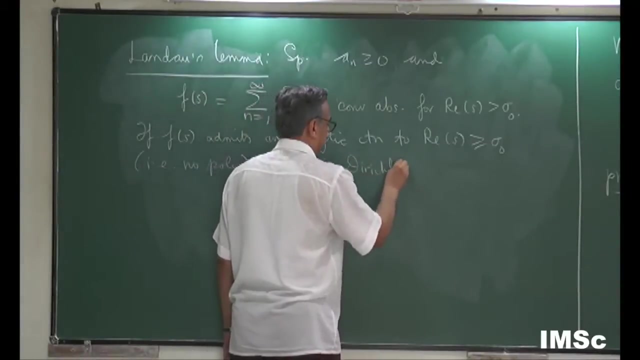 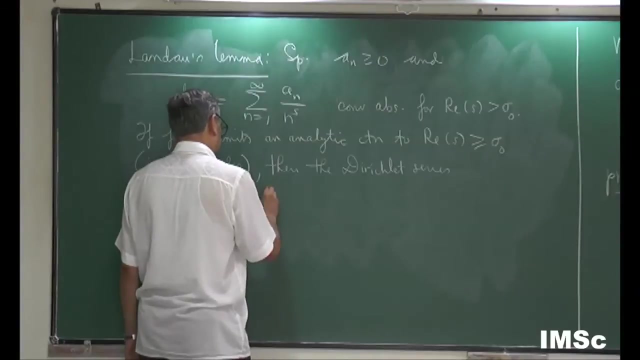 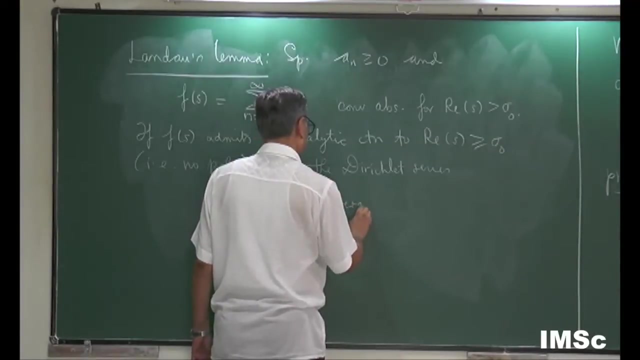 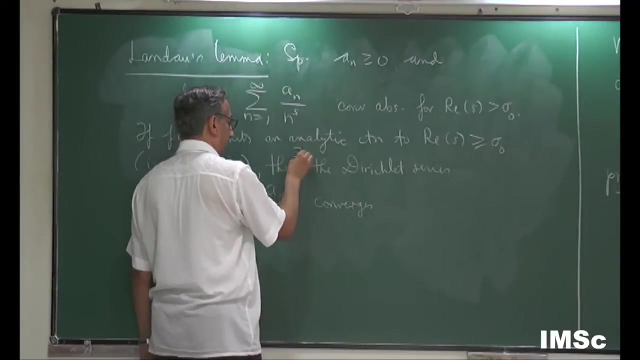 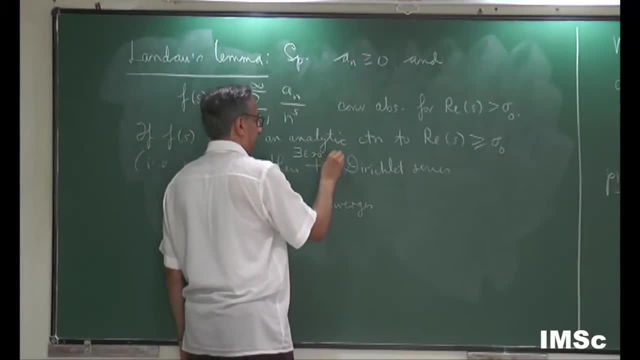 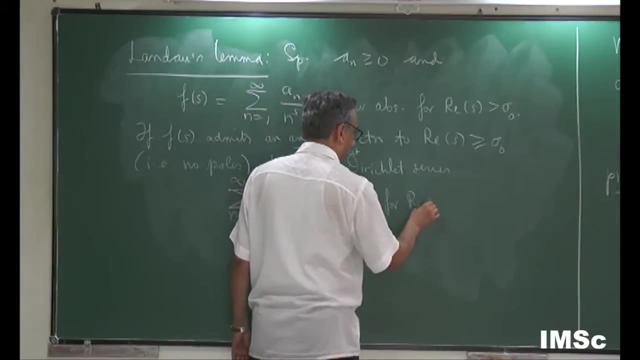 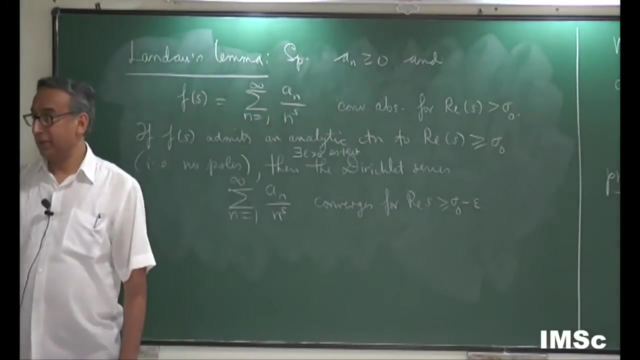 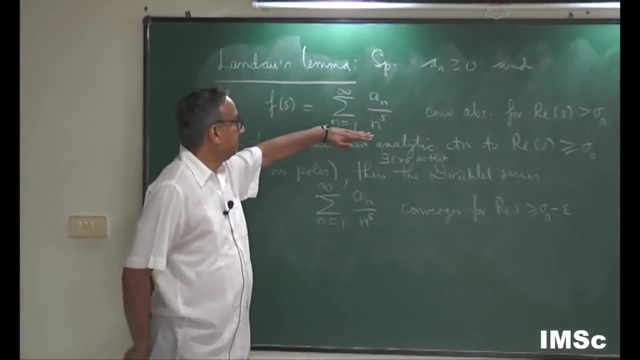 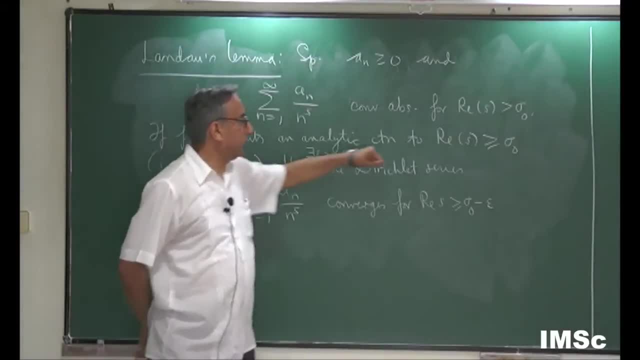 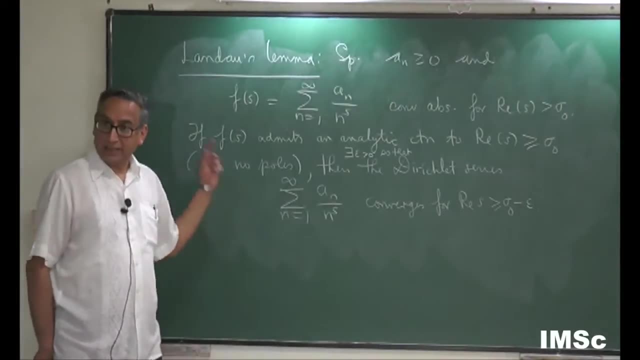 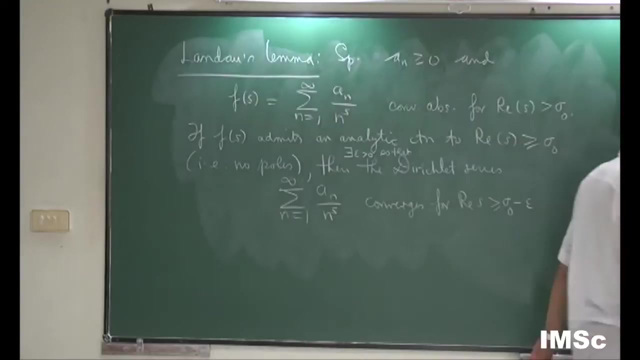 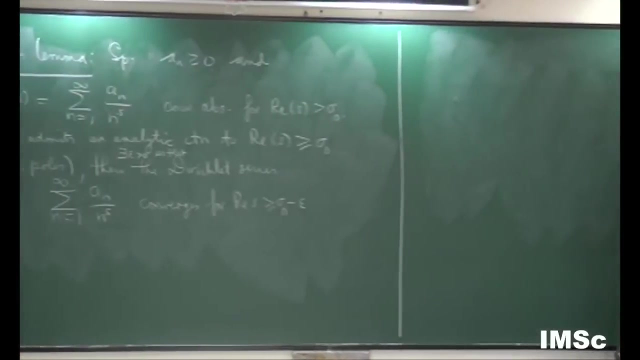 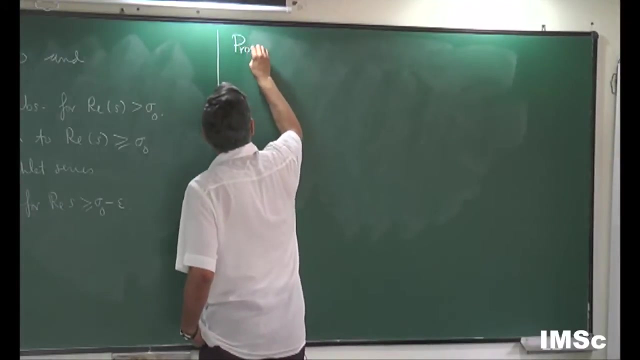 an analytic continuation to a larger region, then the Dirichlet series itself actually converges in this larger region and is that function? so it's kind of very interesting statement being made here. So let's see how you prove this. it's pure complex analysis. so prove well by shifting. 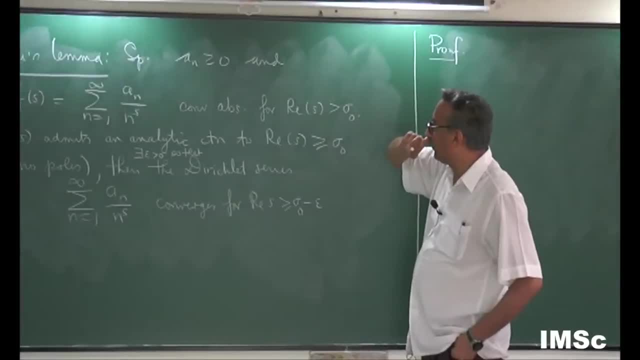 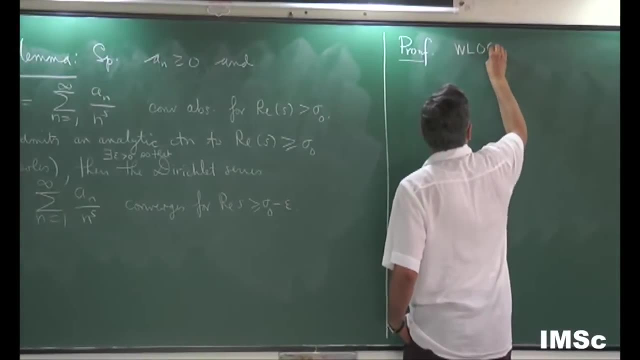 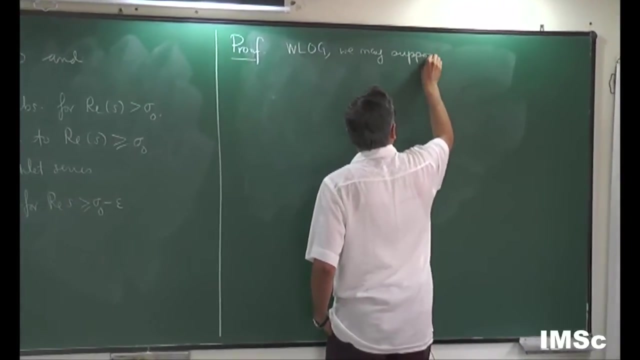 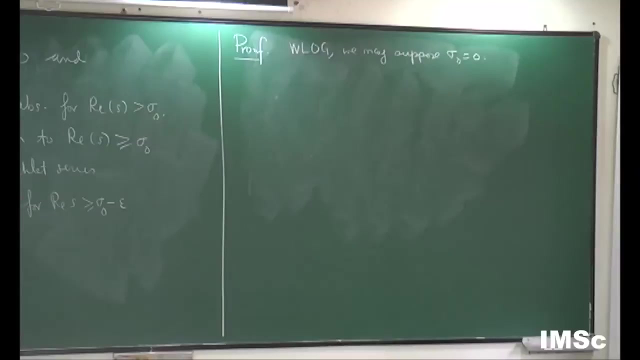 with. you know, we're shifting the redefining a sub n's. if necessary, we can assume sigma 0 is 0, so, without loss of generality, we may suppose sigma 0 equals 0, because you could just replace a n by a n over sigma 0, shift the whole business to that, okay. So, having done so, then the, the 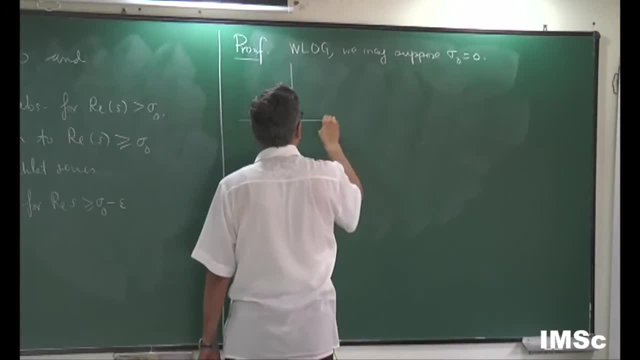 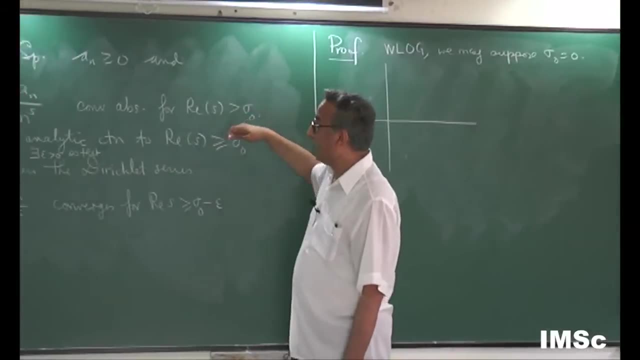 hypothesis of the state of the theorem tells me that the Dirichlet series converges from the Dirichlet series. converges from the Dirichlet series, converges from the Dirichlet series, converges for real part as bigger than 0, it has an analytic continuation to real part as equal to 0, and then 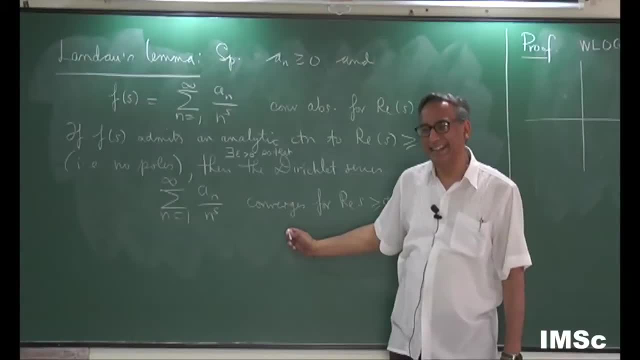 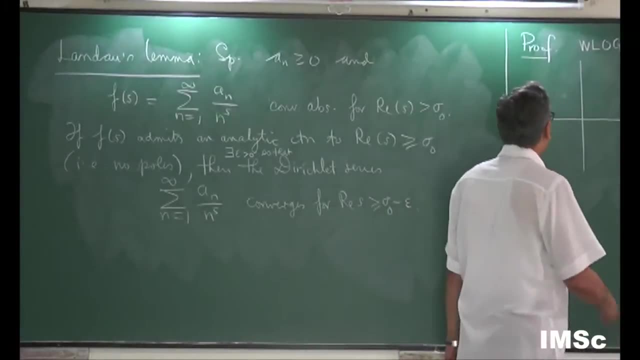 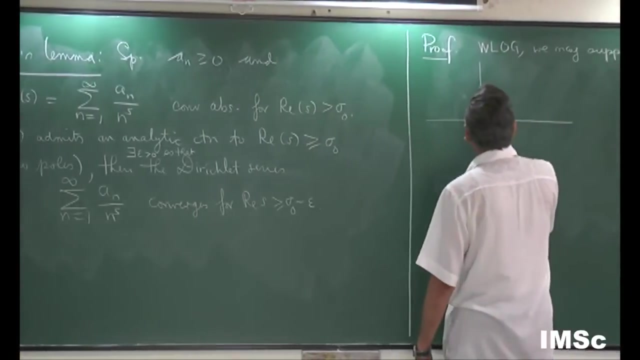 the Dirichlet series actually converges at 0, and even to the left. that's. that's basically what this is saying, and so let's see how that works. if the function admits an analytic continuation to 0, then there's some small difference between the Dirichlet series converges from the Dirichlet series converges. 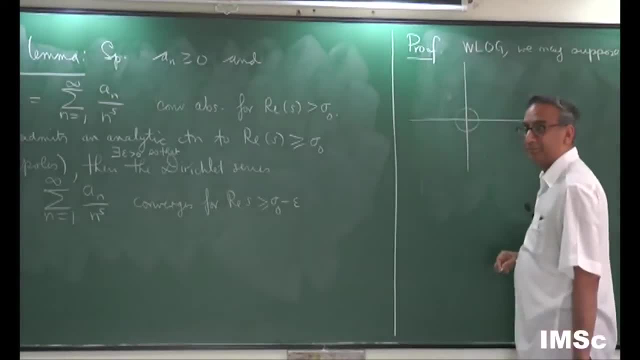 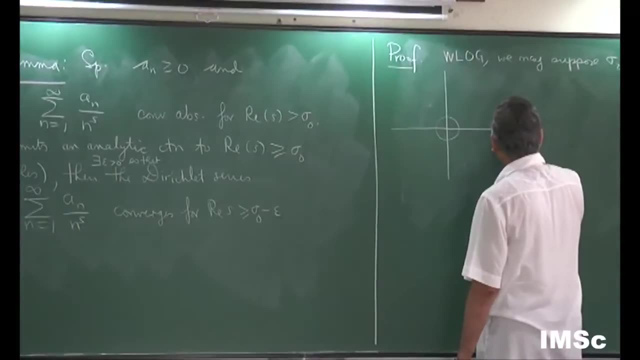 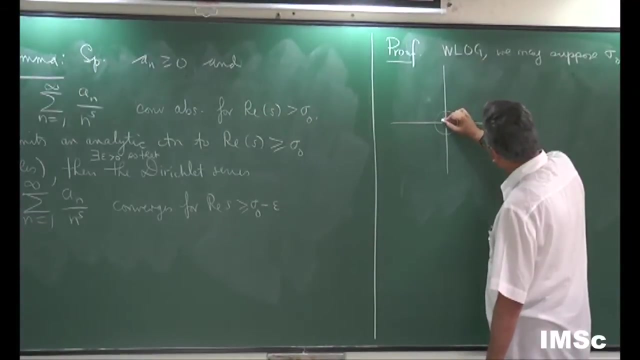 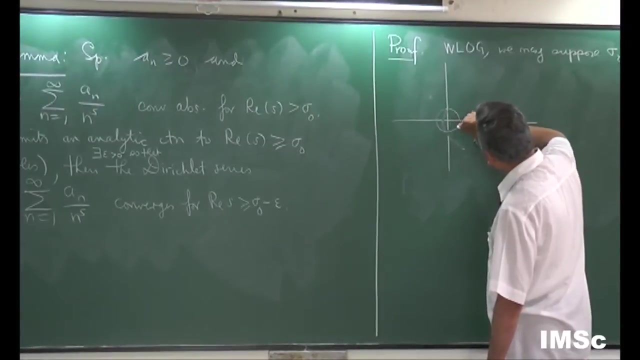 small neighborhood of 0 for which it's analytic in that region. so here's: s equals 1, let's just keep. and so that means I can draw some circle. oops, this is my bad at drawing, so. so here's the circle in which the thing is analytic. okay, so I'm going to draw the circle in. 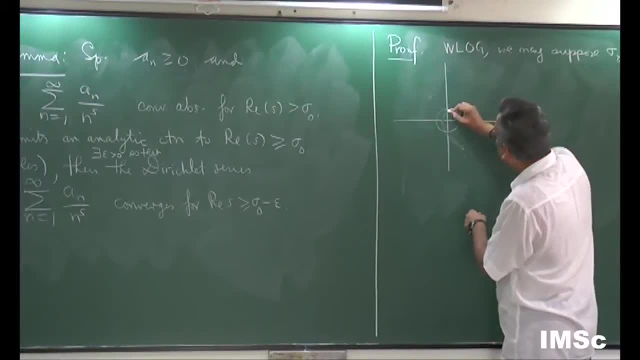 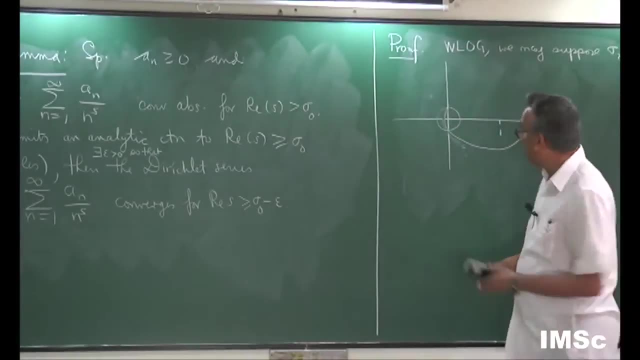 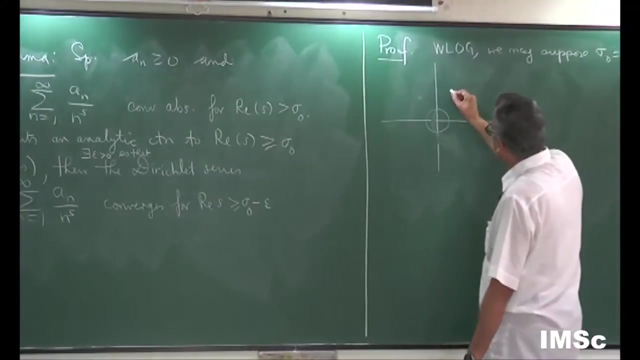 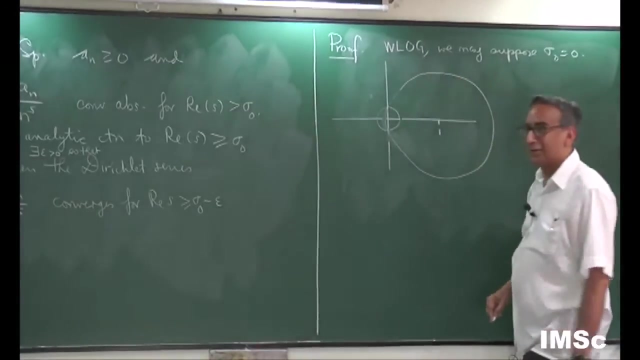 such a way centered at 1, in such a way that this- okay, this is not a circle, wait a minute. sorry, sad thing is that this is even being filmed, so. so let me draw a circle first. does that look like a circle? okay, good, that's looks reasonably like a circle. I want to have a circle centered at 1. 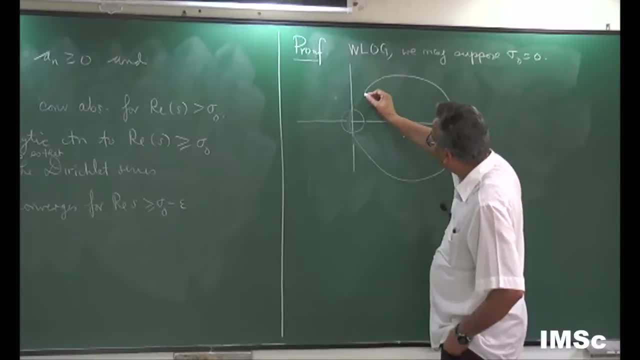 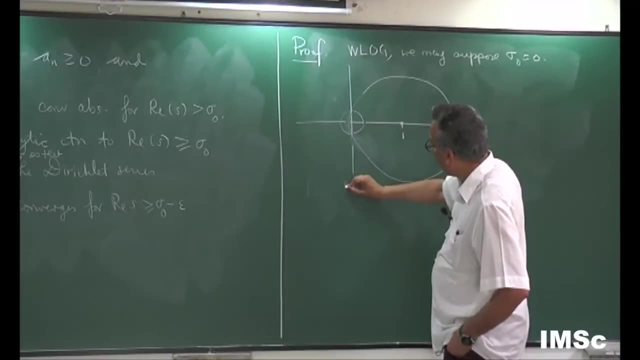 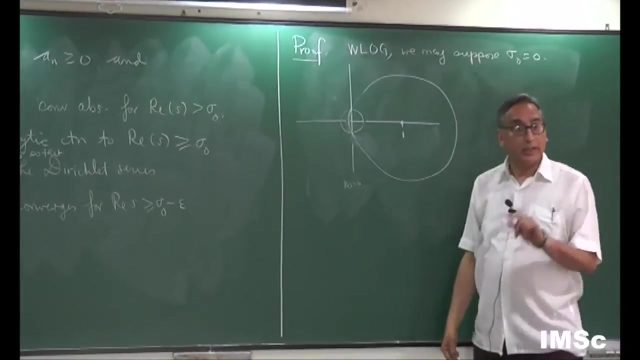 and I want the region that extends to the left of real part s equals 0. so this is real s equals 0, to be. that little bit that it extends to should be in that neighborhood in which the function is analytic. okay, so now I know that in this 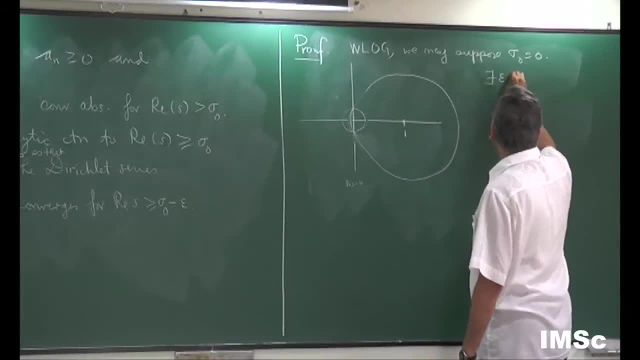 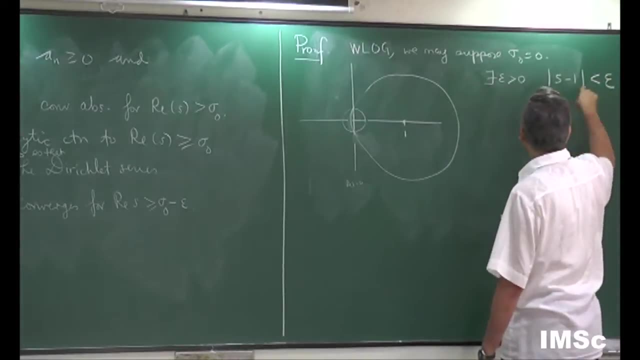 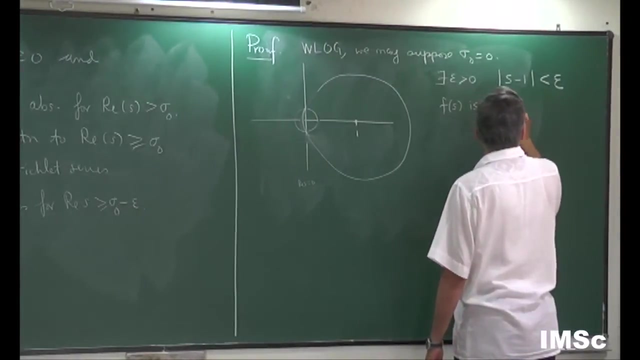 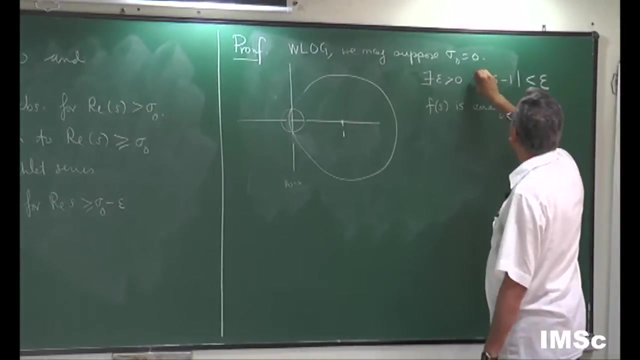 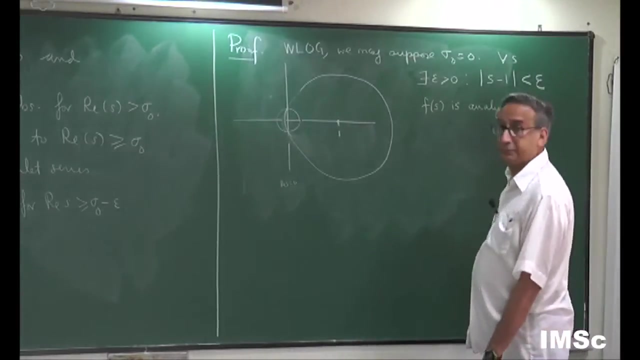 region there. firstly, there exists an epsilon positive. this is all I want to say. so it's that, such that for this region, f of s is analytic in this region. so there is just an epsilon positive, such that for all s in this, hmm, I want to put one plus epsilon, thank you. 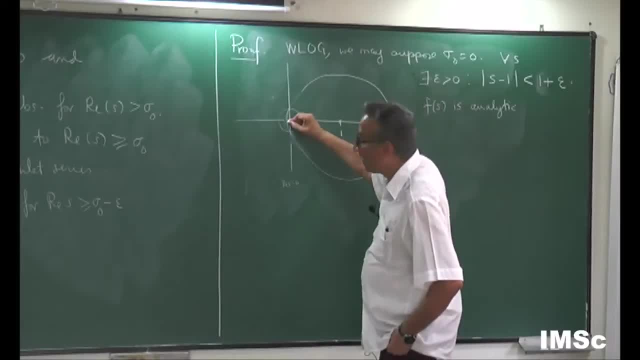 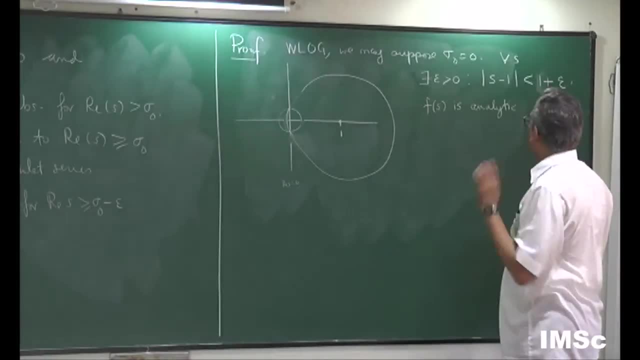 yeah. So yes, this little itsy bitsy bit here, epsilon should be small, so you don't want to make it bigger than one. this is part of mathematical theology, I guess. Anyway, ok, f of s is analytic in this region, and so it has a Laurent expansion. 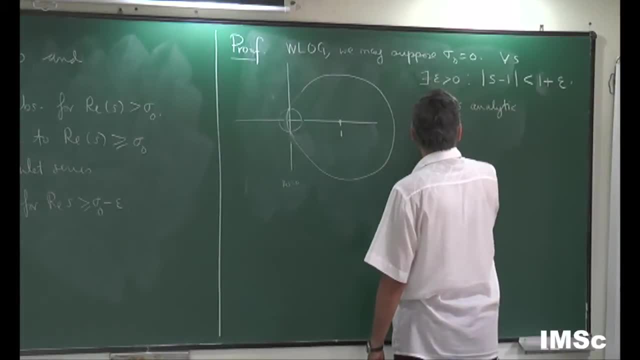 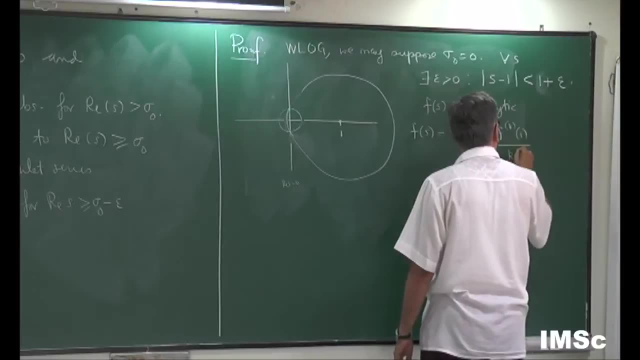 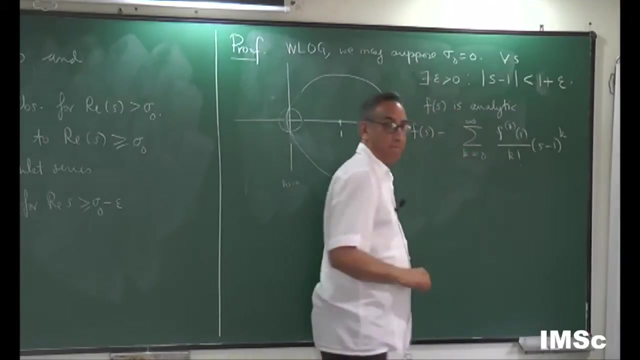 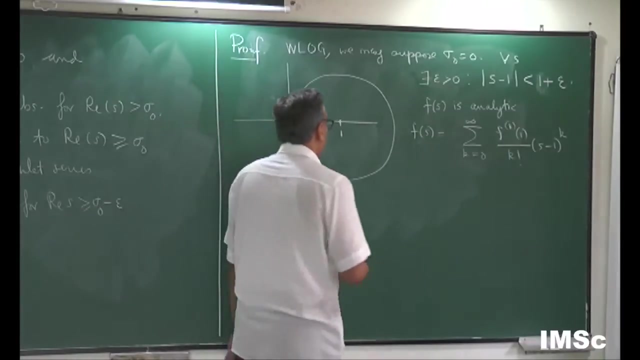 so it has a f of s. S can be expanded as a Laurent series about 1, Taylor series or, in complex analysis, will be called Laurent series. Now, what is Fk of n? So here now I am in the region of absolute convergence. remember the Dirichlet series? 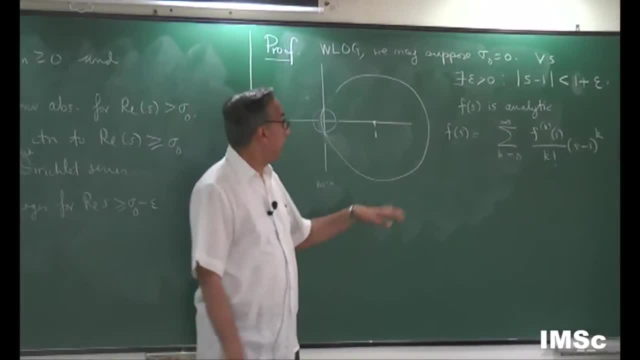 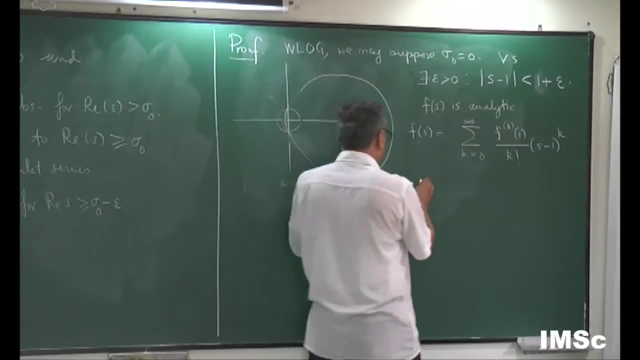 converges absolutely. for real part S bigger than 0. So 1 is certainly in a reasonably good region. the Dirichlet series converges absolutely and so you have F of S in that region, given by An over N to the S right. 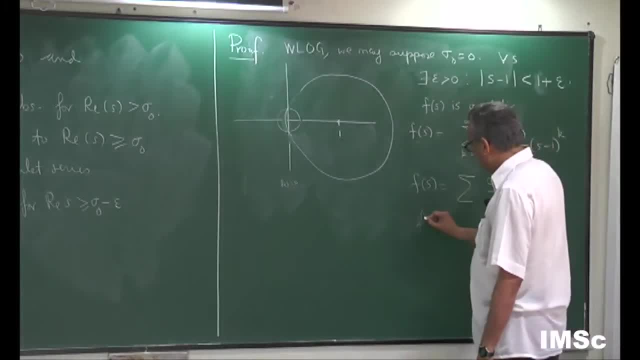 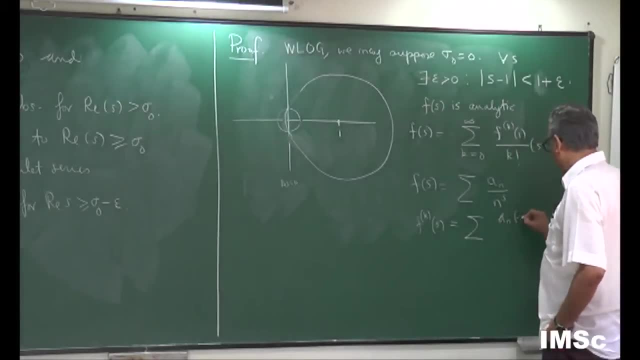 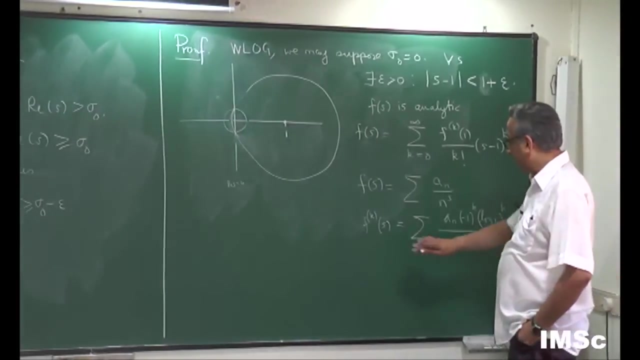 That is the Dirichlet series. And so if I want to differentiate umpteen times, I differentiate it umpteen times and get right. And so if I was to put S equals 1, now, which I can, this is an absolute convergence series. 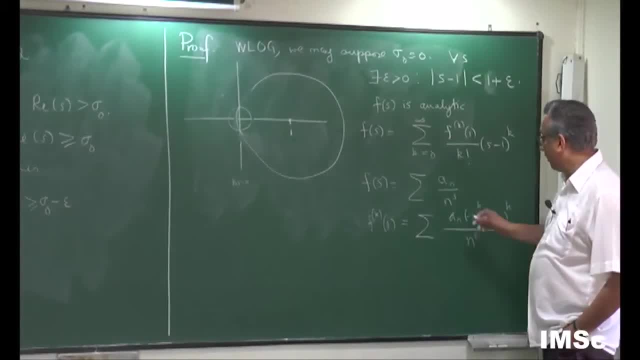 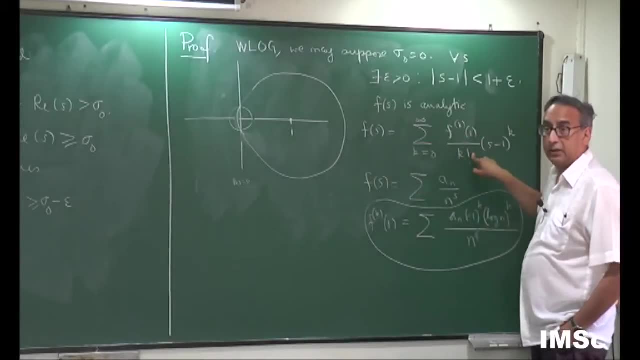 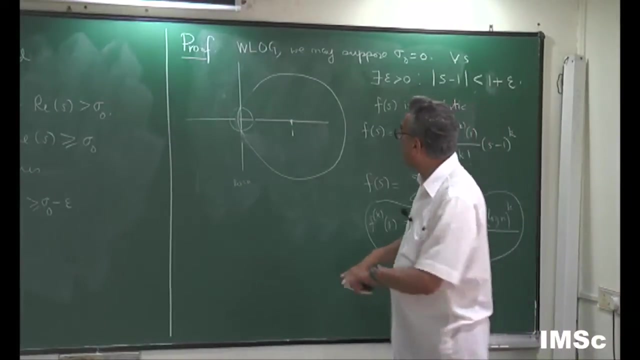 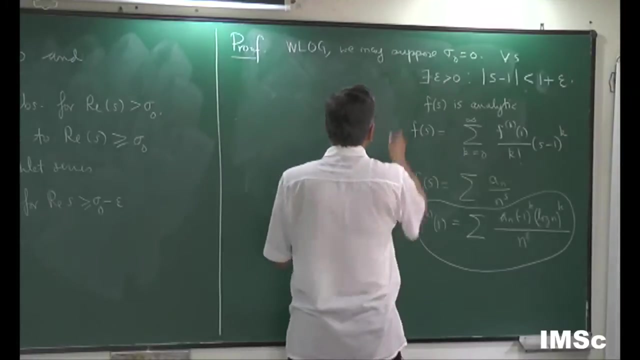 right. So you get that, and so I am going to use this expression and shove it, this Laurent expansion right. It converges absolutely in this disk. okay, region of analyticity. So let me now rub this bad picture off. continue here. 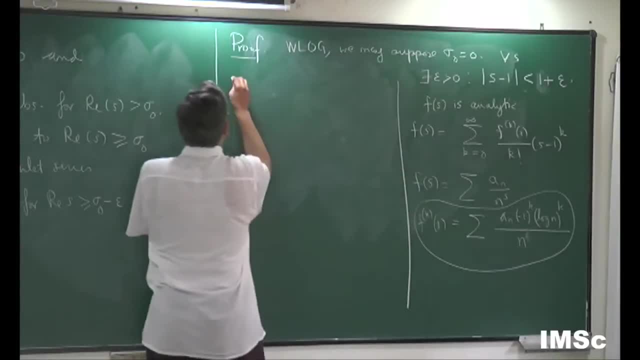 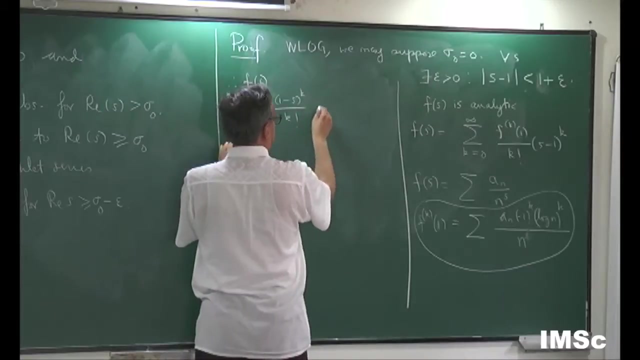 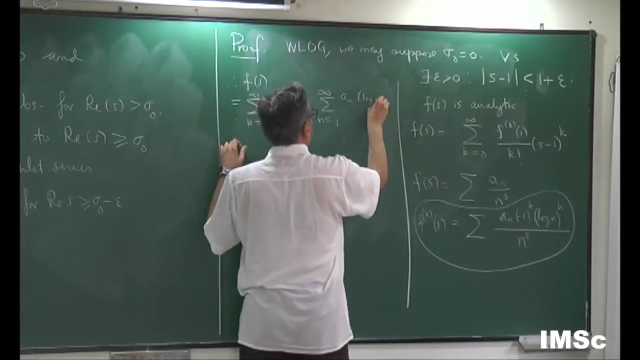 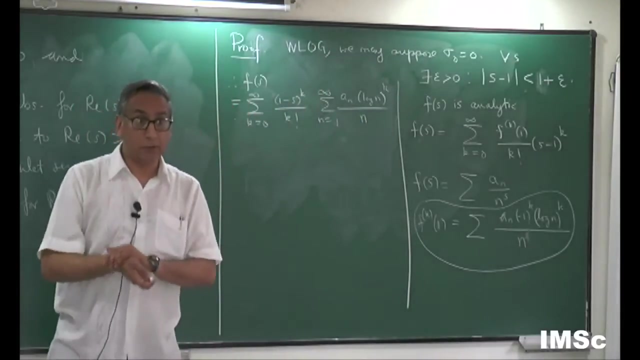 So now plug this back in here. everything is now convergent, absolutely So, the minus 1 to the k. I am going to put 1 minus s to the k. Everything is convergent, absolutely okay. That's why I am. 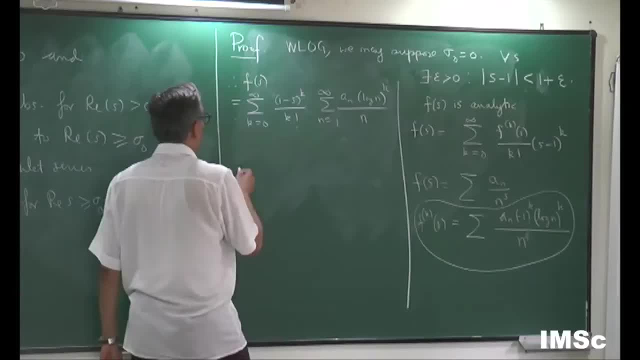 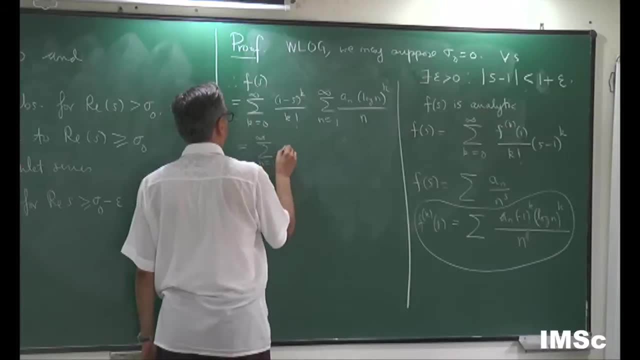 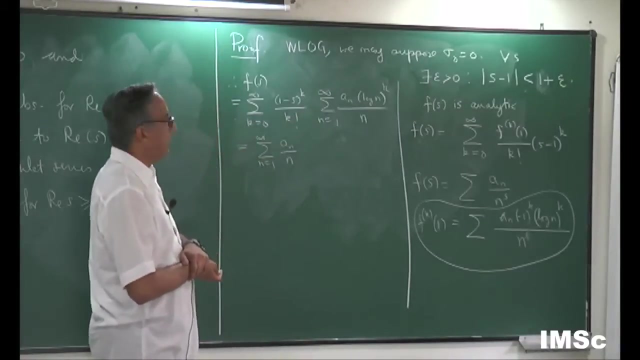 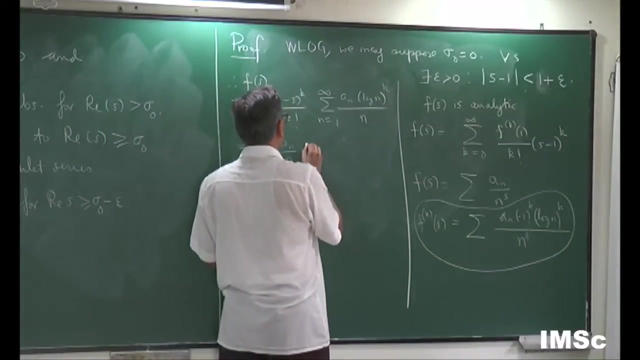 I have moved to 1, safe place. And now so I interchange summation And recognize that the inside sum is the sequence for e to the power 1 minus s, log n, which is basically n to the power 1 minus s. 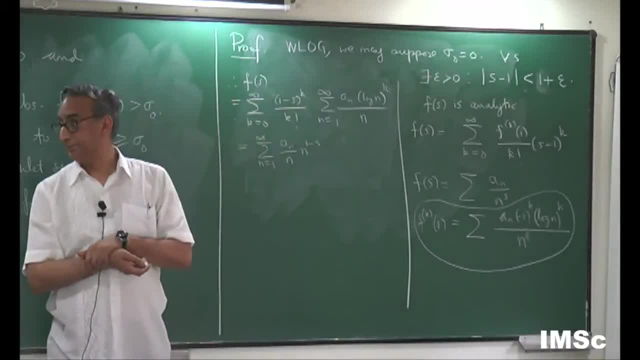 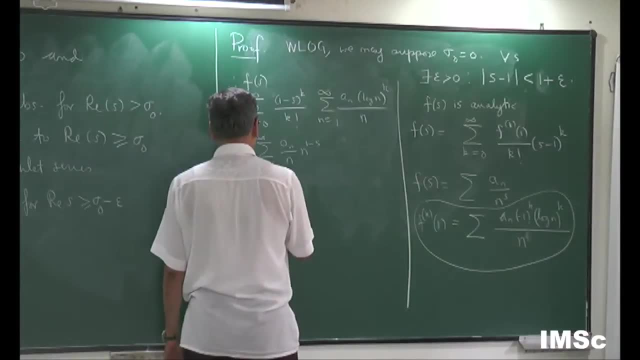 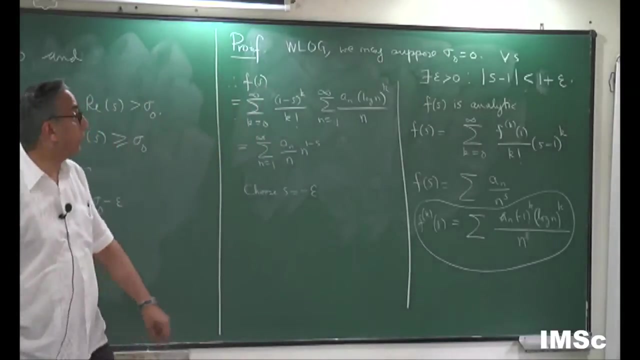 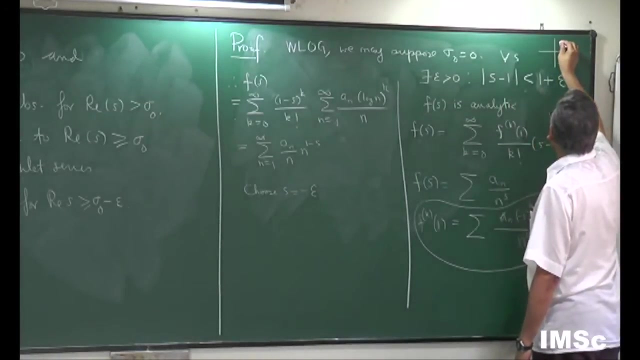 This is all good. This is all valid in that region. So now choose s equal to minus epsilon, which you can do, because I took away that picture, but remember that picture was something. maybe this is the way I should have drawn it first. 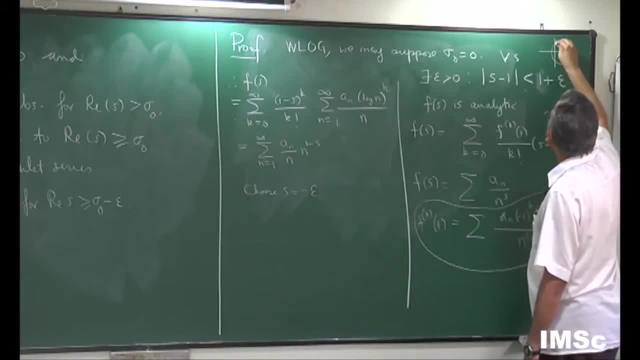 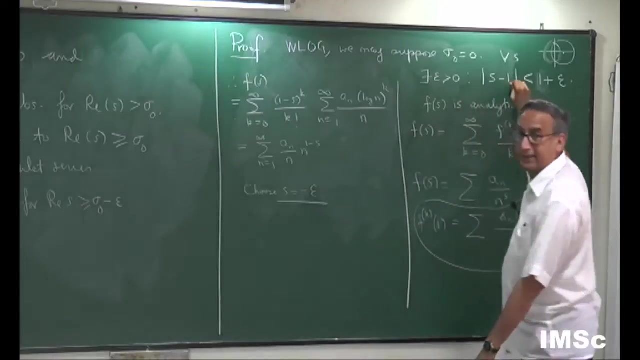 Okay, And then Okay, And then made a little thing like that, But anyway, okay. So this, there is a little bit of an epsilon that goes out there, So I choose that which I am valid, which is valid because I am still sitting inside. 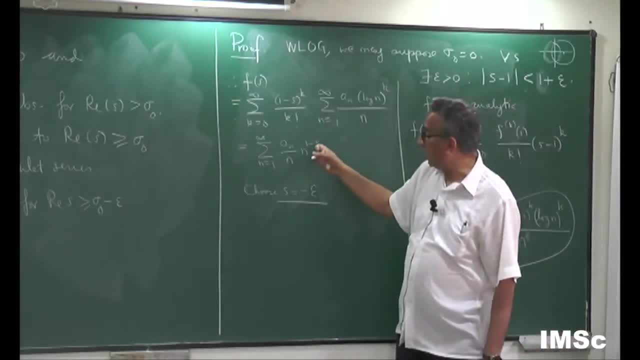 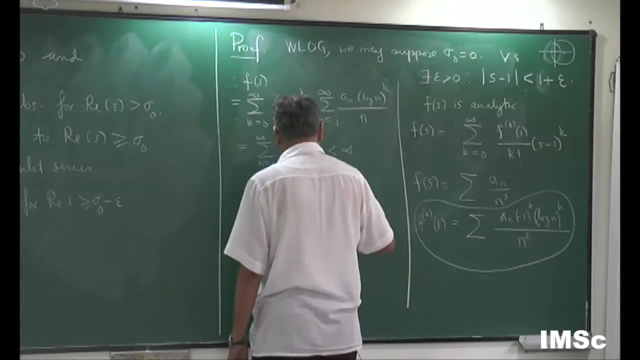 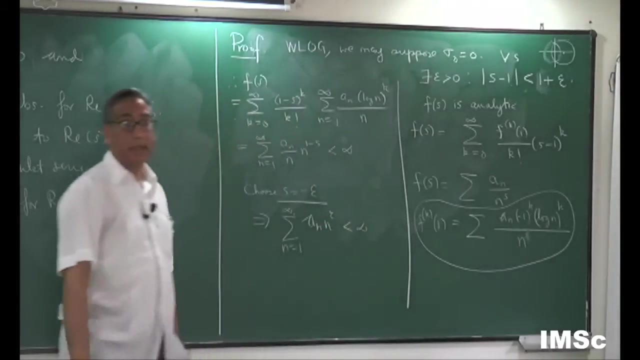 this region. When I do that, you can see that it becomes 1 to 1 plus epsilon And therefore this actually still converges and therefore you get an n to the epsilon converges, Which is Okay. The Dirichlet series at minus epsilon. 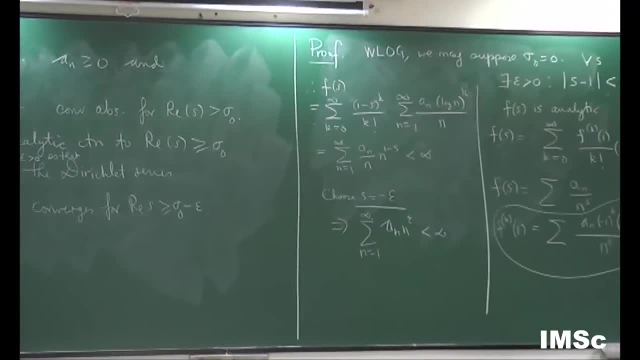 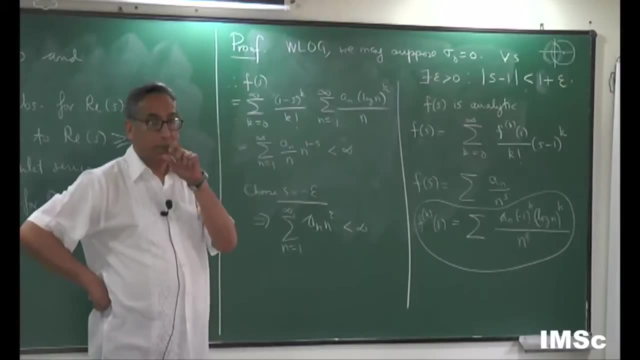 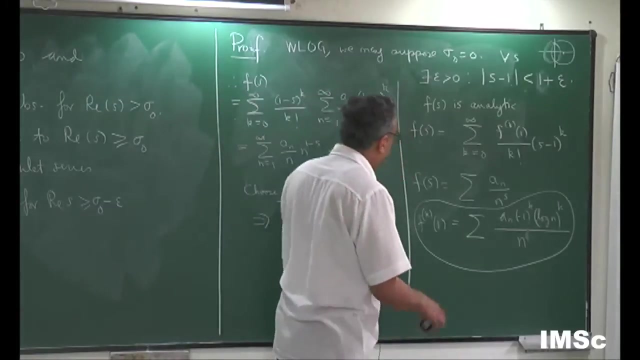 That is the proof. Okay, That is the proof of Landau's theorem. So it is a very interesting theorem. It is a theorem in complex analysis and relatively easy to understand If you have some basic intro to that. Okay, So the region of analyticity: 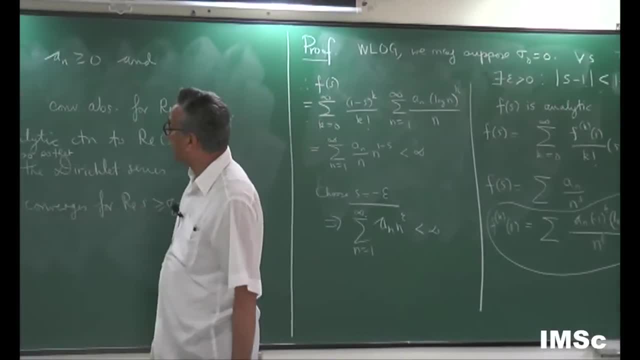 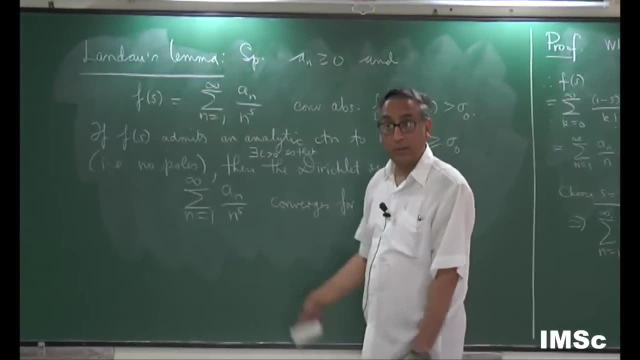 So there is this very powerful tool- Actually This thing is- And now we are going to use it to show non-vanishing. Everybody okay with that? All right, Okay, So I am going to rub this off If everybody has finished copying. 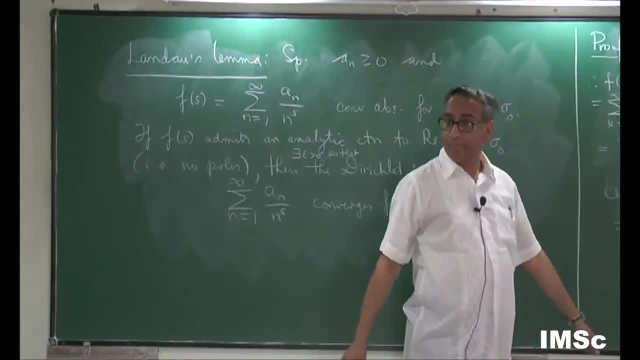 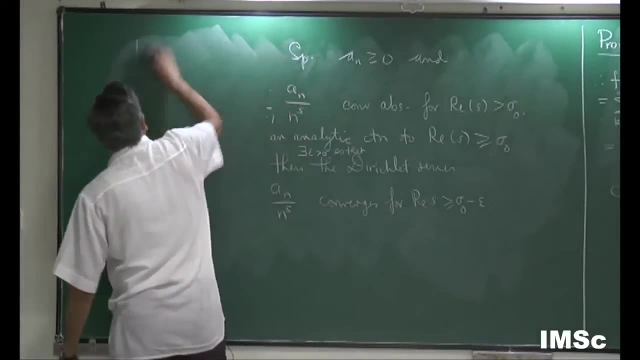 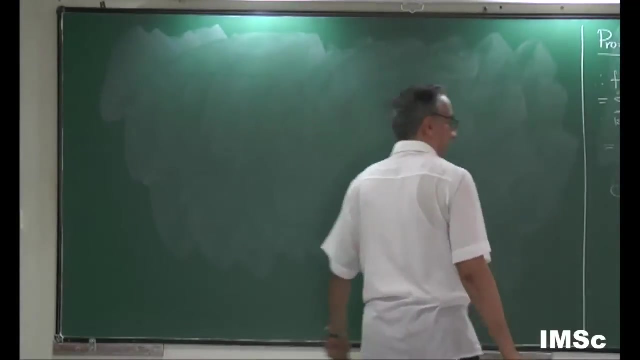 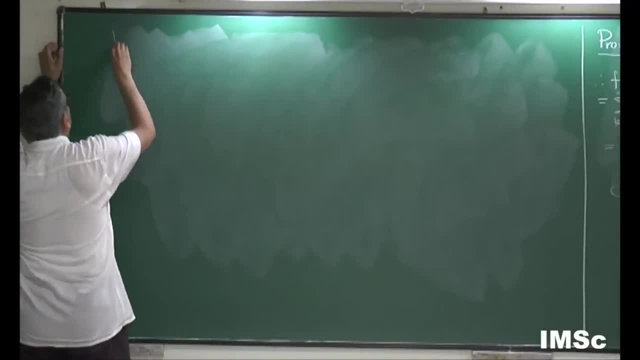 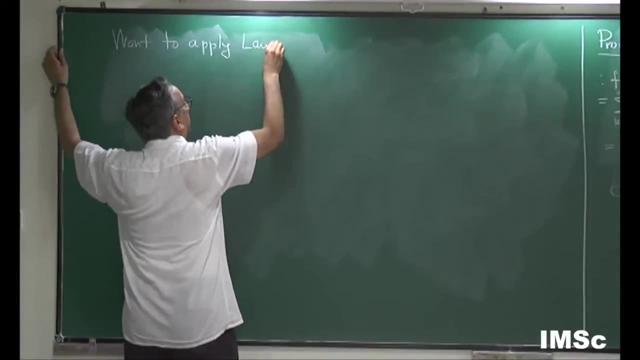 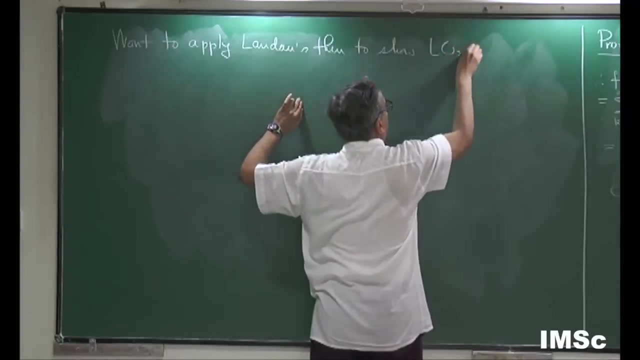 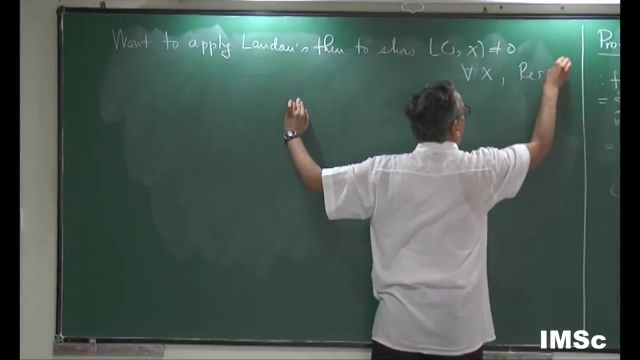 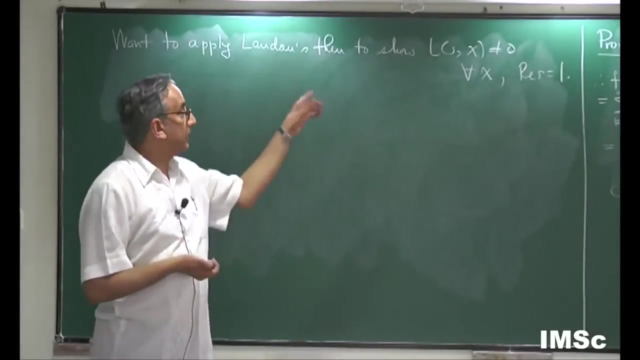 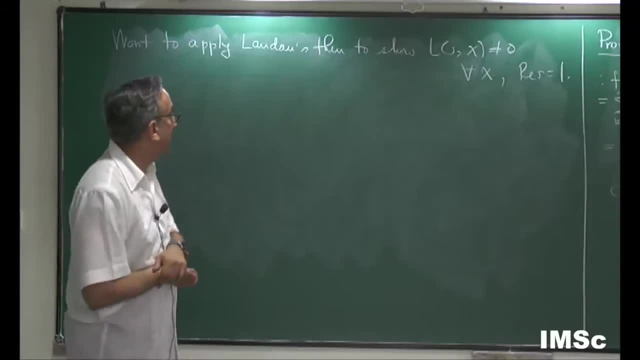 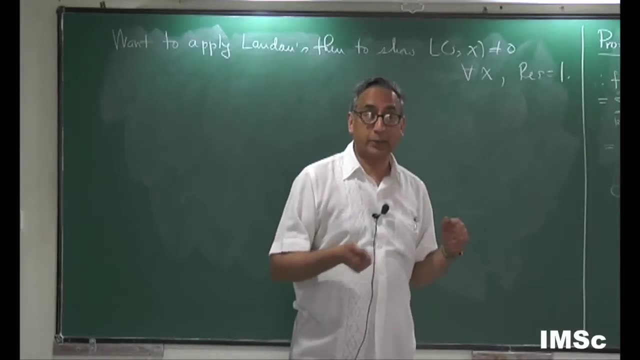 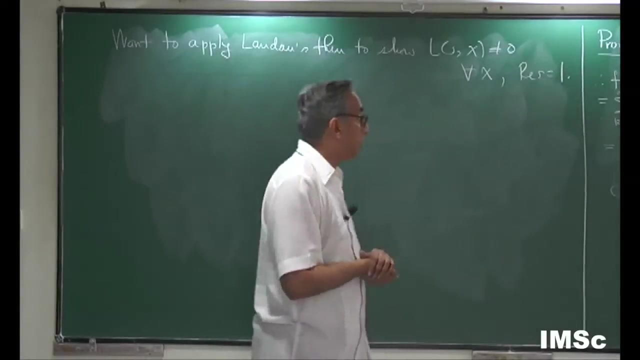 identity 3 plus 4 cos theta plus cos 2 theta non-negative right. And you might think at first hand that how come we cannot use that trick again for this situation. and actually you can, you can, you will see that, you can do that, you can get. 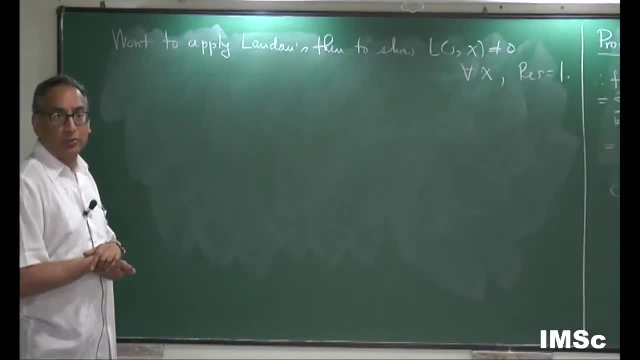 away with it, except there is going to be one point where you cannot use that trick, And so at that point I have to use lambda. okay, so let us see how that works. So we want to prove the non-vanishing, so here is how you kind of do it. 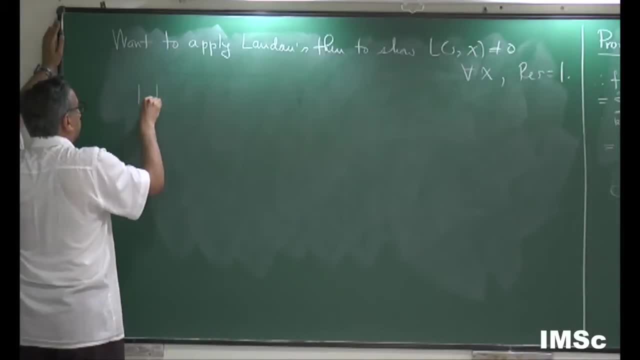 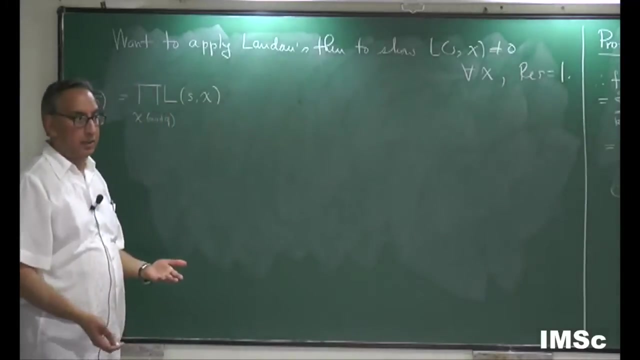 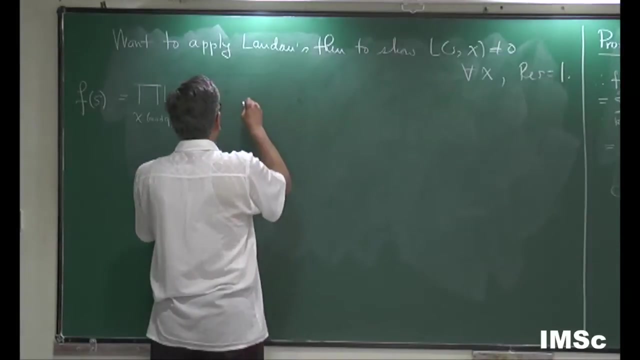 So you kind of consider product Ls chi, So let us call this guy f of s, Okay, And remember, each of these Ls chi is another Euler product And so if you think about it, let us see the easiest way to do. this is probably okay. 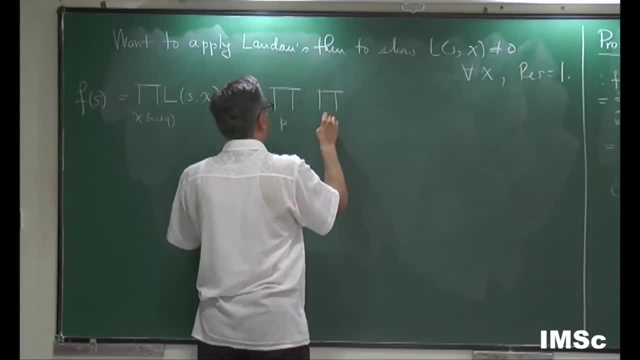 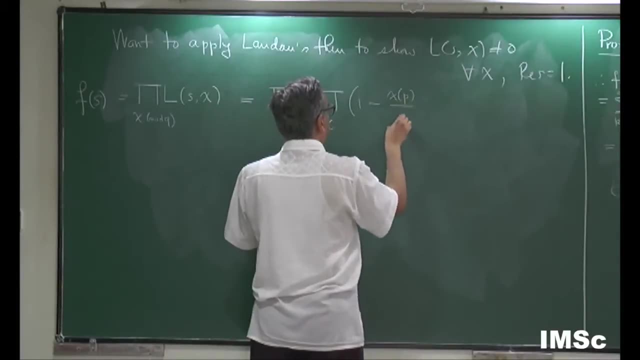 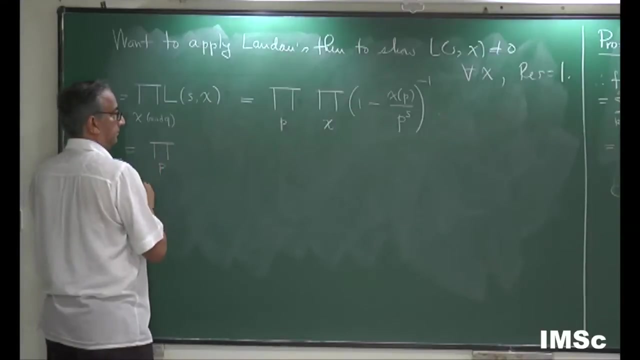 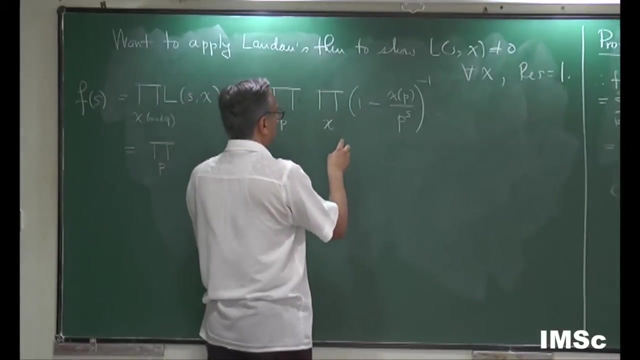 okay, I have an Euler product and I do that right Now. this guy, the inside guy, I can write it as So I have. So this guy is a body Right, So So. So if I write, I mean I can rewrite this guy here as exponential summation: chi minus log. 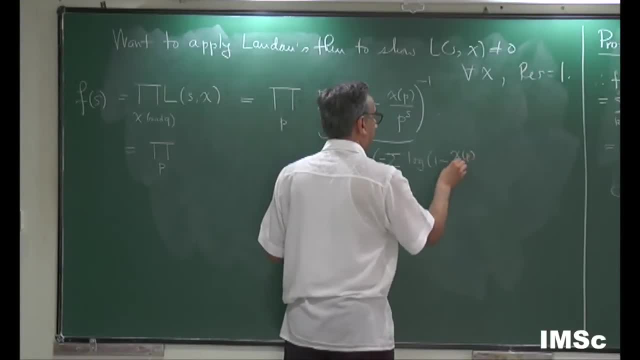 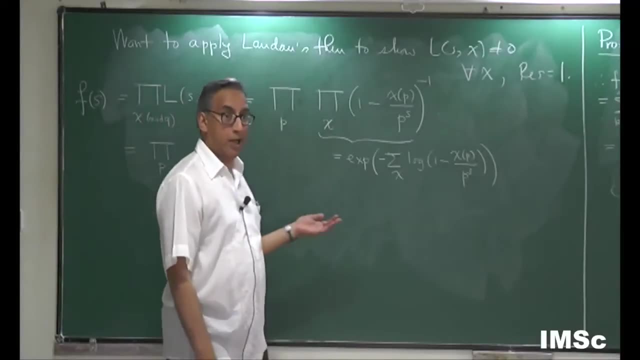 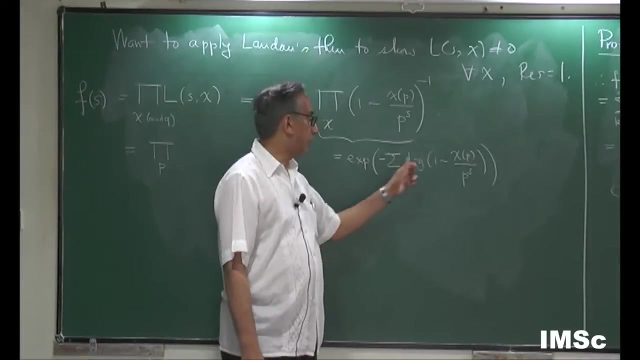 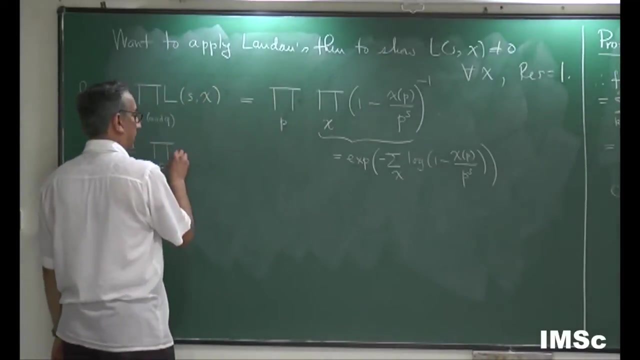 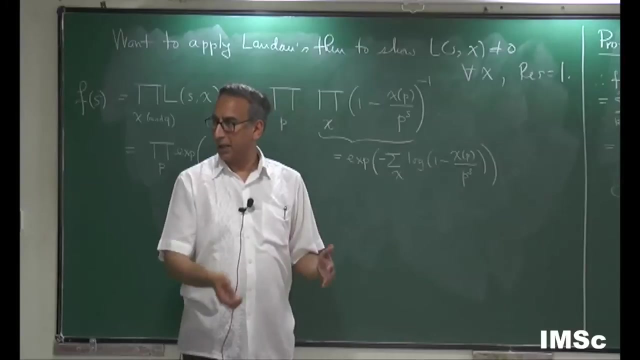 1 minus chi of p over p of the S. You may wonder why, but you'll see in a second. I can write this product as this thing. Exponential of log is the inverse function, so you can do that. And now that allows me to write this as exponential. so remember: minus log of 1 minus x is summation. 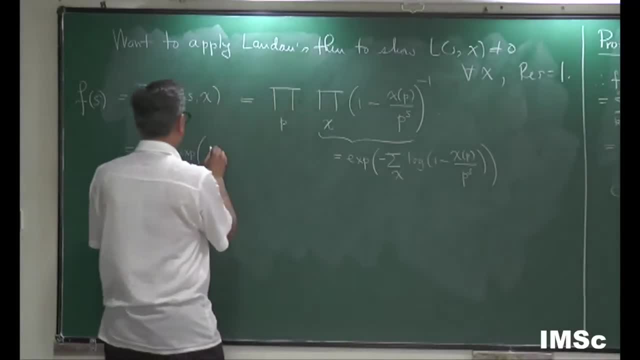 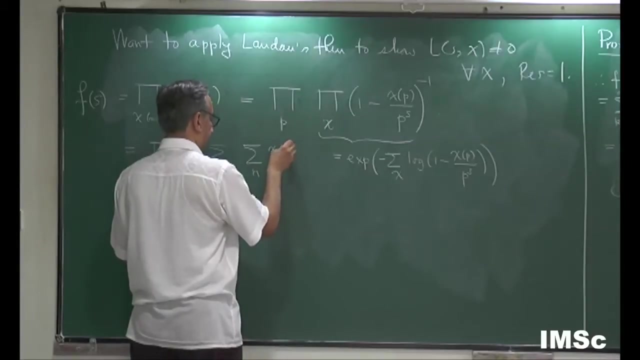 x to the n over n, the usual expansion. So this is an expansion over all n. So firstly it's an expansion, Firstly it's an expansion Over chi and then over n, chi of p to the n. Now, remember, it's a completely multiplicative function, so let's put it in here. 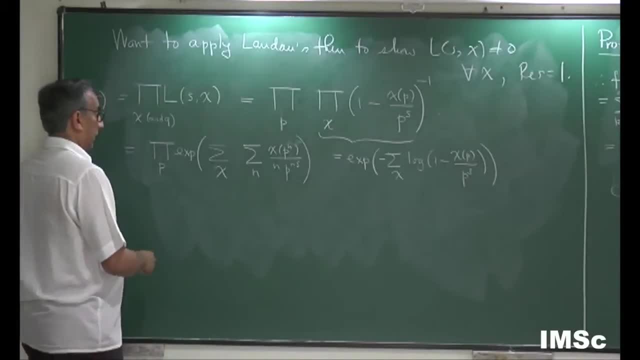 Everybody. okay with that? Okay, now you know. remember the orthogonality relation: summation: chi chi of a Is equal to phi of q if a is congruent to 1 mod q and 0, otherwise right. 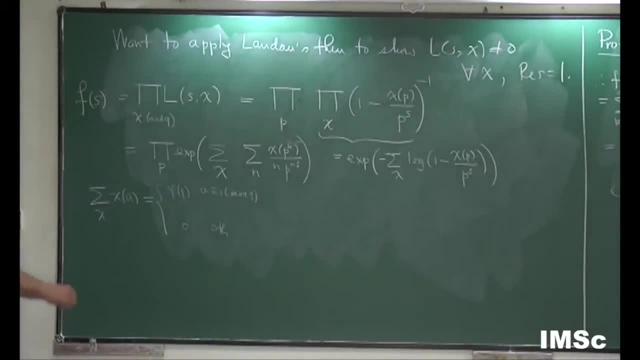 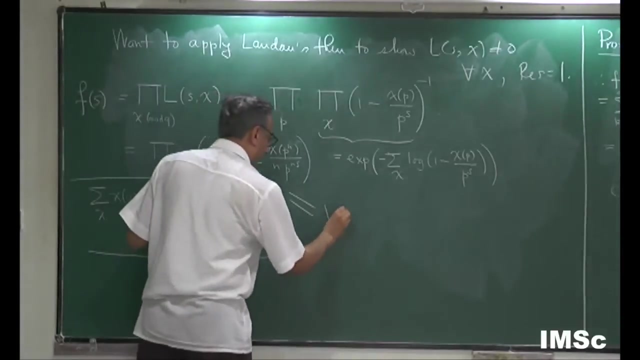 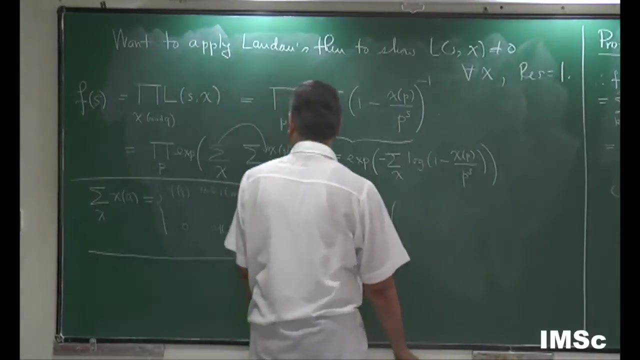 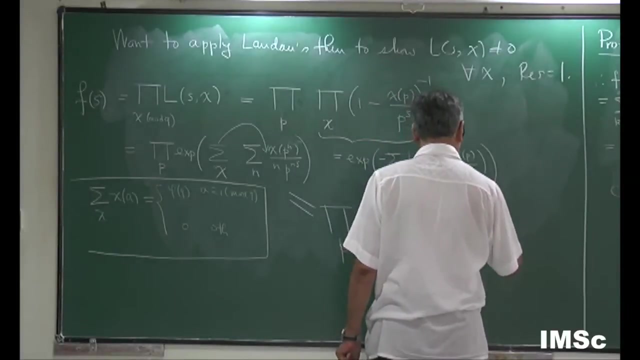 Got this orthogonality relation. So therefore, if I shove this summation here, this whole product here turns out to be: product over primes: p. Exponential of phi of q. summation 1 over n, p to the n, s, p to the n, congruent to: 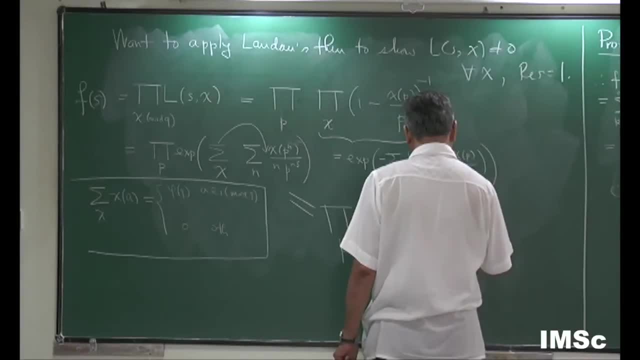 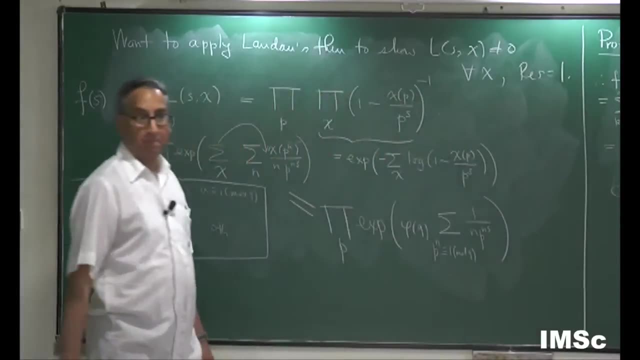 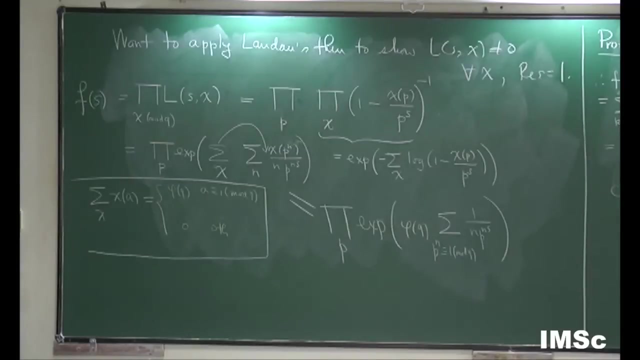 1, mod q. Everybody okay with this? Okay, Now what's the advantage? What's the advantage of doing this? The advantage is this is a Dirichlet series, now with non-negative coefficients. The problem with the characters was they could take on roots of unity. 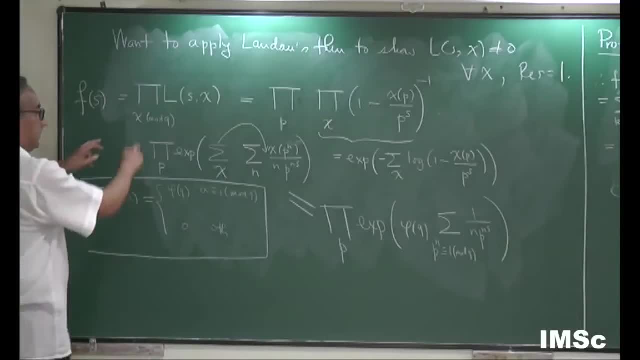 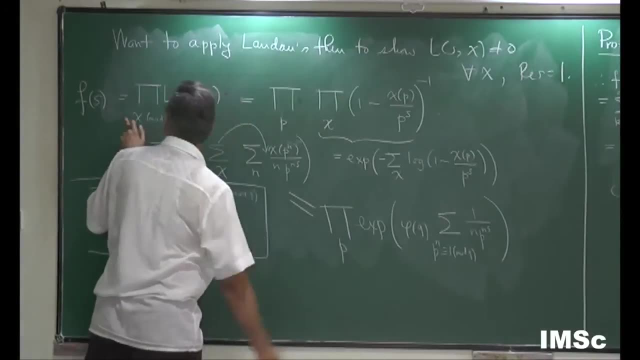 it could go all over the place, but considering this neat combination allowed me to make a Dirichlet series with non-negative coefficients. Therefore, f of s has got to be a Dirichlet series with non-negative coefficients. It's just a product of the whole thing, right? 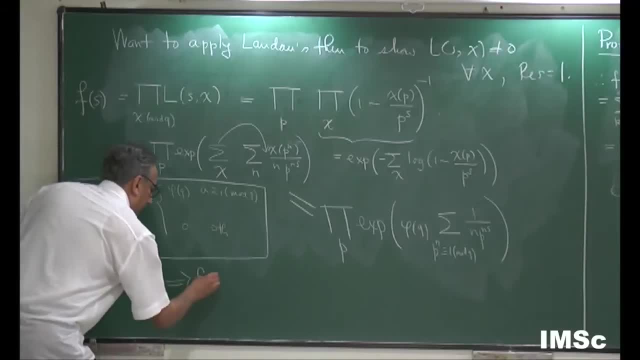 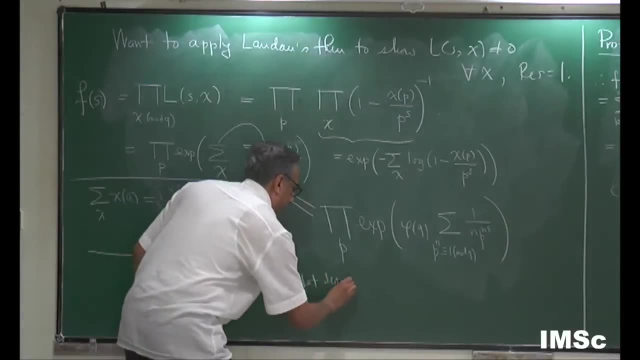 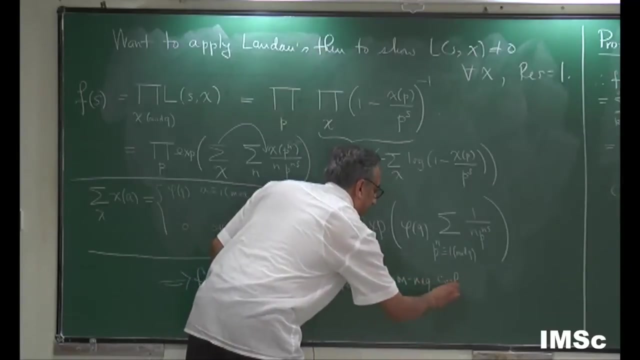 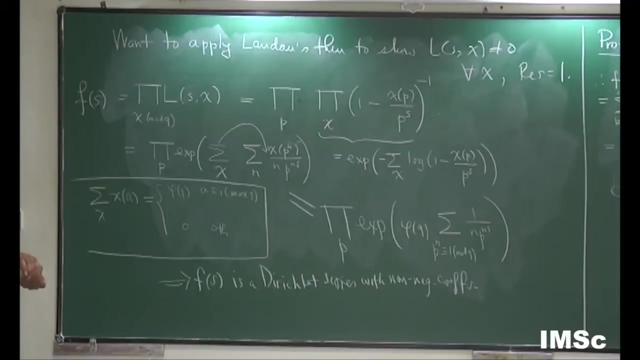 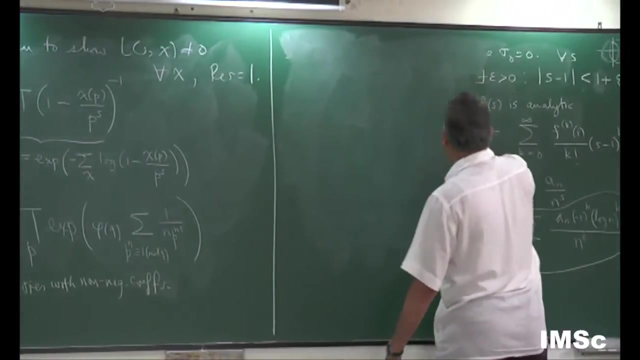 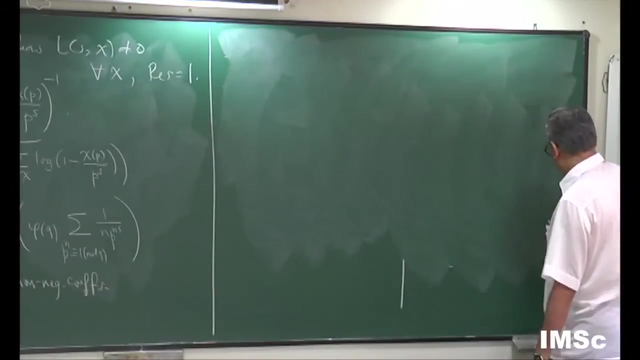 This implies that f of s is a Dirichlet series with non-negative coefficients. Okay, So, in other words- and now this is probably a good thing to understand with respect to the role of abstraction, I mean the idea of that three plus four cos theta. 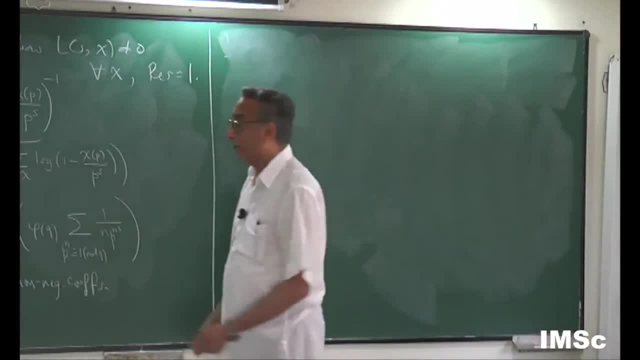 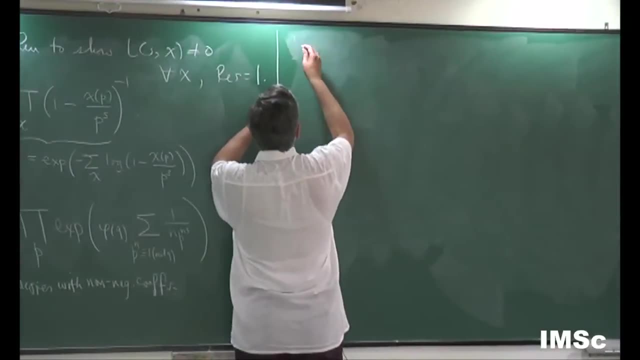 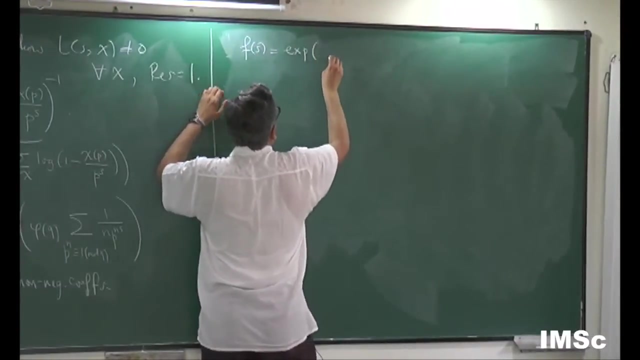 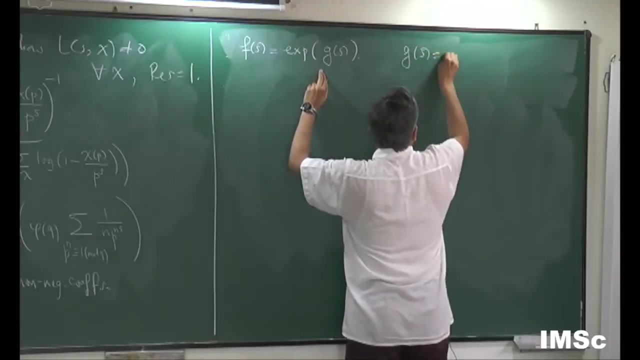 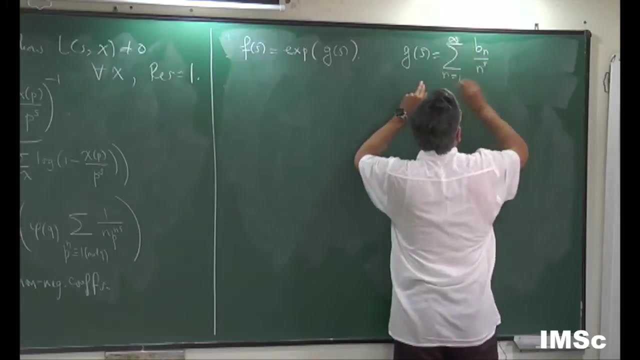 plus cos two theta non-negative trick really has nothing to do with the Riemann's function at all. So we're basically writing. so we have a situation where we are writing f of s as exponential g of s, where g of s is a Dirichlet series: b sub n over n to the s with b sub n's. 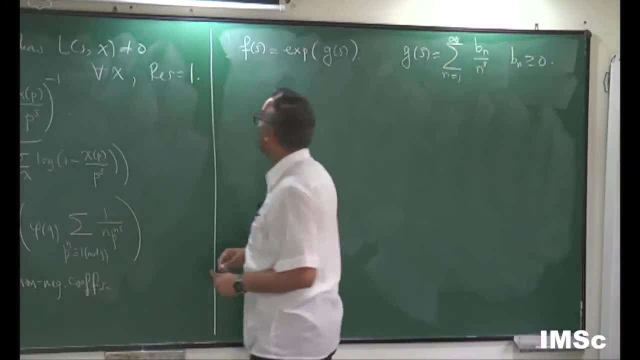 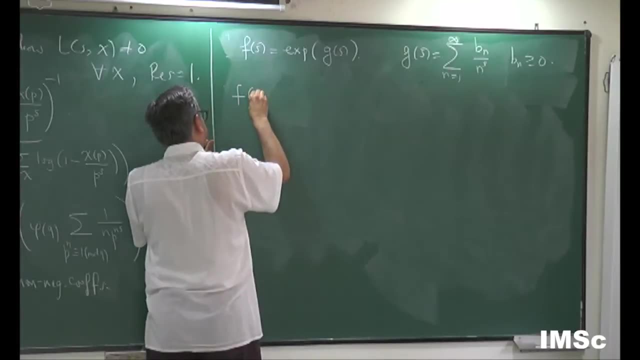 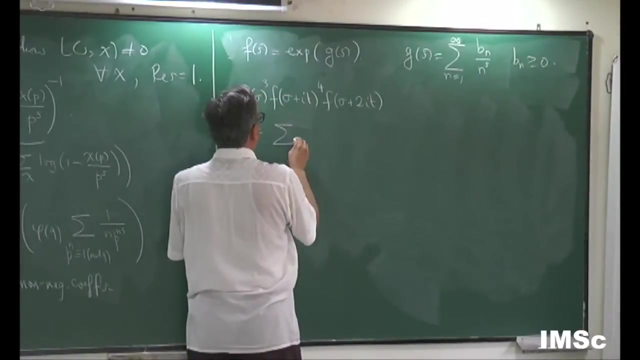 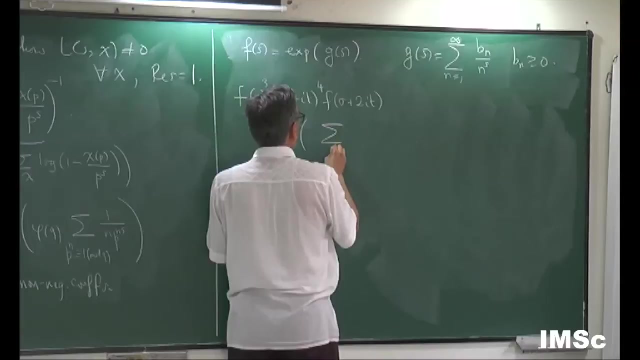 non-negative right. I mean, we have such a situation like this. Therefore, like the, the, if I, if I look at this combination, this combination, I write this as summation. I'm sorry I write this as exponential of. well, it'll just be bn over n to the sigma. 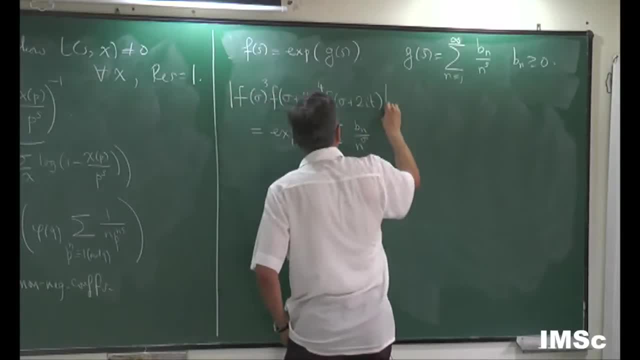 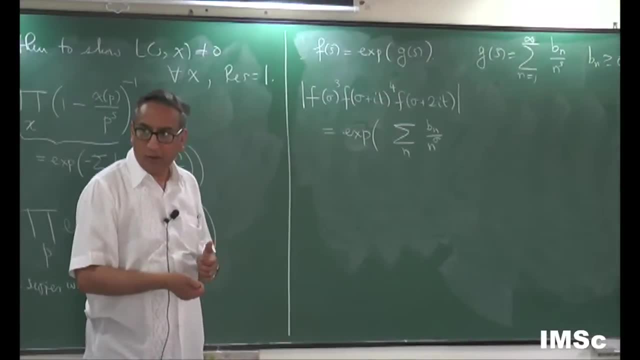 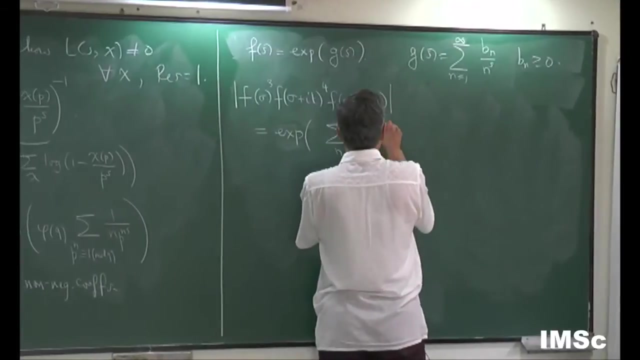 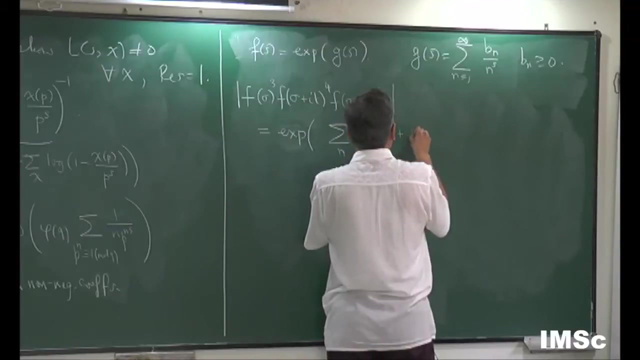 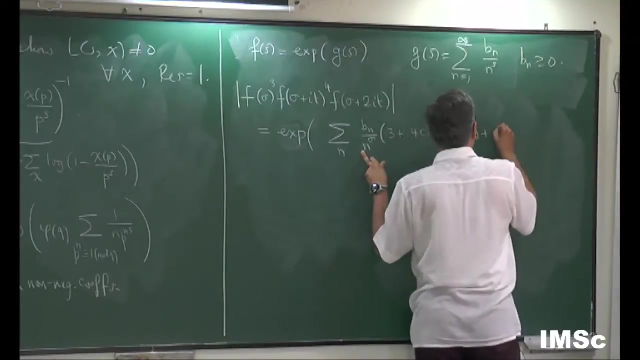 Okay, I'm going to now take absolute values. Remember, with the same old absolute values. so the log of z is equal to log of the absolute value of z, plus i times the argument right. So if I take that, then you'll see that this is really 3 plus 4 cos t log n plus cos 2t log n. 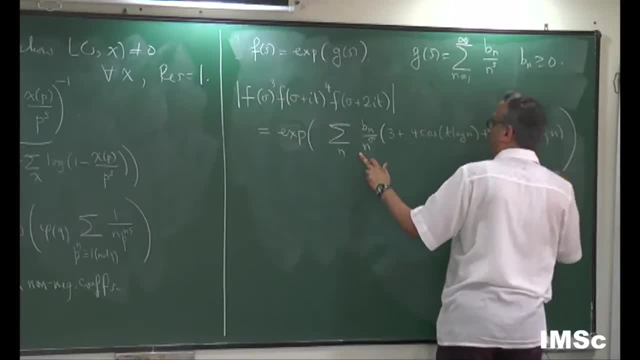 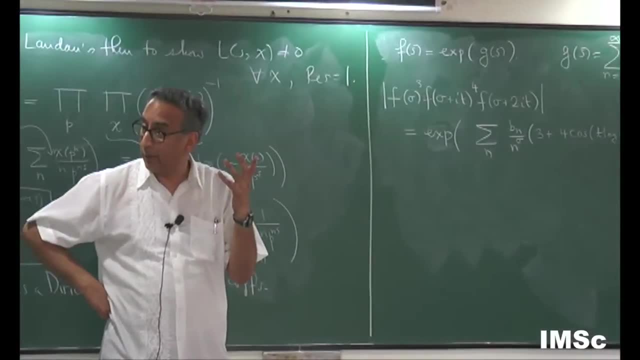 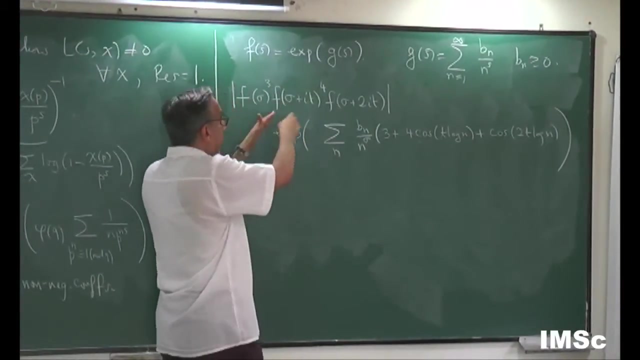 So that's what that is. Do you want to see this? Because that's exactly what we did in the Riemann zeta case. In the Riemann zeta case, we also had that. When we take the absolute value of this, 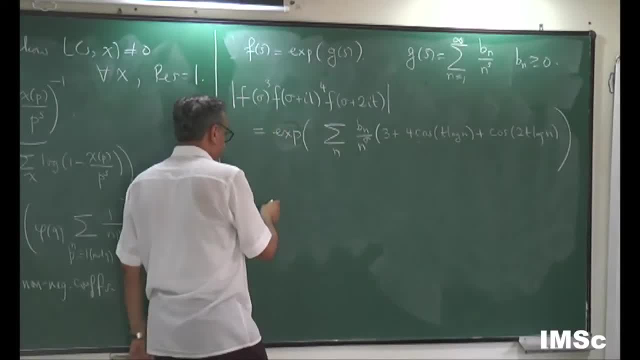 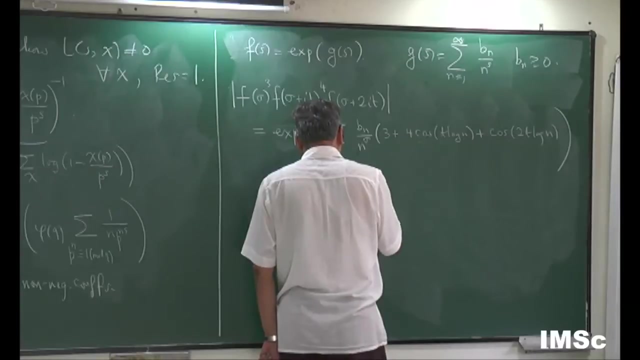 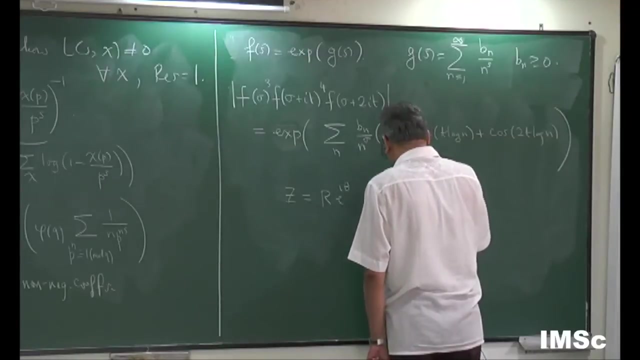 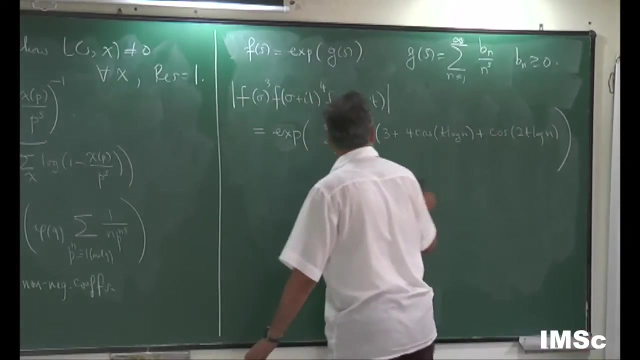 complex number. what am I saying here? I'm basically saying that e to the- let's see z- can be written as a constant. So that's what we did in the Riemann zeta case. So that's what we did in the Riemann zeta case. So that's what we did in the Riemann zeta case. So that's what we. 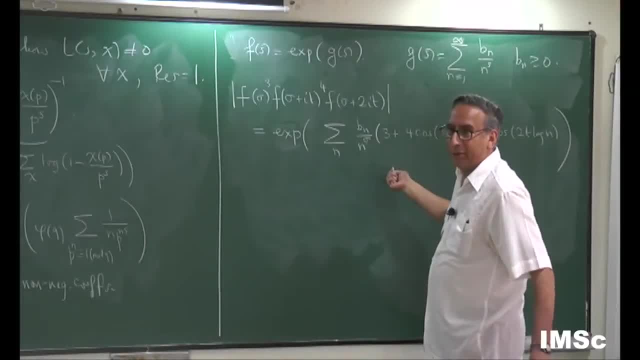 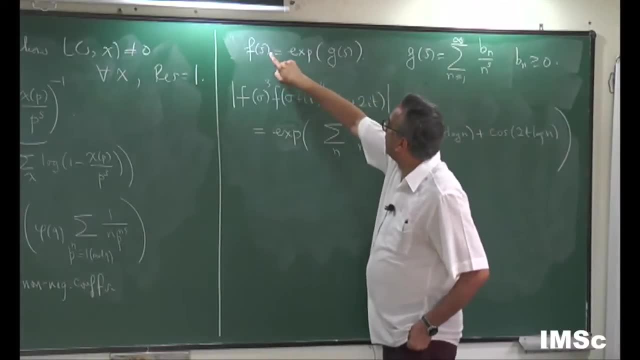 Can I just leave this as an exercise, or do you want me to? Okay, So what's going on here is you have this: 3 times g of sigma plus 4 times g of sigma, plus i t, plus dot, dot, dot, and what we're doing 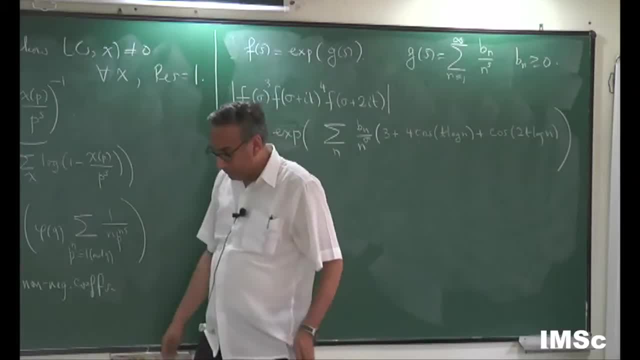 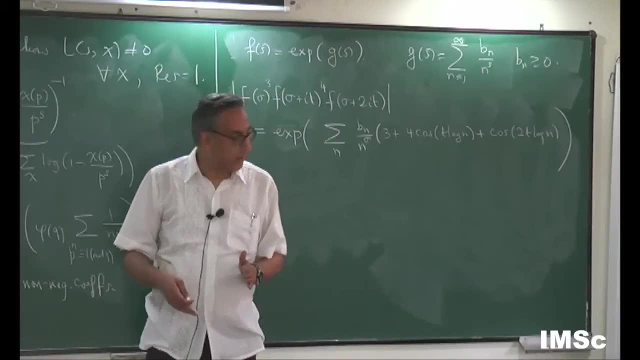 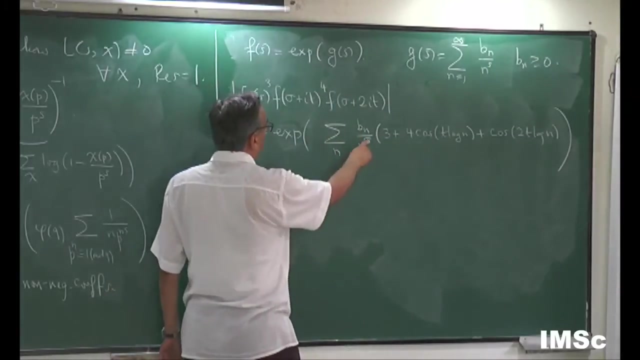 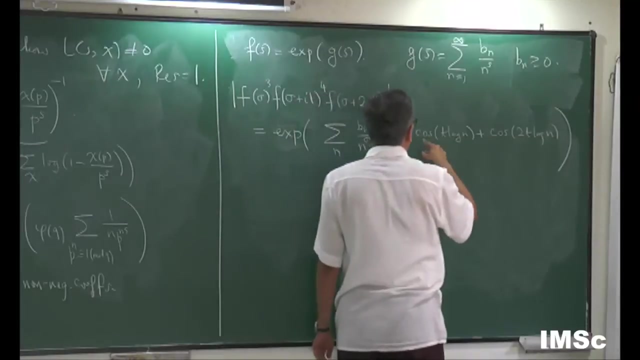 is when you take. when you take that, remember, um, the um, essentially you're taking the real parts of the um, of this combination. so so when you, if i were to have put this thing in here, it would have been 3 um n to this i t. well, 3 um, 4 over n to the i t, and so i'm just taking the real parts. 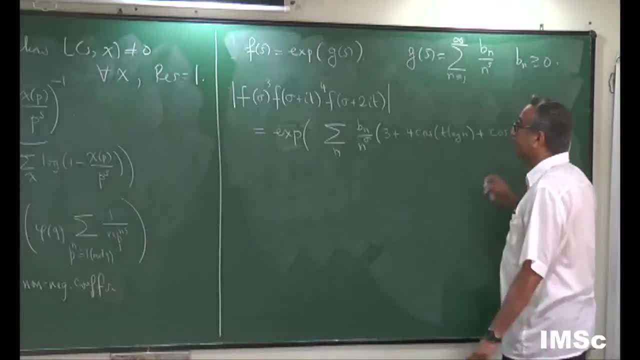 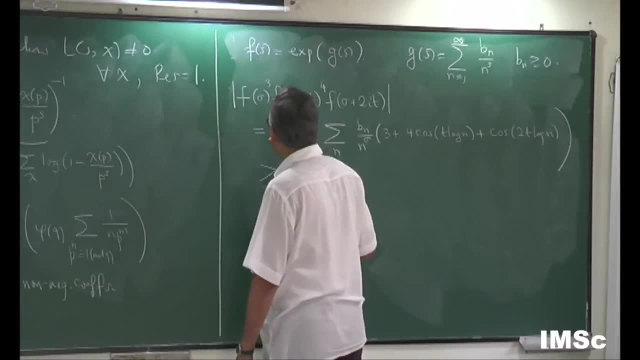 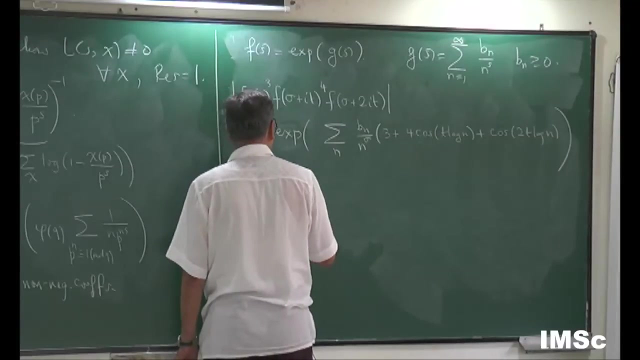 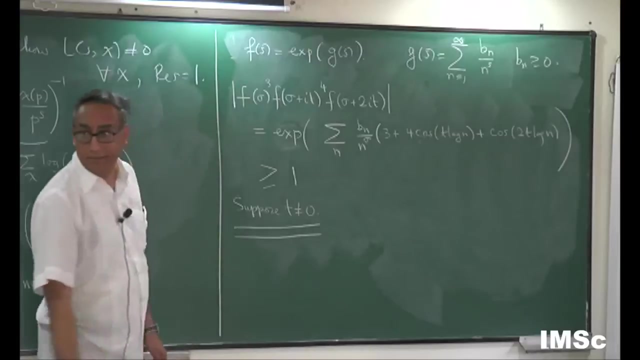 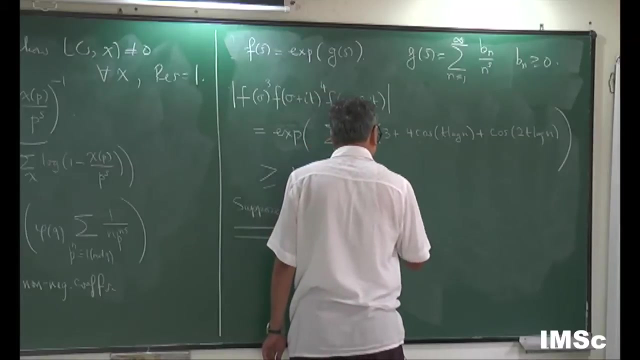 and this is what you end up getting. okay, so now, this is non-negative, therefore. uh, the whole point is that this is bigger than or equal to 1. okay, and we now suppose, let's suppose t is not zero first, suppose t is not zero and suppose that if f of 1 plus i t equals zero. then 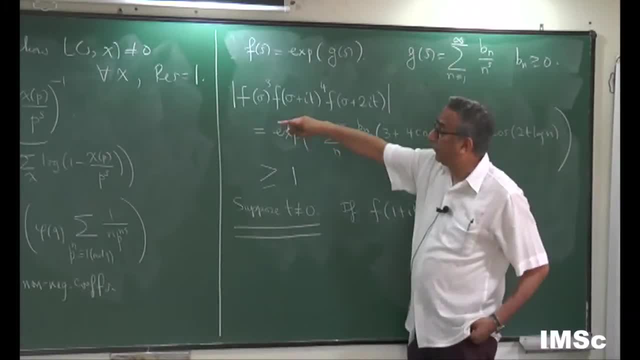 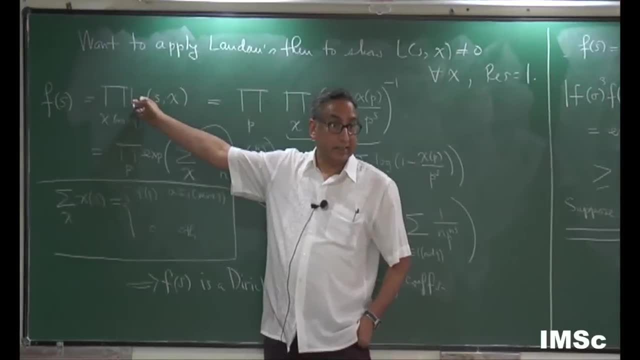 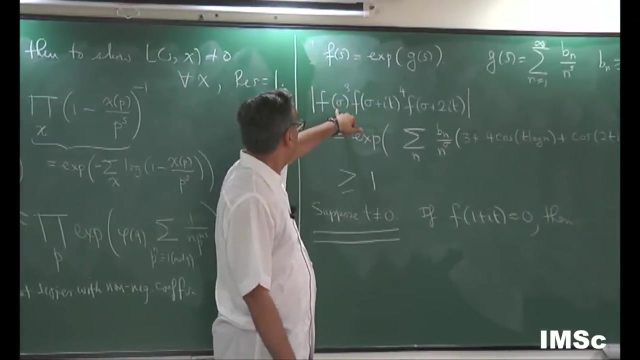 what happens. well, remember that one of these things is the Riemann zeta function at chi equal to chi, naught, and that's got a simple pole. so therefore, f of sigma, f of s has a simple pole at sigma equals 1. therefore there's a pole of order three here. 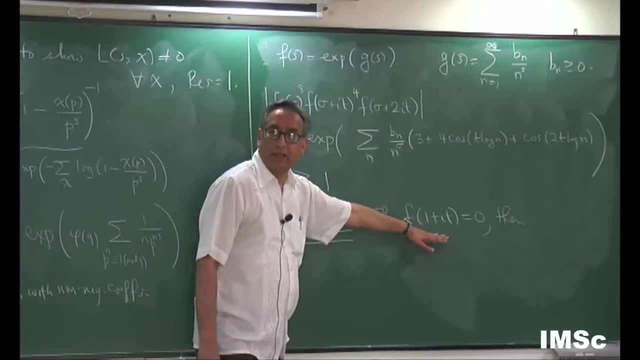 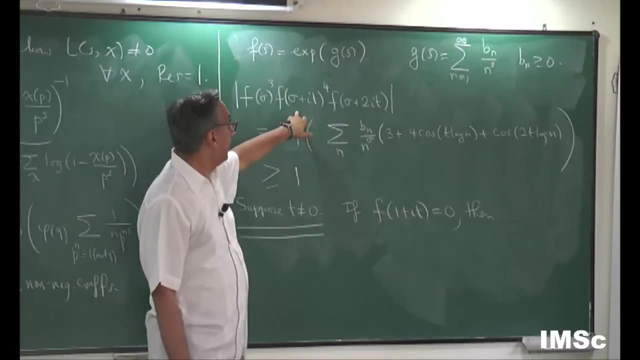 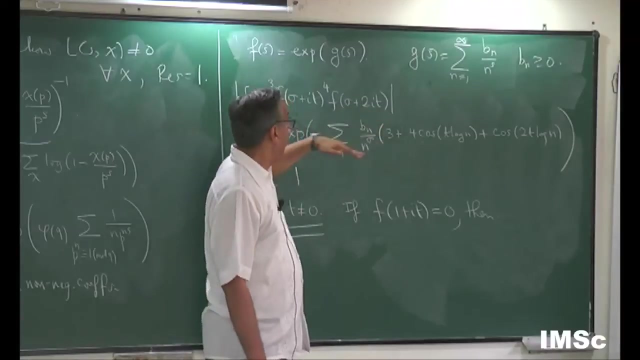 and if, if it happens that f has a zero at 1 plus i t, that'll introduce a zero of order. four at sigma equals one, okay, and that would cancel that pole and make the zero dominate. and then this guy's analytic, and therefore as limit, sigma tends to one, the, the uh, left-hand. 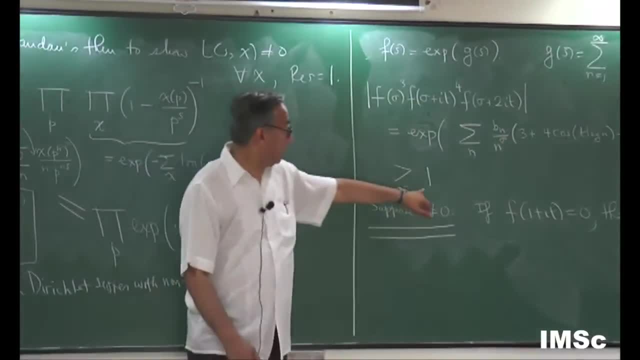 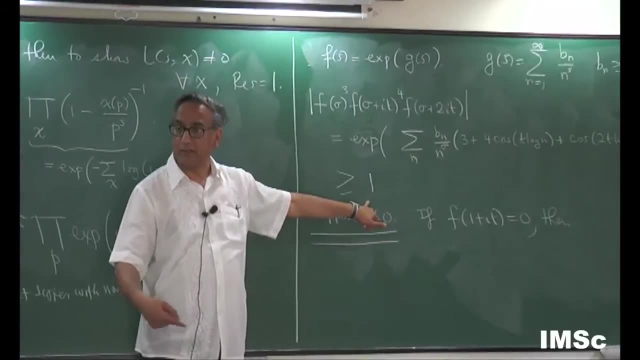 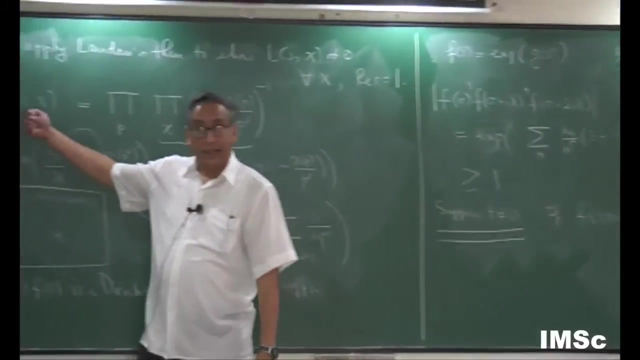 side should tend to zero, but it is. it shouldn't because? okay. so this, this argument, the argument that was used to show the Riemann zeta function doesn't vanish on the line. real part s equals 1 actually works for LS chi's also, because none of these things will vanish provided you create. 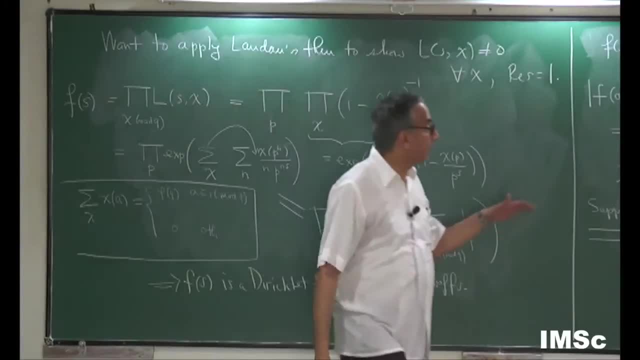 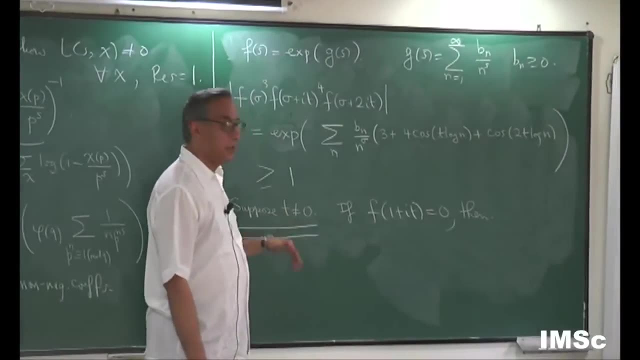 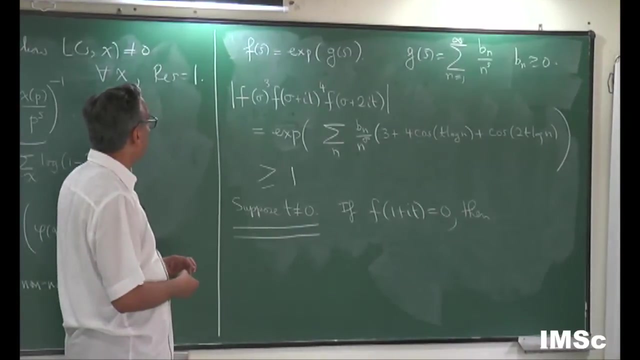 use this function instead of the zeta function, and the argument more or less runs along this line: everybody okay with that. now why did I have to assume T naught equal to 0? why do I have to assume T naught equal to 0 in this proof actually? 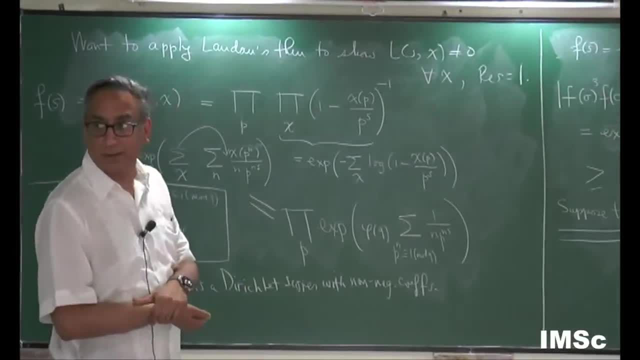 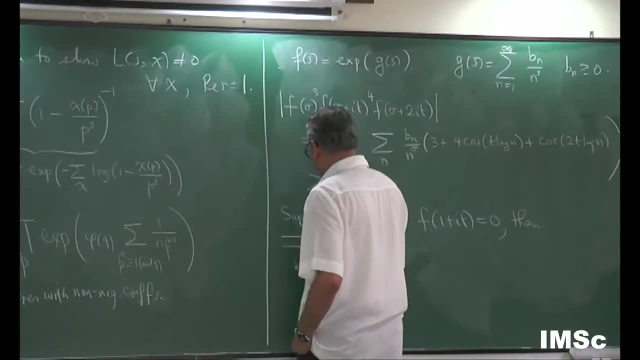 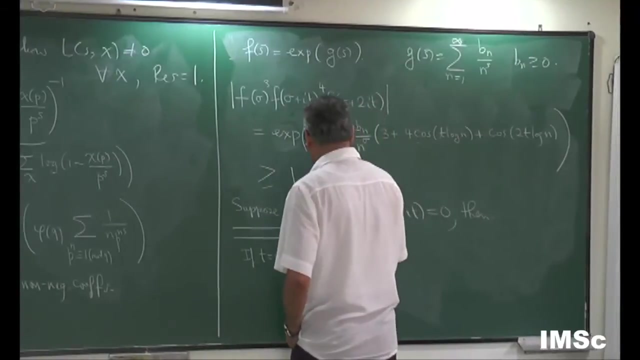 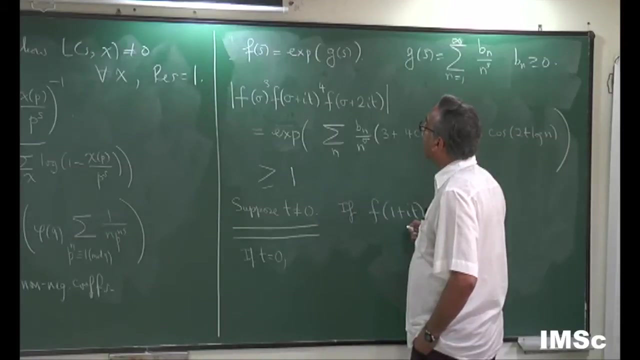 actually this proof works, doesn't it? if T equals 0? if T equals 0, then, and I guess if T equals 0, there's there's a part of a problem, right? because then I'm looking at yeah, I'm looking at yeah, exactly, if T equals 0, I'm looking at F. 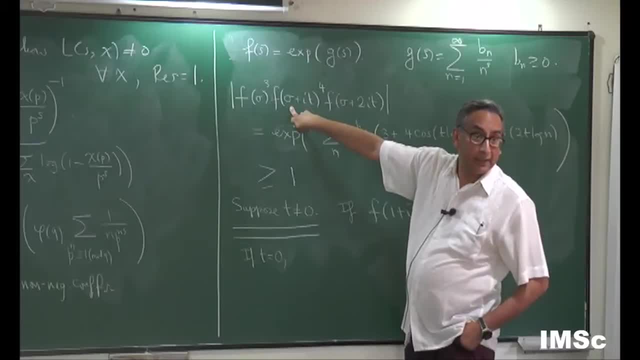 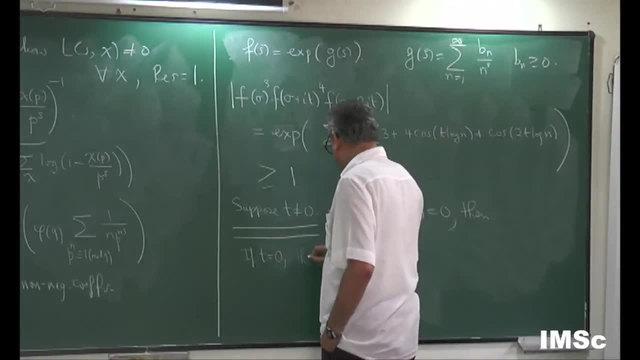 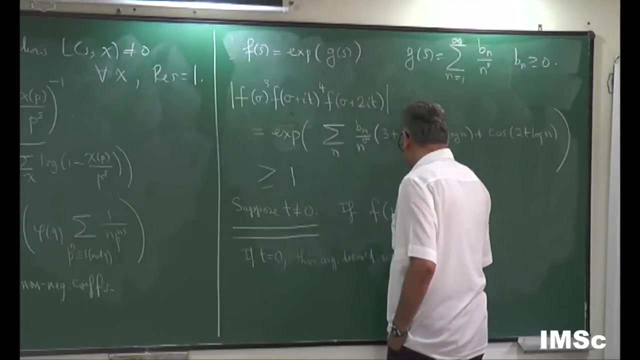 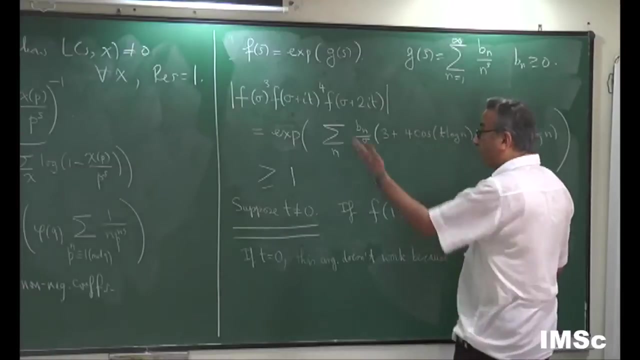 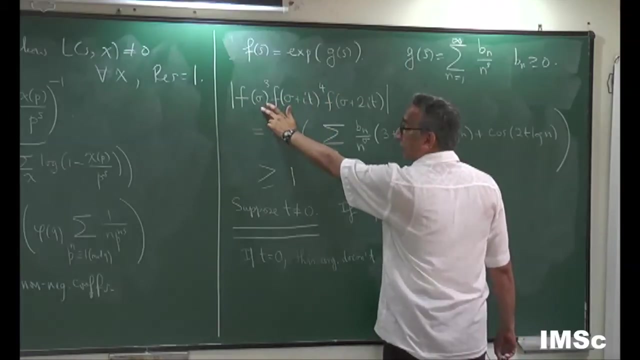 at 1, right, and that's got a pole again. so if T equals 0, this argument doesn't work. this argument doesn't work because because there's still a pole there. so if T equals 0, I've got a pole of order 4, a pole of order 3, you know, and so this whole thing's got a pole and there's nothing. no, 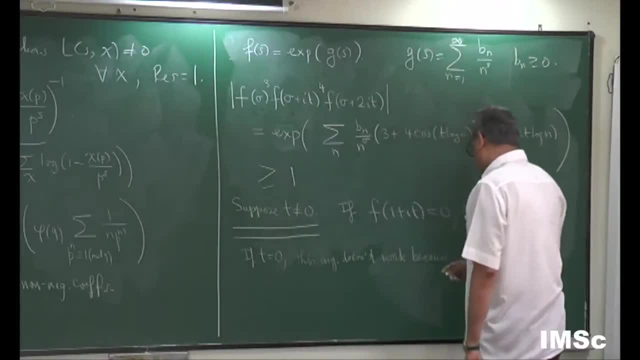 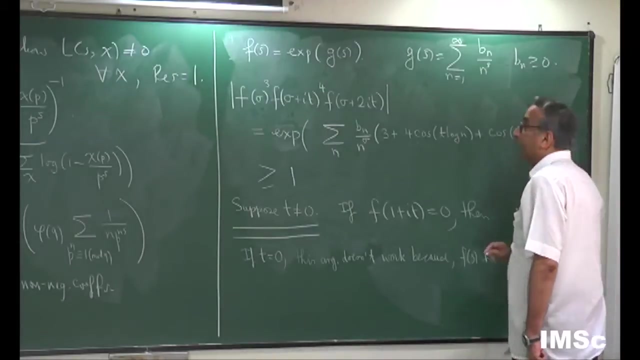 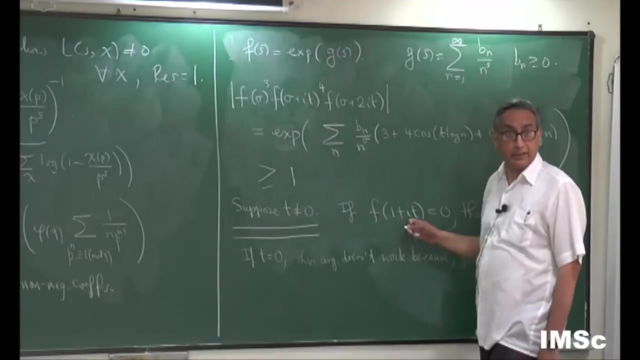 contradiction: sigma goes, it explodes, all right. so this started because the limit process doesn't work, because F of s has a pole at s equals. so if I was dealing with, if I wanted to show F of F doesn't vanish for any other T which is not 0, this argument works. so that argument for the Riemann zeta. 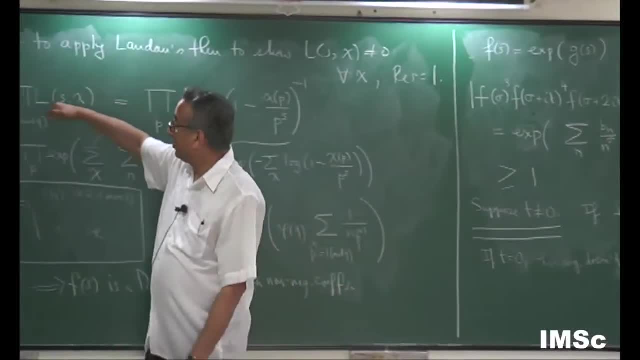 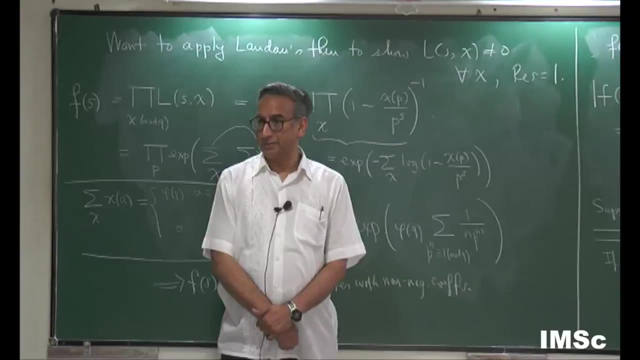 function case actually nicely translates to do this except at 1. except at s equals 1, so this argument fails, and this is this is actually the the heart of why Dirichlet had trouble. there's a small thing, you know. so sometimes, when we get into these snags, 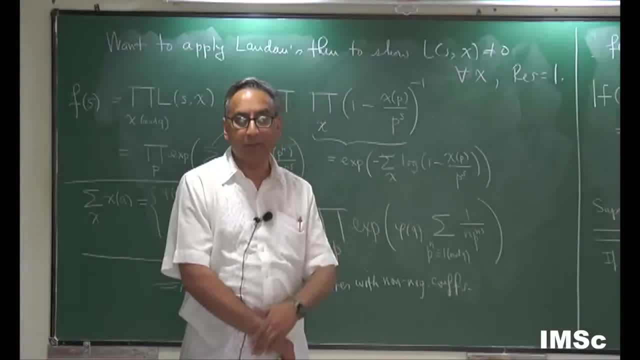 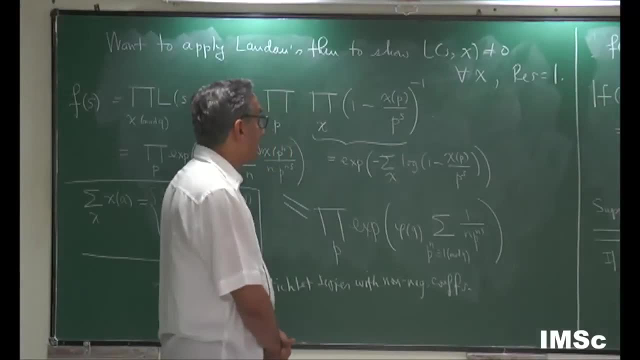 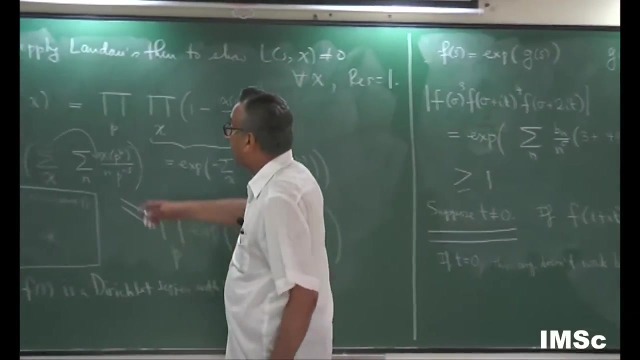 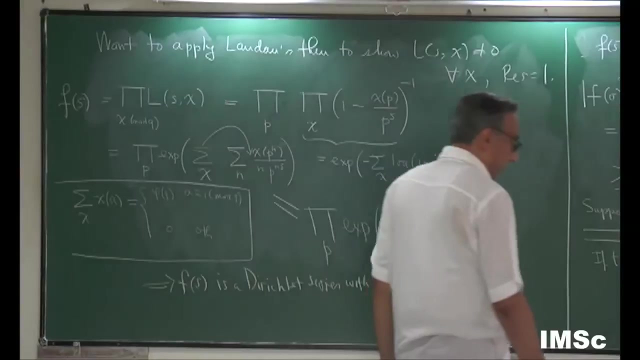 we're irritated, but that there's an obstruction, but maybe you're putting your finger on something extremely important and and he was, so let's try and see what. how to deal with. T equals 0. well, if you, in that case, if L1 chi, you want to show L1 chi is not 0, okay, so if L1 chi were 0. 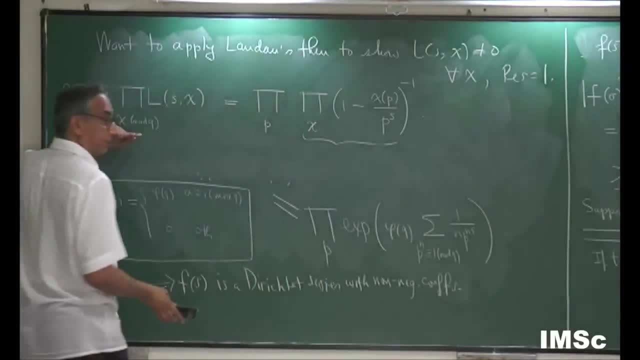 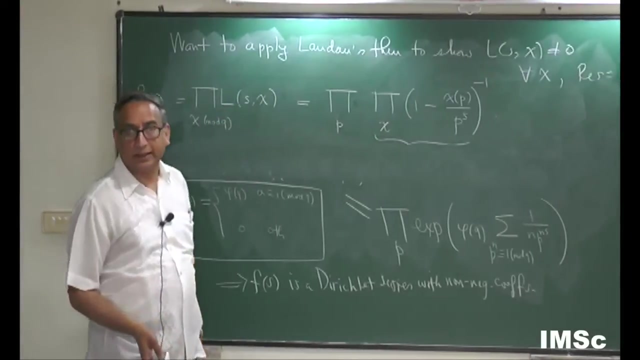 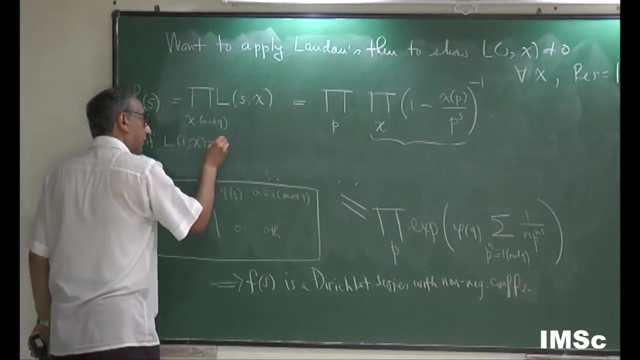 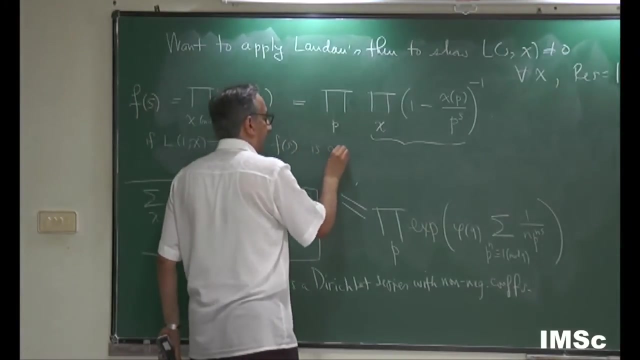 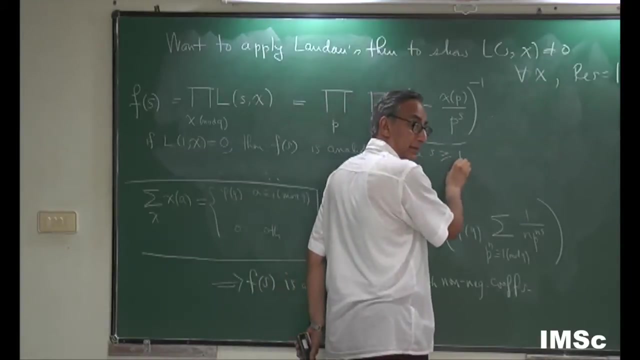 then what happens in this product? in this product, the pole at s equals 1, coming from the trivial character, is eliminated by the 0 and from L1 chi. so okay, if L1 chi equals 0, then F of s is analytic for real part s greater than or equal to 1. the pole got eliminated right before we knew. 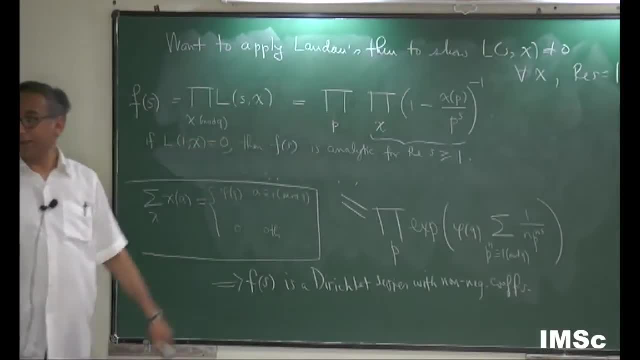 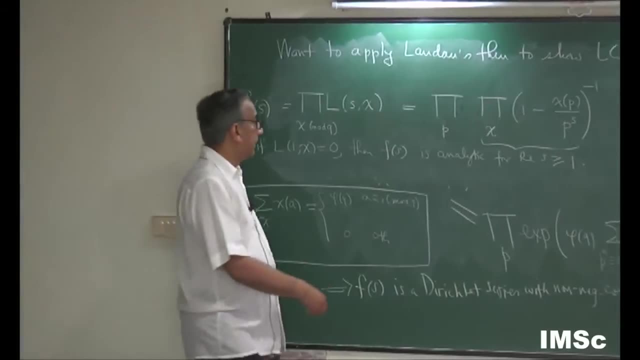 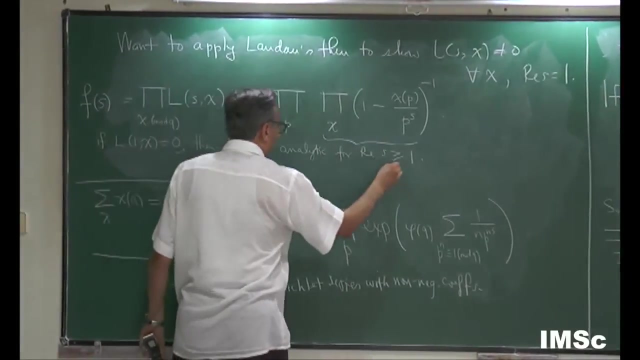 that this thing was analytic for real part of s strictly bigger than 1 and at s equals 1. it had a simple pole, we said, but it's now viewing zeta as as a factor there possible simple pole. so now if the pole got eliminated by a zero, then the thing is analytic for real part as greater than. 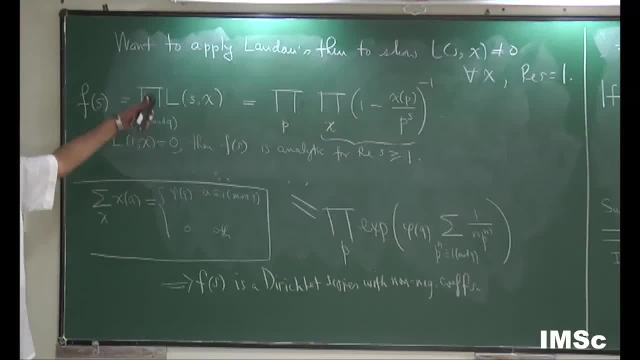 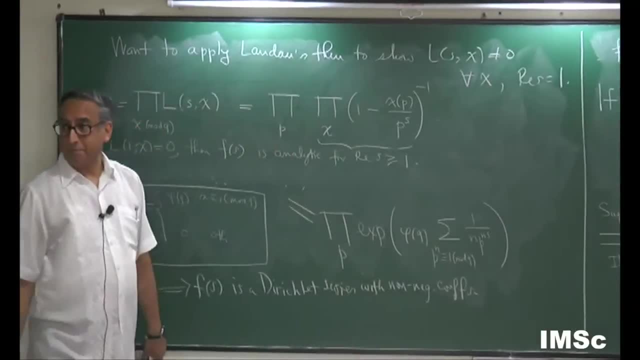 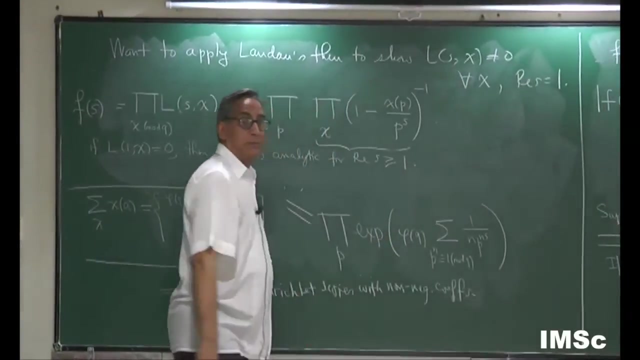 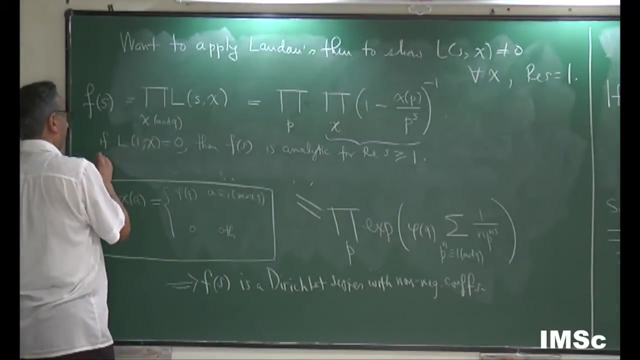 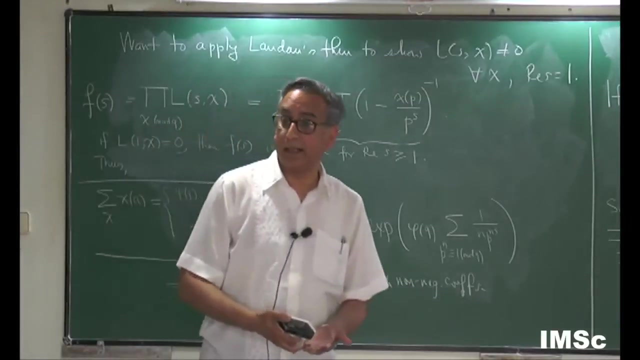 Ok, now Landau's Theorem is applicable, right, this is a Dirichlet series with non-negative coefficients from this concoction, non-negative coefficients is analytic for real part of as bigger than or equal to 1. therefore, what, therefore? it extends now f of s. thus we showed, remember we showed, the Riemann zeta function has an analytic. 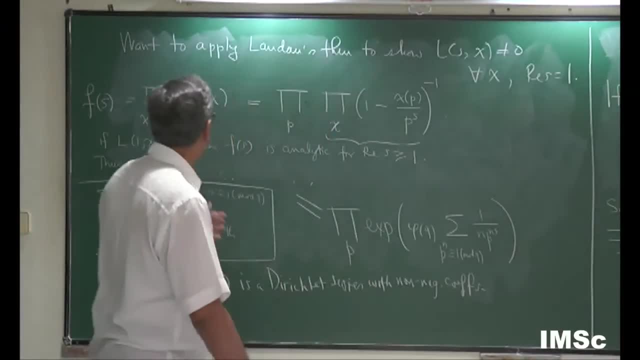 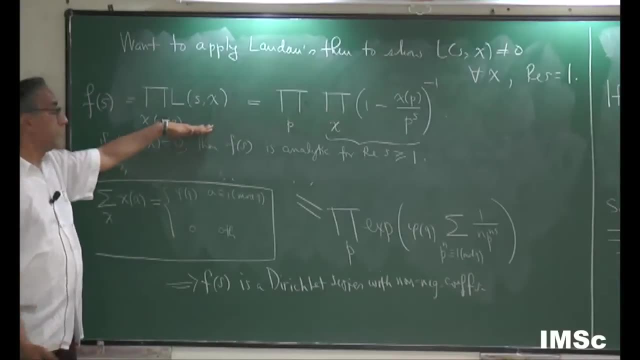 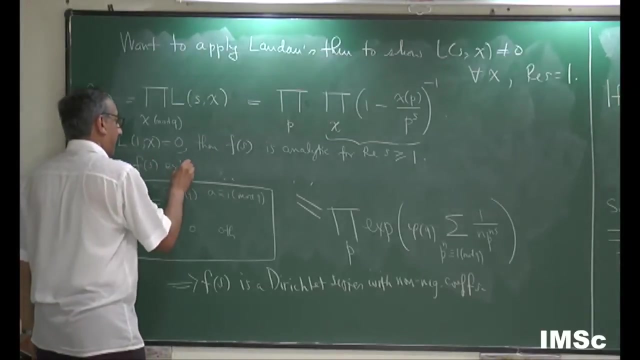 continuation for real part s bigger than zero, and we showed that all these Ls chi's were analytic for real part s bigger than zero. The pole got cancelled. now, therefore, this function is analytic for real part s bigger than zero. Thus f of s extends to an analytic. 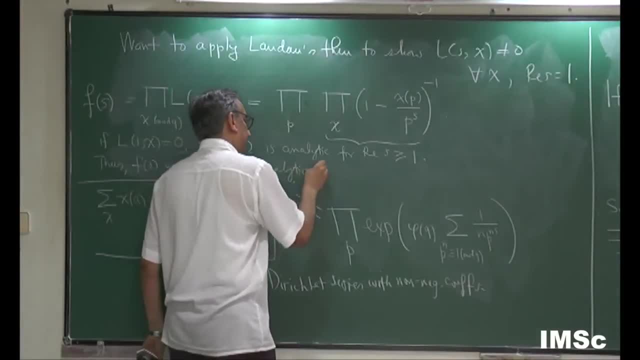 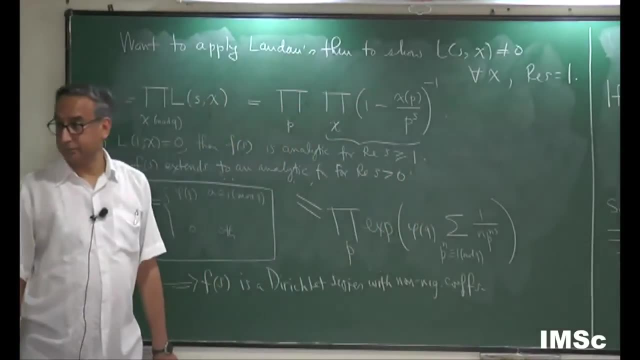 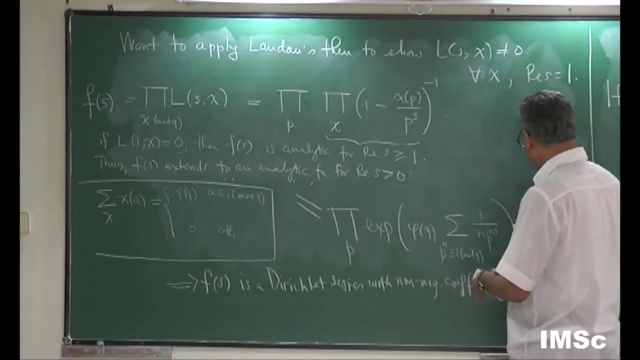 function for real part s bigger than zero. Okay, but let us see what is going on here. Let us see what is going on here. So that means, in particular, this Dirichlet series should converge for any number with real part s bigger than zero By Landau's theorem, right? Landau's theorem says: if you 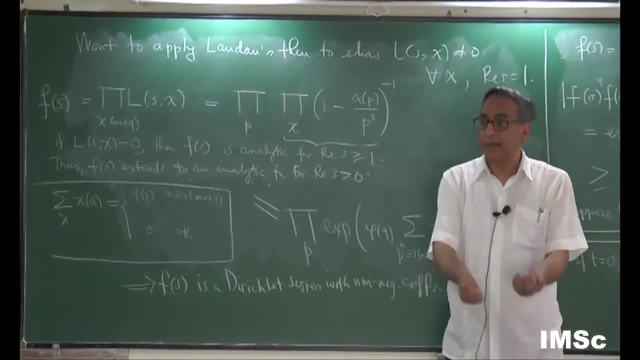 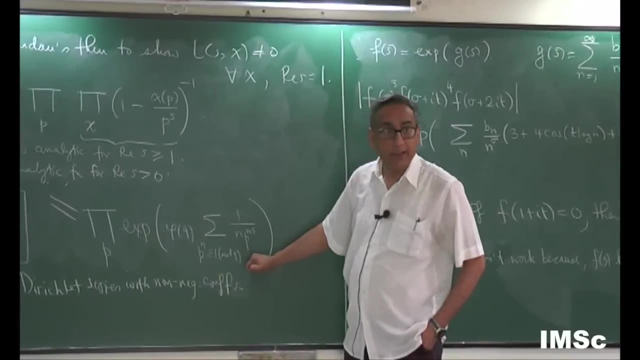 have an analytic continuation for real part s bigger than zero. the Dirichlet series actually converges there now, So therefore this Dirichlet series has to converge for any point, for real part s bigger than zero. In particular, it should converge for s. 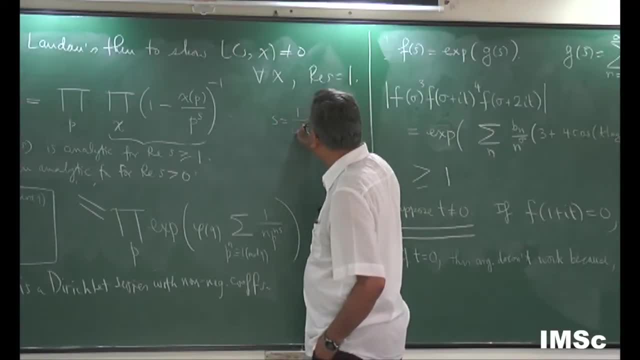 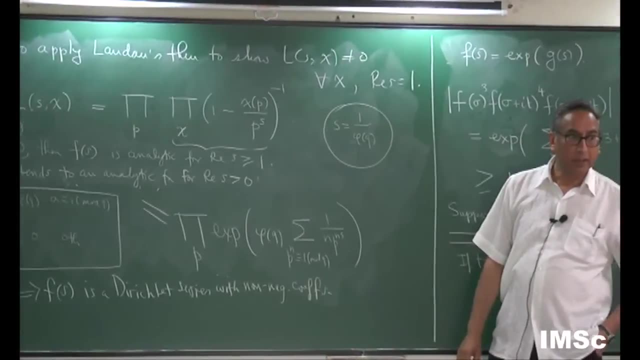 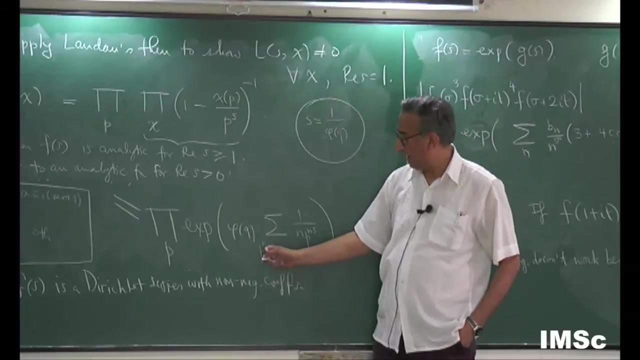 equals 1 over phi of q, which seems to be positive number. okay, Now notice that every prime satisfies this congruence with n equals phi of q. That is Euler's theorem. See. Euler's theorem tells you that p to the power of phi of q 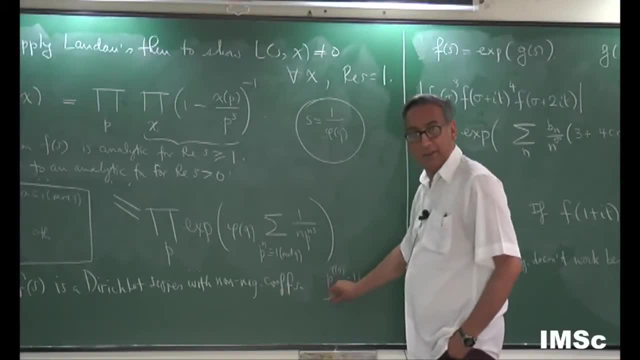 is always congruent to 1 mod q, right? That is Euler's little Euler's theorem. So you can see that Euler's theorem does not make any sense. As soon as you vary from 1 to 1, you will find that here. you will see that, of course, that Euler's theorem does not make. 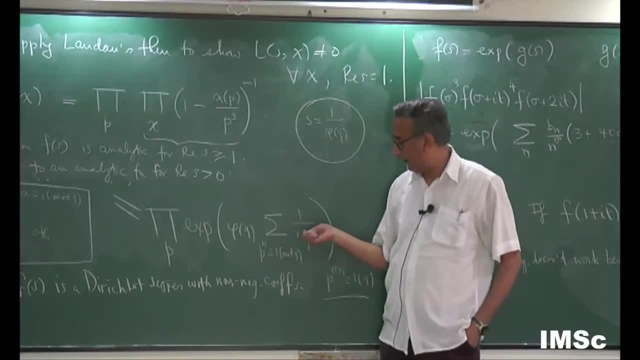 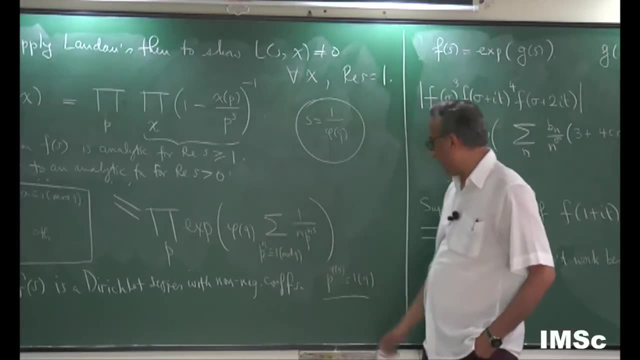 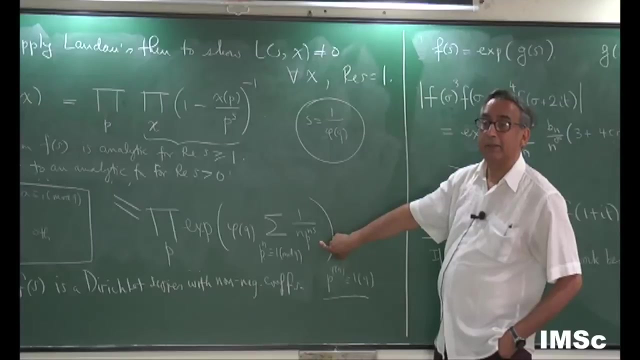 right. So that means every prime is going to appear here, every, yeah, so every prime and phi of q. So now what happens when I plug in s equals phi of q is that I'm going to get a 1 over p as a contribution. 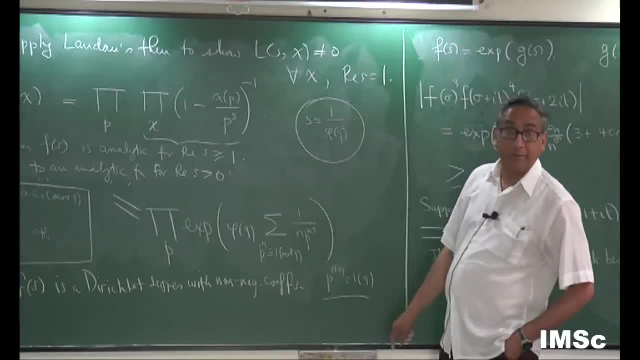 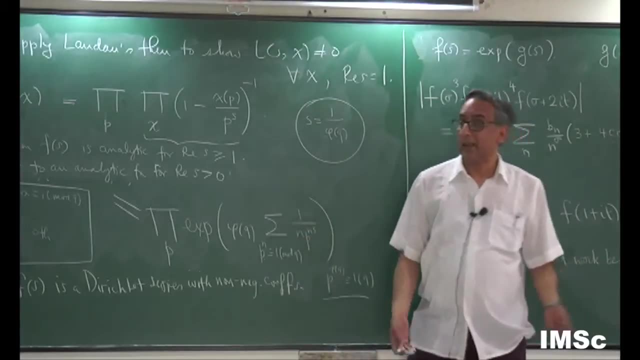 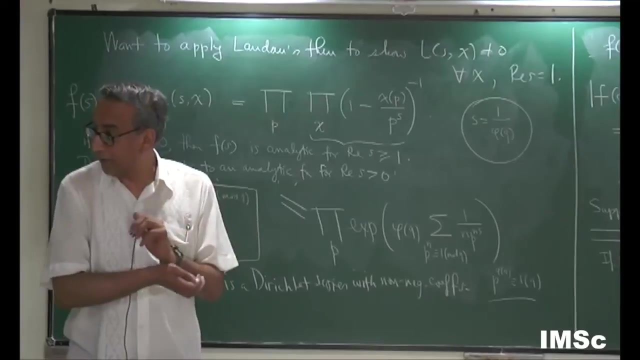 Okay, n is n is equal to phi of q, s is equal to 1 over phi of q and there's going to be summation 1 over p. but the sum of the reciprocals of the primes, remember, diverges and therefore it can't converge because otherwise, right, we kind of saw that from earlier. 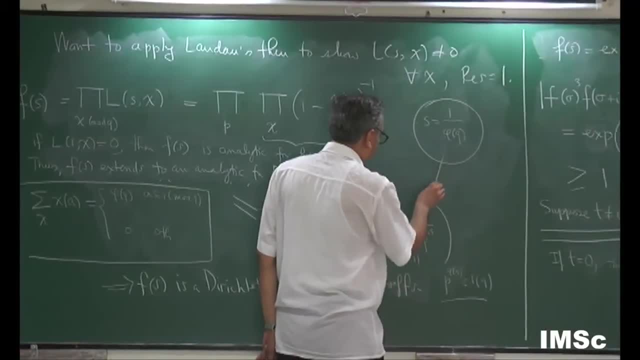 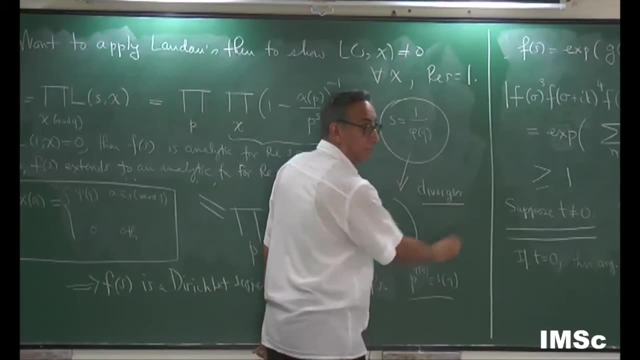 work. therefore, this actually diverges. So at this point, this series diverges. So that's the proof that L1 chi is divergent. So that's the proof that L1 chi is divergent. So that's the proof that L1 chi is. 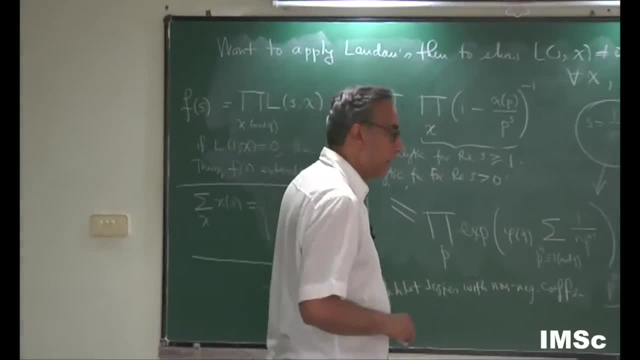 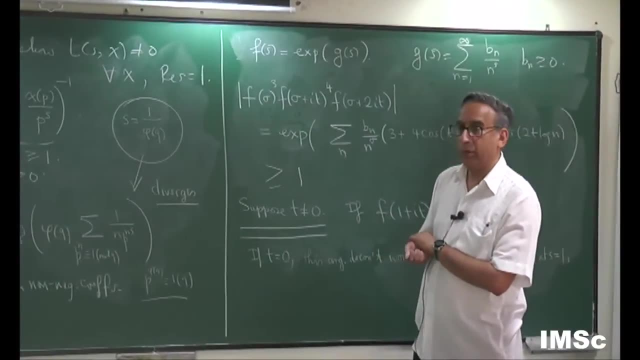 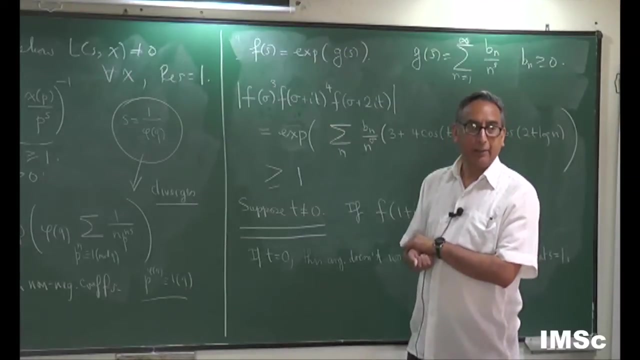 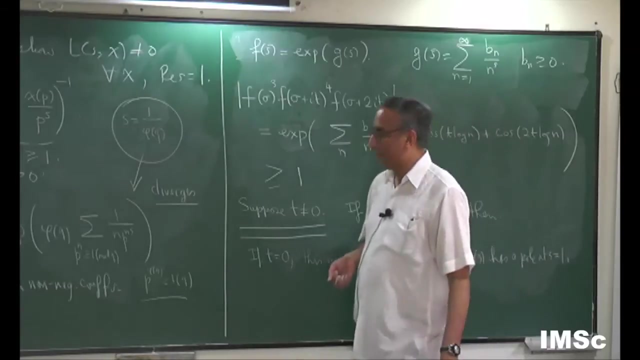 not 0. So the point at s equals 1 is actually a very subtle point to analyze and it requires a little bit more care. How did Dirichlet circumvent this problem? He actually calculated L1 chi explicitly. I mean, he did realize that there was. here's how he did it. actually He realized that if chi was a 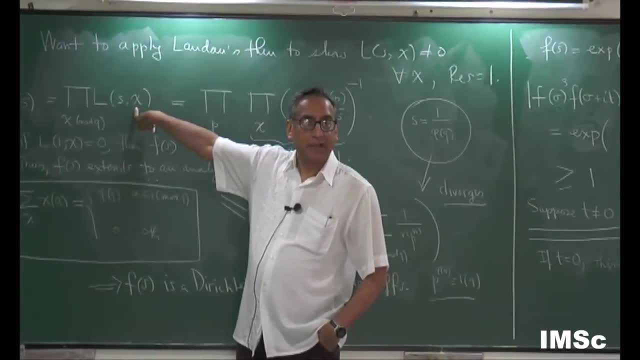 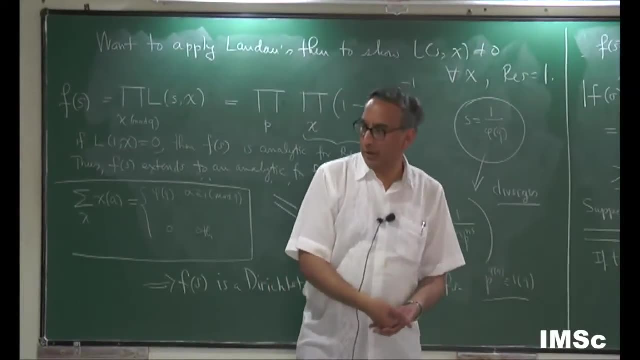 complex character. okay, if chi was a complex and L1 chi was 0, then L1 chi bar is also going to be 0. So you'll introduce a double order, 0, and but this guy- chi equals chi dot- has only a simple pole. therefore this: 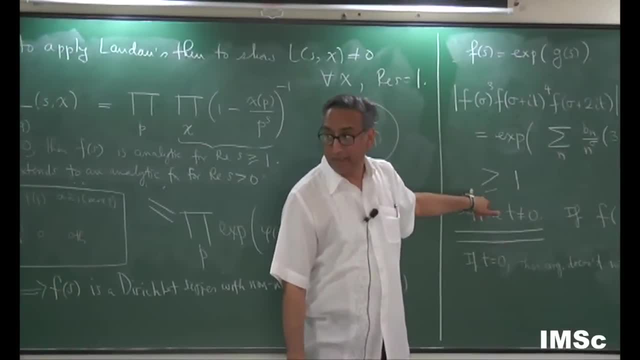 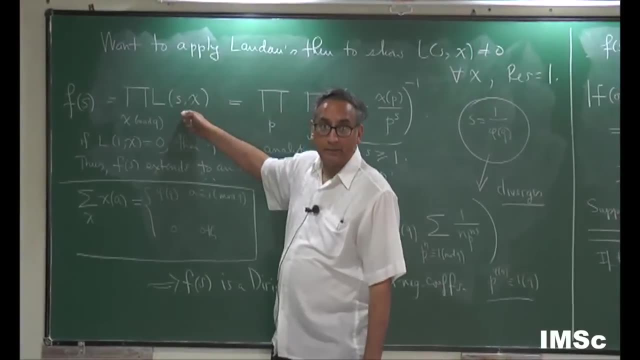 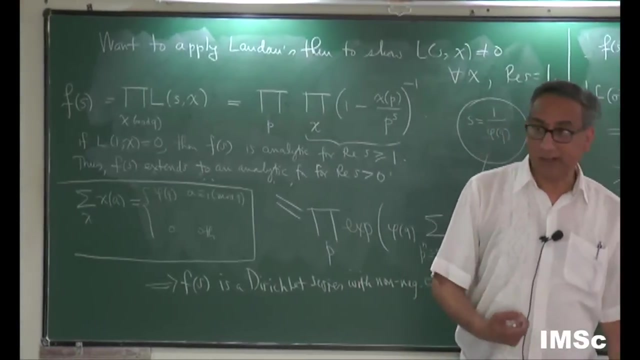 argument actually still continues to work in that case that the poles there's too much of a 0, if chi was not a real character. So the only problem we're all going to have is that you know if chi is a real character and when chi is a real character, Dirichlet went about going and 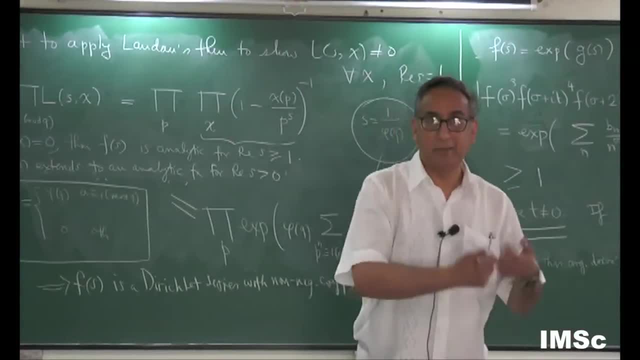 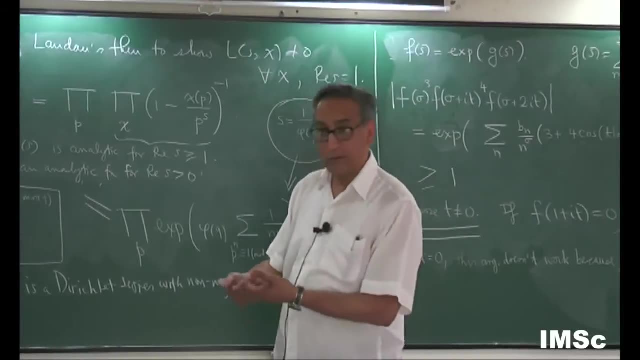 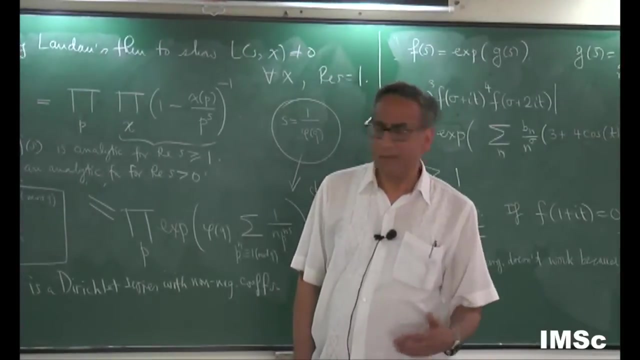 calculating what L1 chi is, He related it to the class number of imaginary or real quadratic fields and then showed that it's related to the order of a certain group and therefore it can't be 0. That's how he went about doing it- Very, very complicated way of getting it. But now, of course, 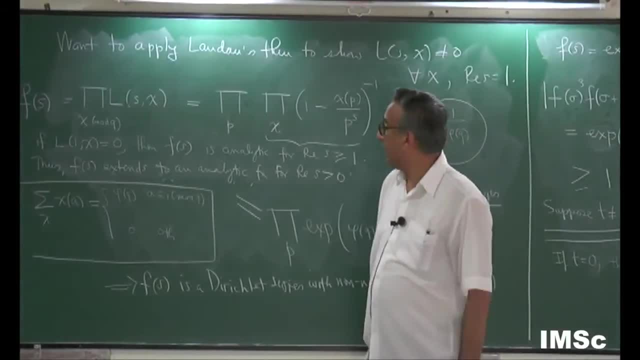 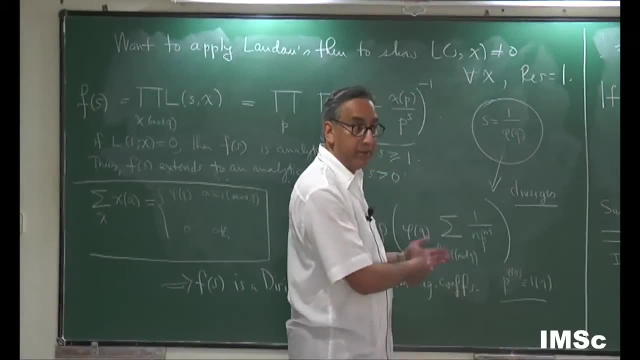 that formula is very important. It's called class number formula. It's very important. Okay, so that's the proof of the infinitude of prime. well, not infinitude, but we actually have the Tauberian theorem giving you asymptotic formulas. All right. 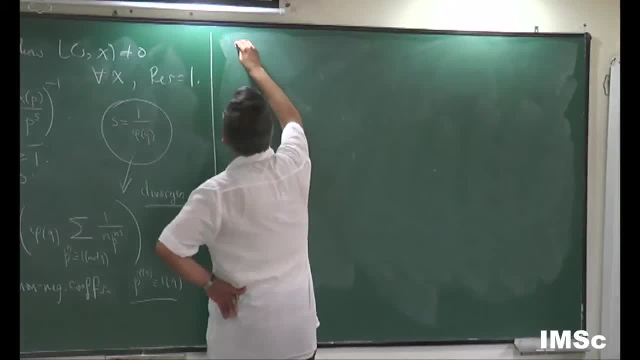 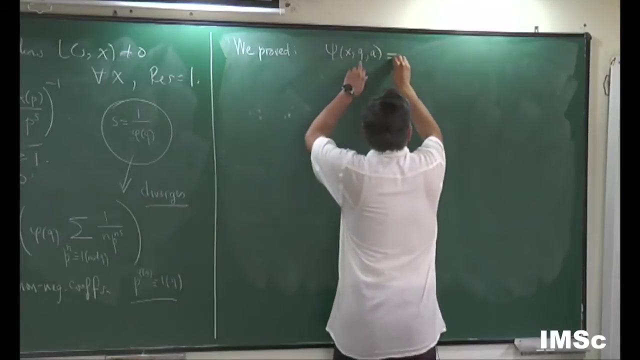 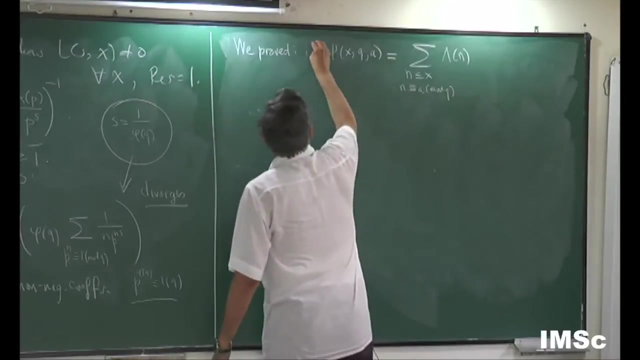 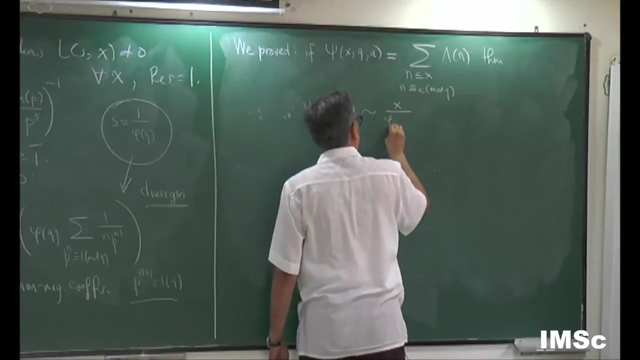 Okay. so let me make a few general remarks. So we've proved the following. We take psi x q a, Okay. Okay, If this is the definition, then psi x q a is asymptotic to x over i over q. 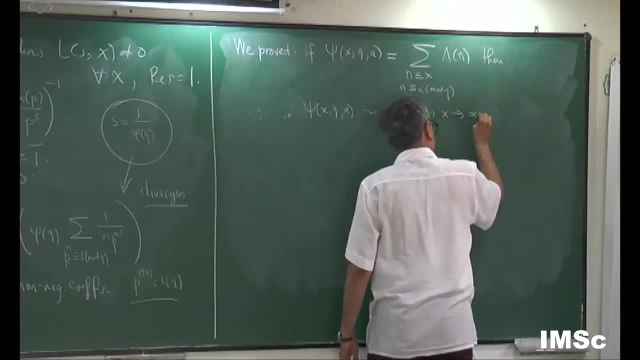 This is the definition. So if this is the definition, then psi x, q a is asymptotic to x over q. This is the definition. Okay, so I'll give you an example. So of course, A and Q are always relatively prime. 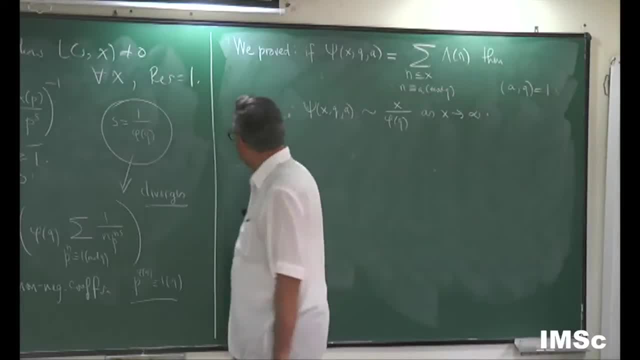 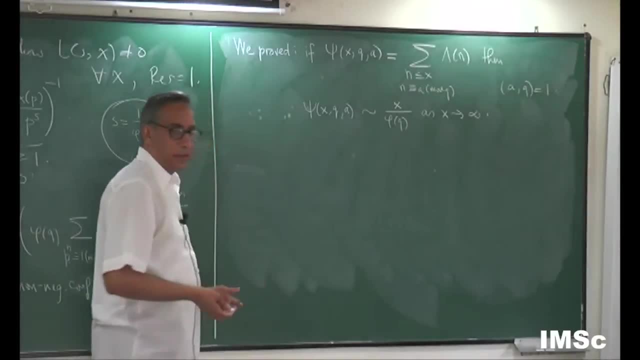 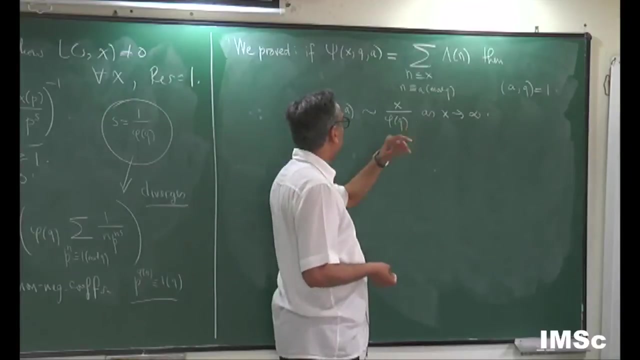 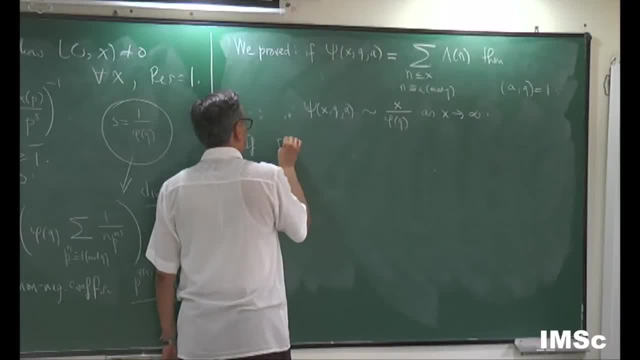 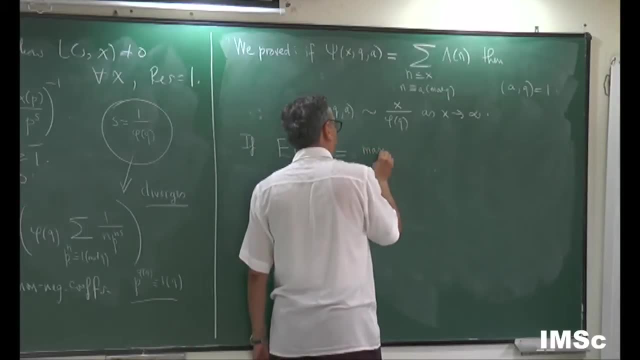 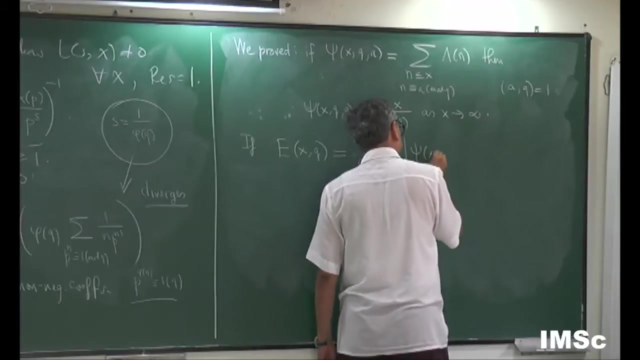 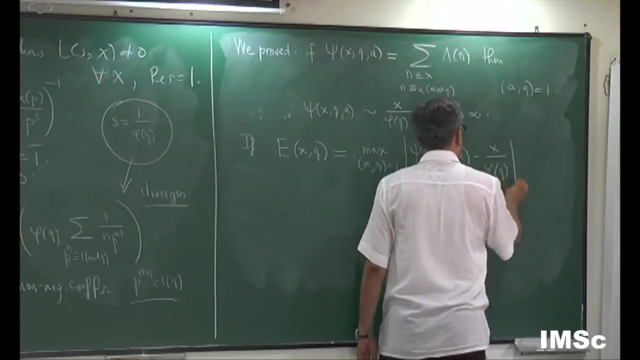 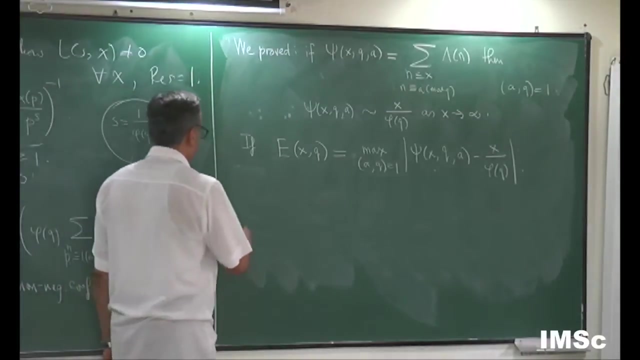 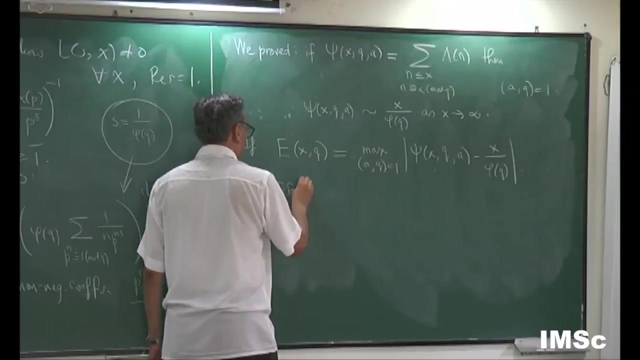 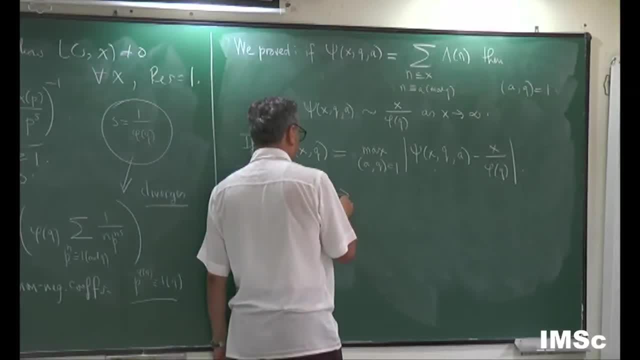 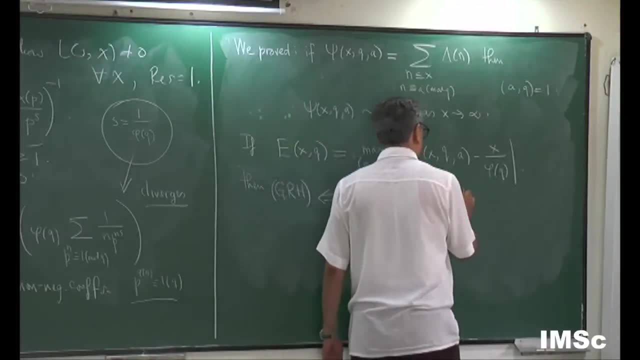 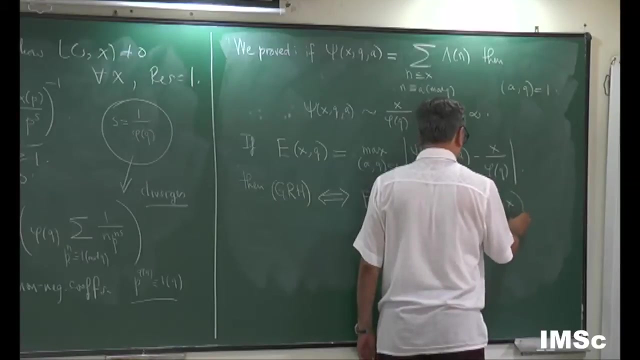 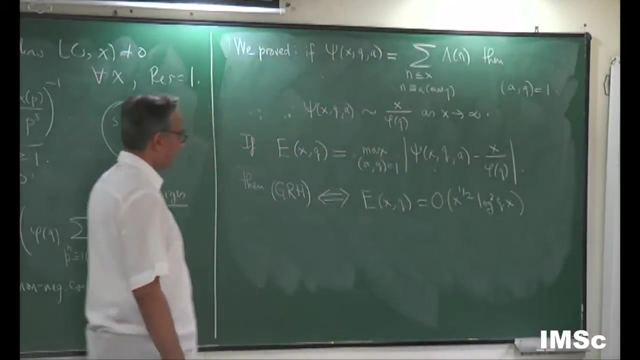 That's the generalized Riemann hypothesis, is equivalent to the statement that Exq is O of x to the half log qx. Is that right? Maybe I better throw in a square there, somewhere you know to be on the safe side. 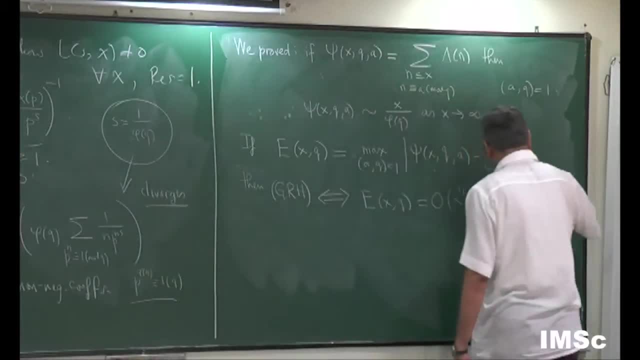 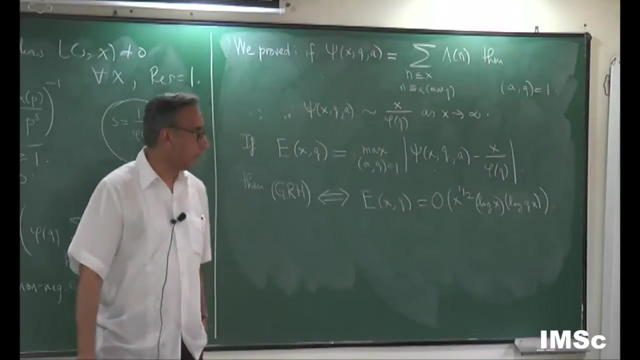 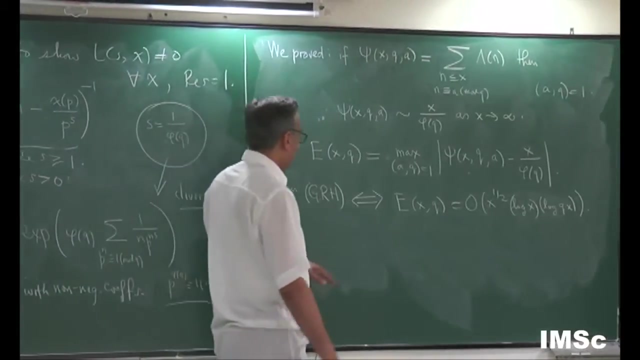 You know, let me put log x, log qx. only for the connoisseur is this distinction very important, but anyway, Okay, so that's the theorem. The q is not in the both of the logarithms. The Riemann hypothesis is equal to that. 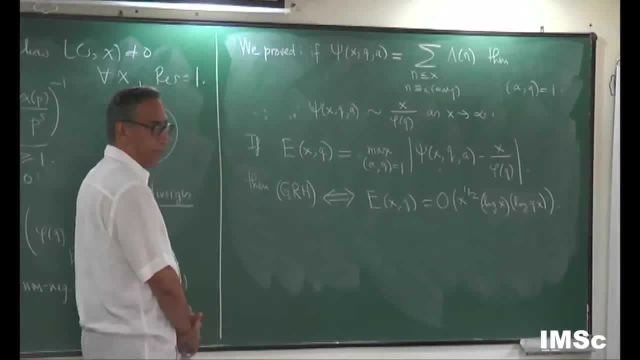 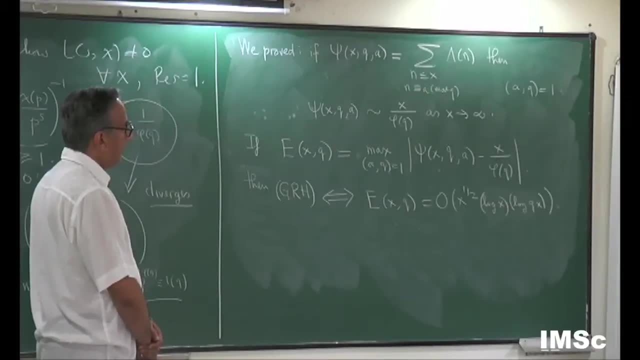 Unconditionally. if you fix q, you could make some statements about the error. but there are all these problems called problems with a real zero coming from again that real character, that nasty real character, And that makes these error terms not so neat and clean. 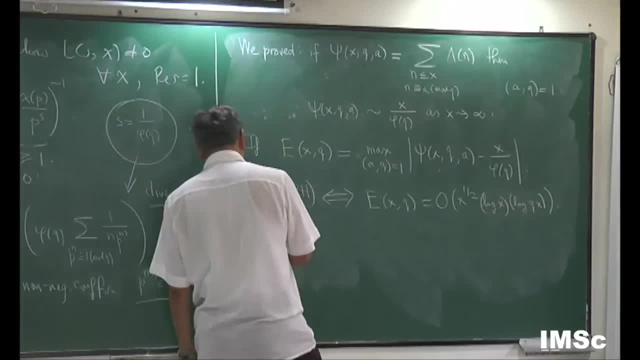 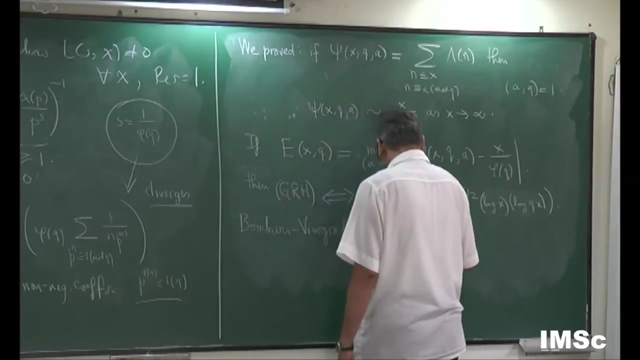 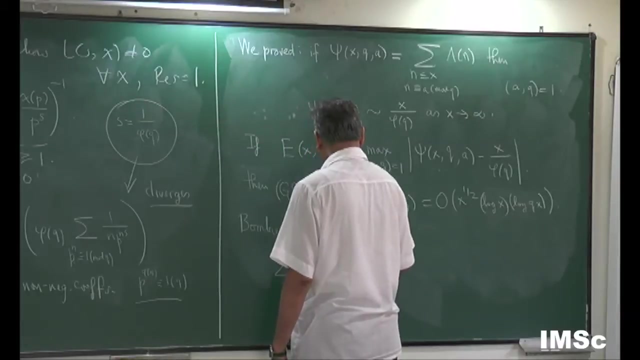 So I would all want to get into the discussion of here, But let me just point out there's a famous theorem of Bombir and Vinogradov Which tells you that if you take the Exq And you add this up, 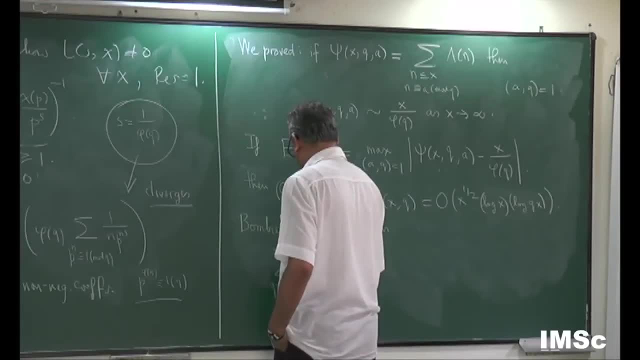 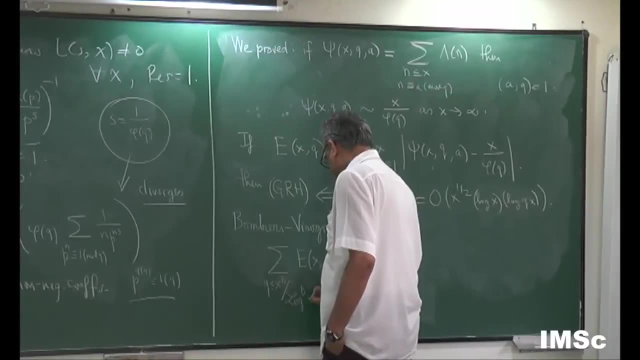 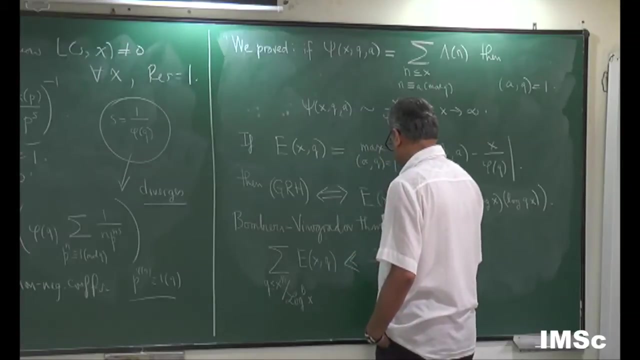 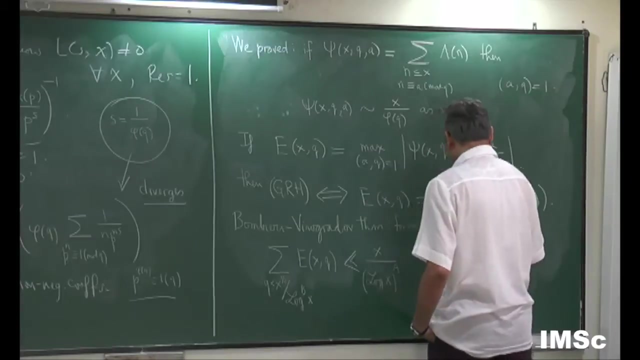 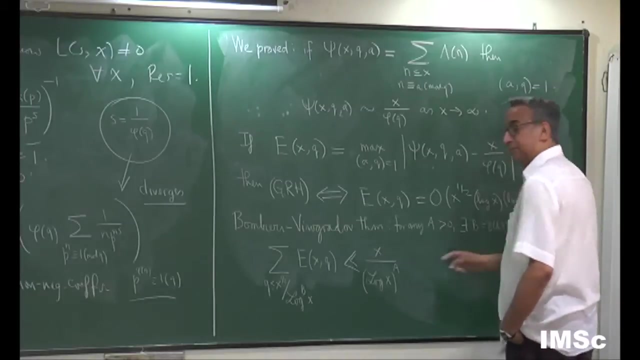 To x, to the half, over some huge power of logarithm, Then this is less than less than x over. So, basically, for any a Positive, There exists a b, which is a b of a, Such that this thing holds. 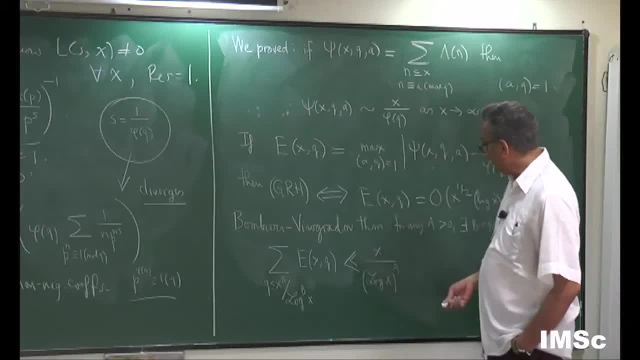 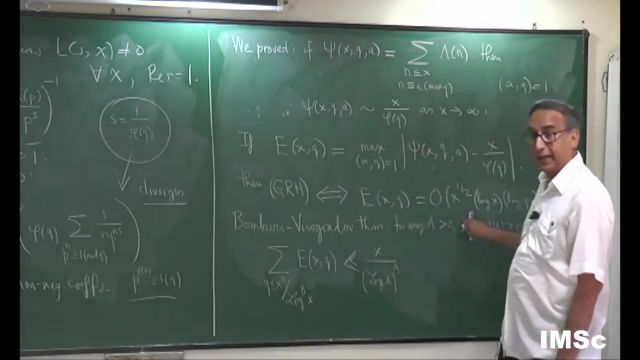 Now, what is the great thing about this? Well, the great thing about this is: this is an unconditional theorem, And if I had the Riemann hypothesis, each of these terms would be like root x. Each of these would be like root x. that's what it's saying. 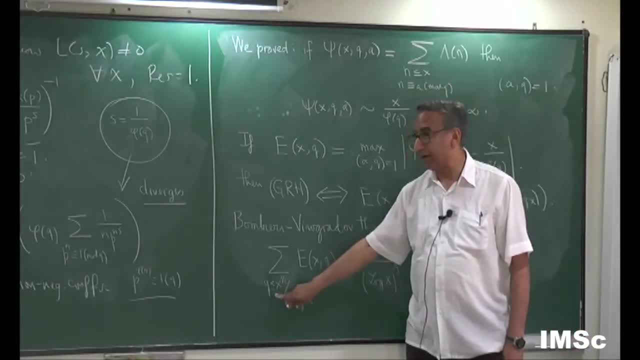 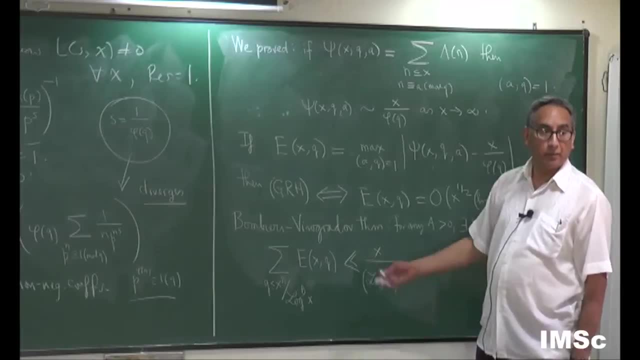 And then I'd add up all these terms. How many terms are there about root x? So I'm getting x over a power of log, So I'm getting an error term which I would get if I had the Riemann hypothesis. 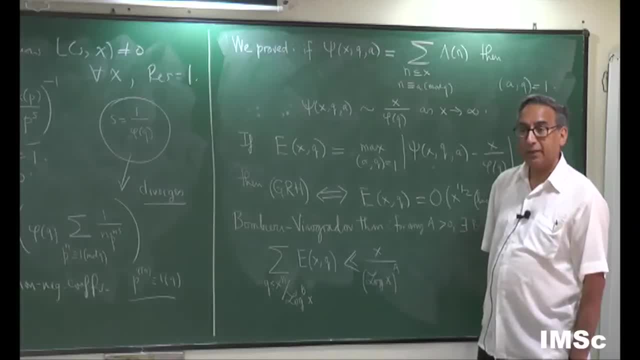 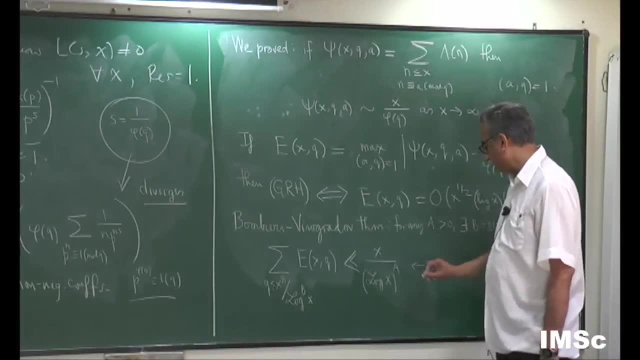 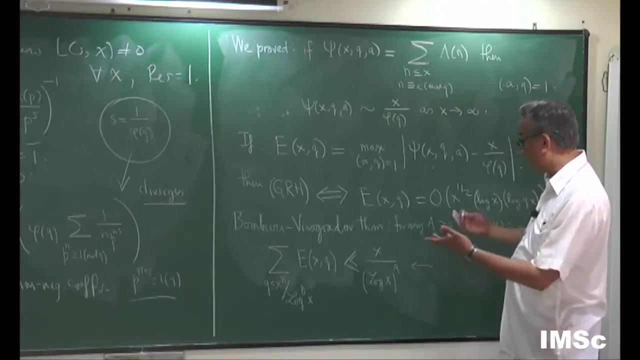 So this is an unconditional theorem And this- the fact that it's unconditional- means that you can apply this to lots of cases where you need the Riemann hypothesis, But you don't need to assume the Riemann hypothesis. 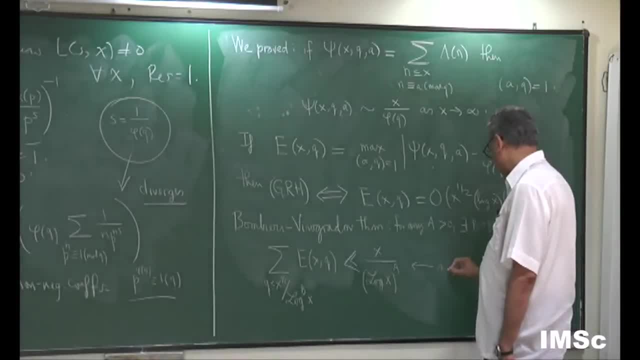 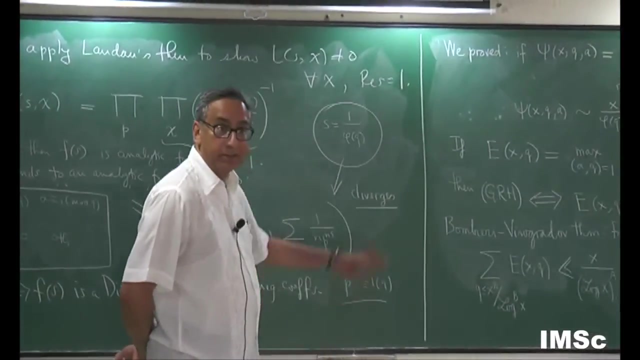 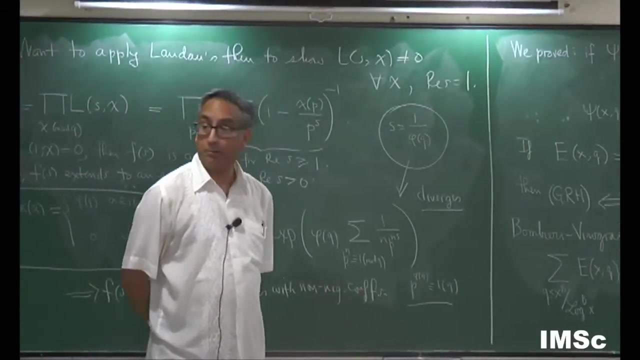 So this is often a substitute For grh In many problems. Some of you are- maybe you will be attending my lectures on new directions in sieve theory, where I'll talk about bounded gaps. This is one of the key ingredients in that theorem of bounded gaps between primes. 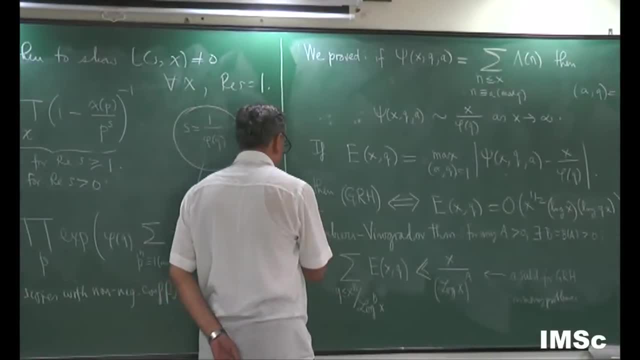 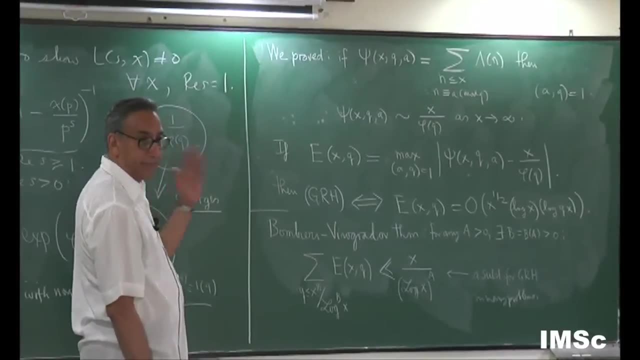 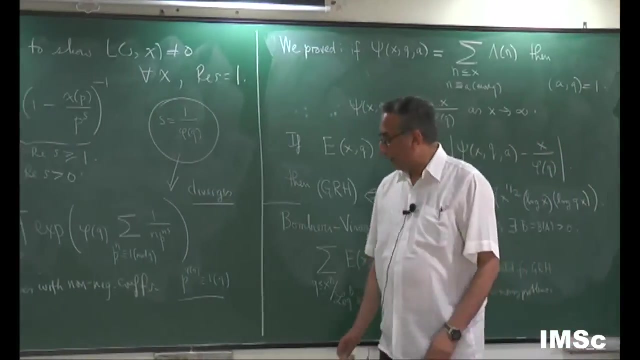 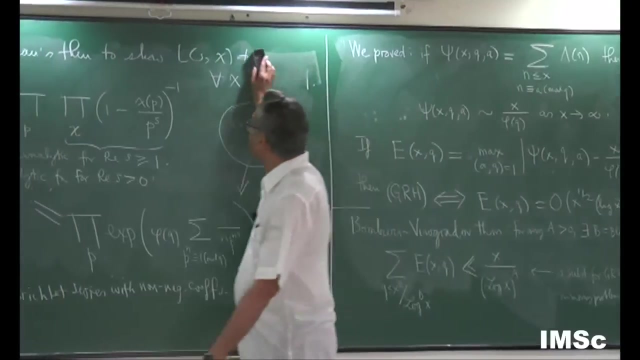 So this is not a actually, it's an interesting topic in itself, but you need the large sieve to prove this. Okay, And, as I said, error terms. if you want to do error terms, you need to have at least different techniques. 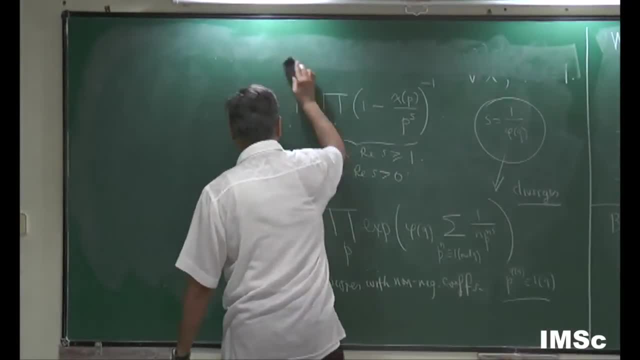 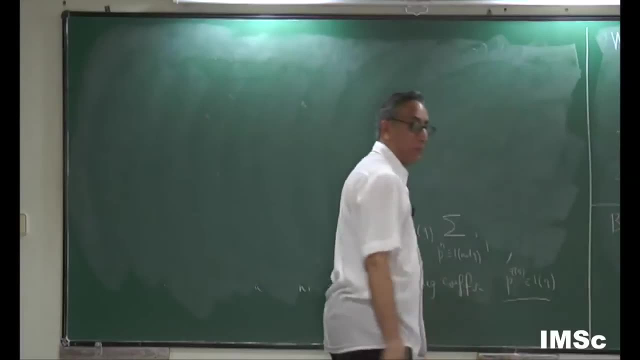 So the Tauberian theorem is too general and it doesn't provide error terms. although there have been people who have researched into trying to deduce error terms from the Tauberian theorem, They're not very good error terms, but people have done this. 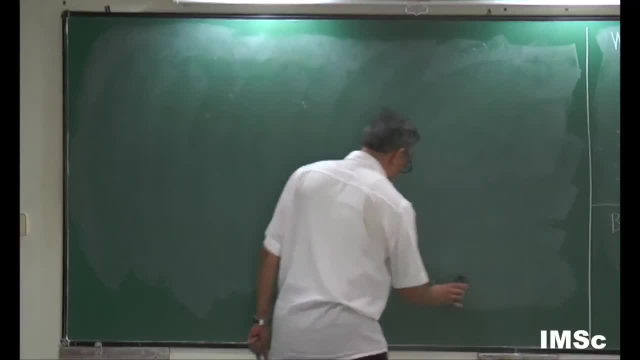 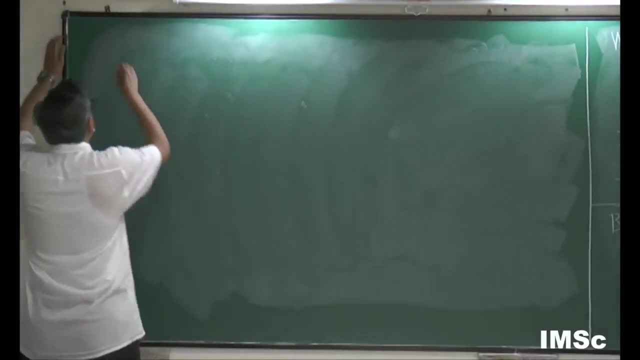 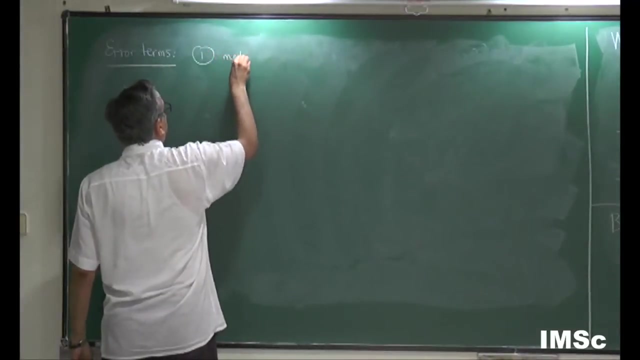 Perhaps it's basically of theoretical interest. They're not very good error terms because in such generality you can't expect to get such good error terms. There are lots of ways of getting error terms. One is the method of contour integration. 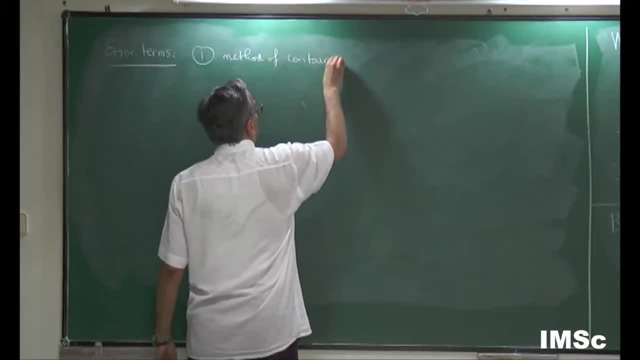 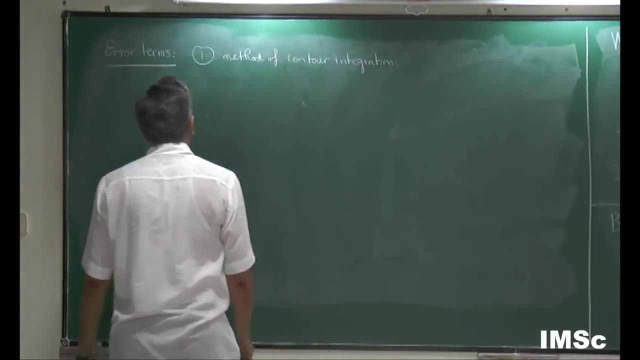 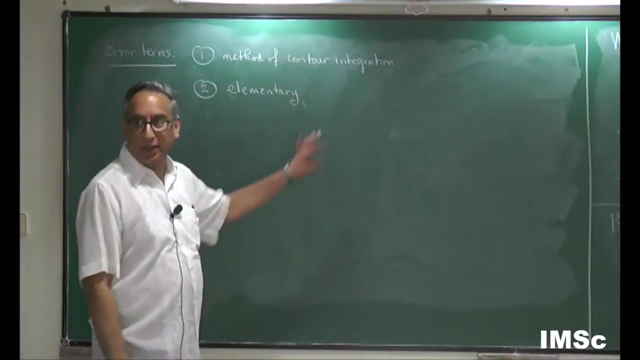 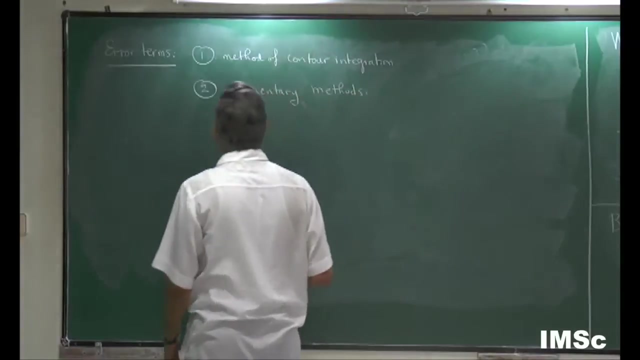 And Andthe second method is elementary methods. I mean, I told you, elementary doesn't mean easy, So let me say a few words about these two aspects. 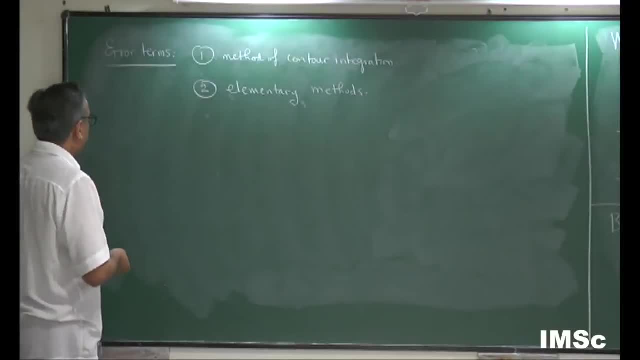 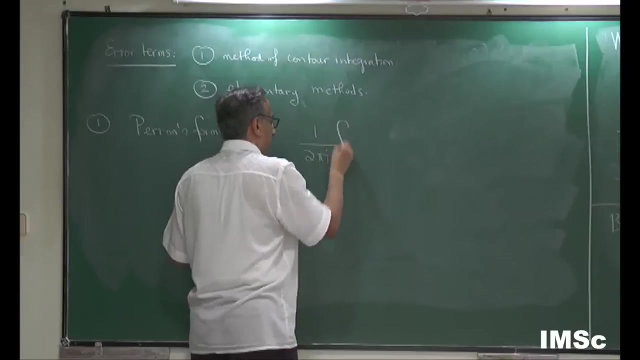 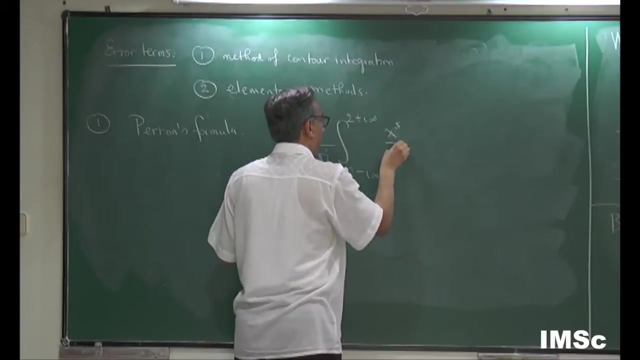 Let me talk about the method of contour integration. A key point is that you use what's called Perron's formula, Which is the following: If you take this vertical line integral. So here you are in the complex plane. 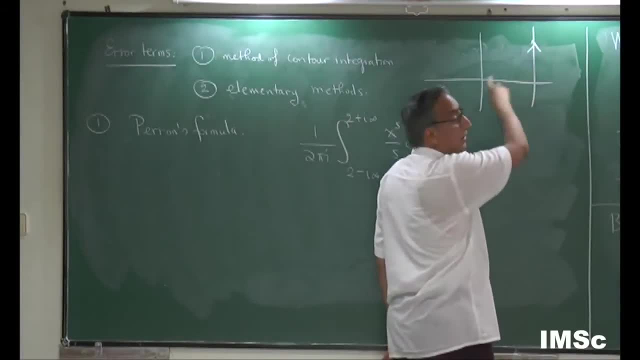 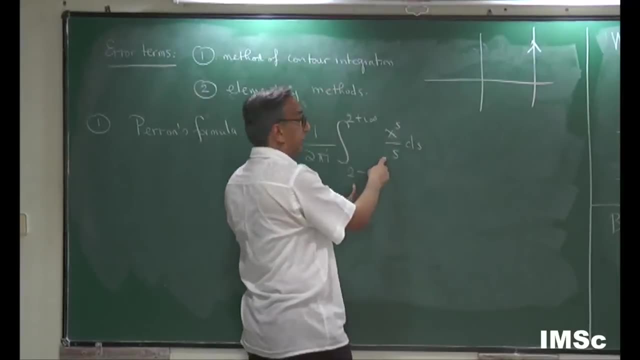 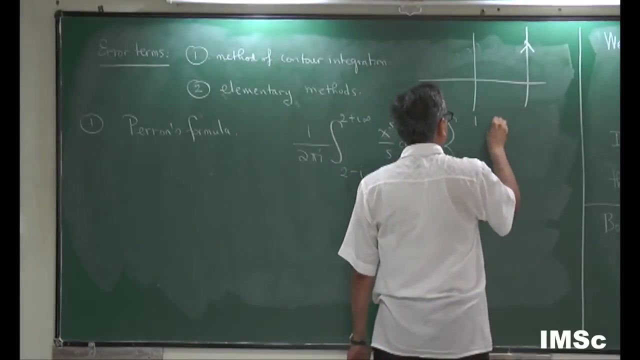 And I'm just integrating it from minus infinity to infinity Instead of from minus infinity to infinity in the real world. You kind of integrate it along the vertical line, This particular function, And the idea is that this is equal to 1.. If x is: 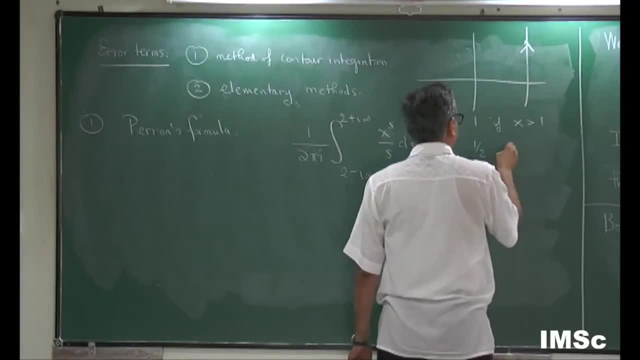 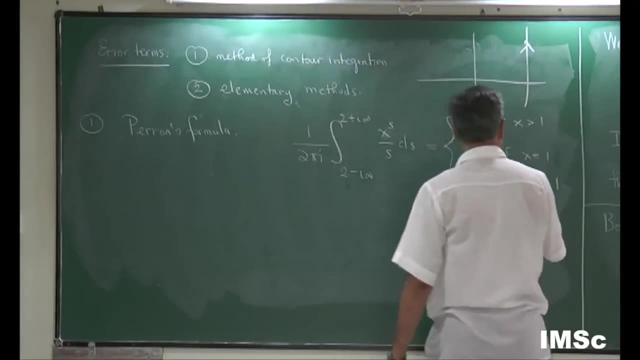 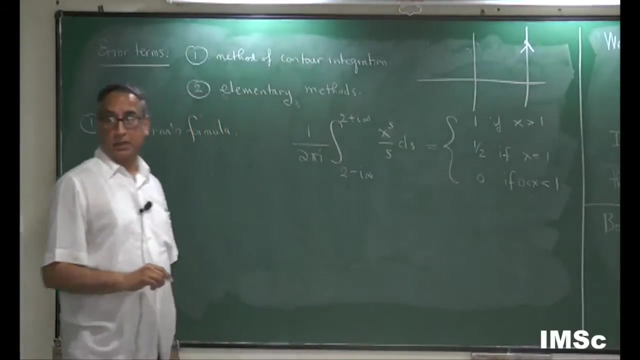 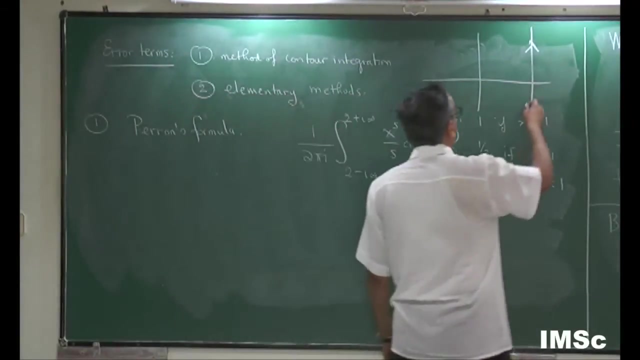 Bigger than 1.. 1, half if x equals 1. And 0 if x is less than 1.. So it's a simple exercise in contour integration. You can, So what you do is you. There's a singularity here. 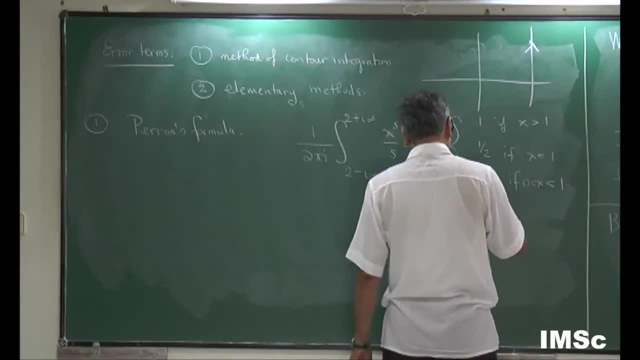 I'll leave this as an exercise. See: Singularity to x equals 0. So it's like a line integral. Perron discovered this. Now, what's so great about this? Well, it's Here's the reason. If I have a Dirichlet series. 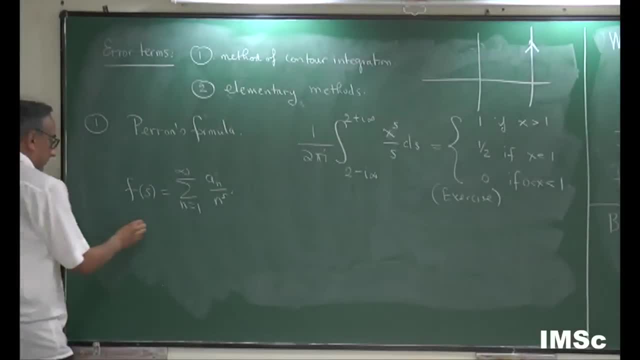 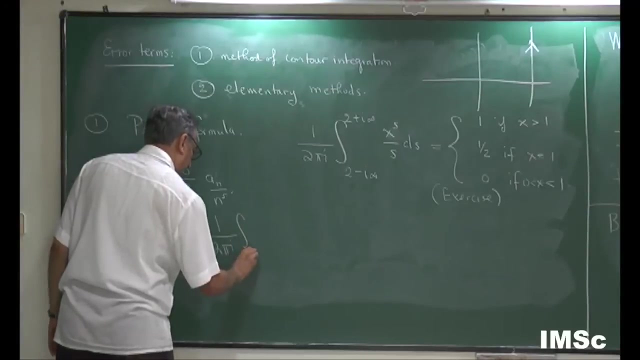 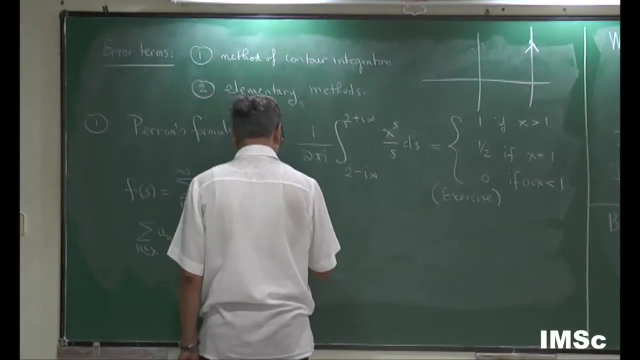 Like so, And I really want to Get Asymptotics for this, Which is what we were trying to do before. Well, There's a nice way to write that, And that is: And that is x As first. 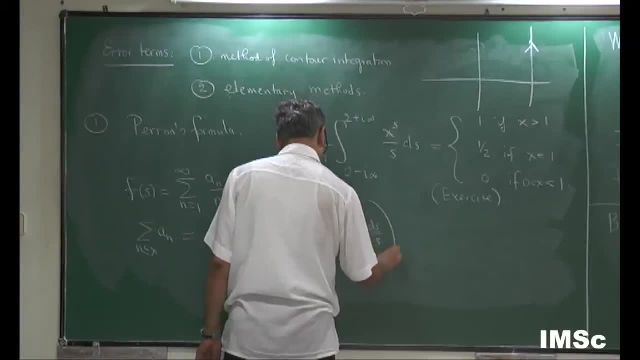 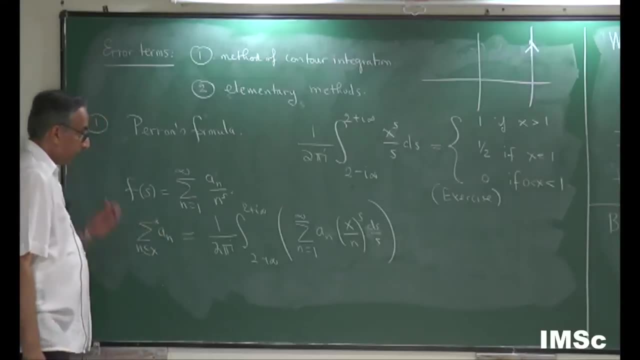 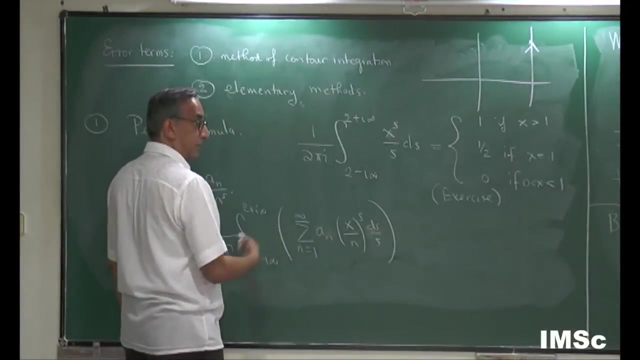 Where, of course, we should take the following understanding: So notice that this thing, if the Dirichlet series, let's say, converges absolutely for real part of S bigger than 1, so I'm in the region, here, I'm real- S equals 2, therefore this thing converges absolutely. 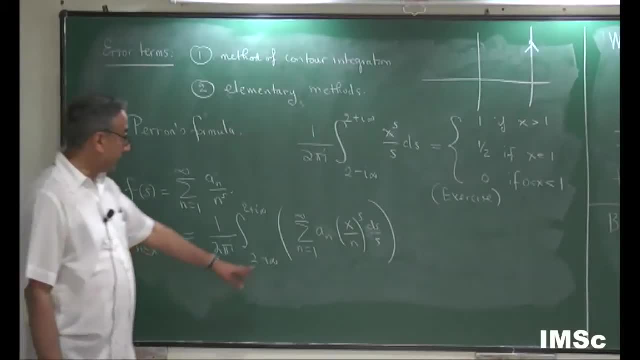 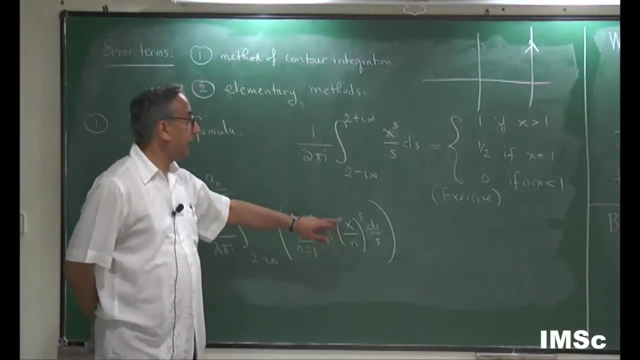 I can interchange the integration and the summation and you can see now that this is going to be summation: a sub n times this Perron integral x over n, which is going to spit out a 1 when x over n is bigger than 1,. 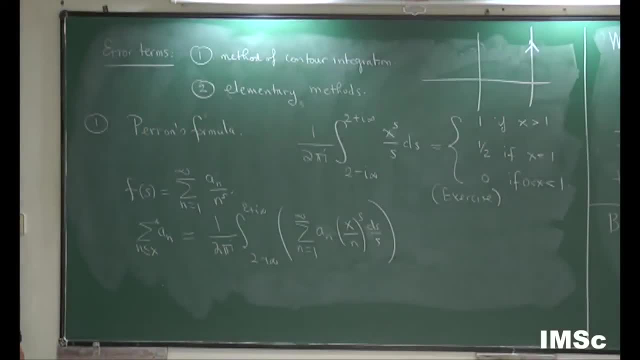 which is exactly the range I need it in. That means n is less than x, And it'll spit out a half when x equals 1, that's why I put the star there. So when x is an integer, it's not going to pick out a n, it's going to pick out a. 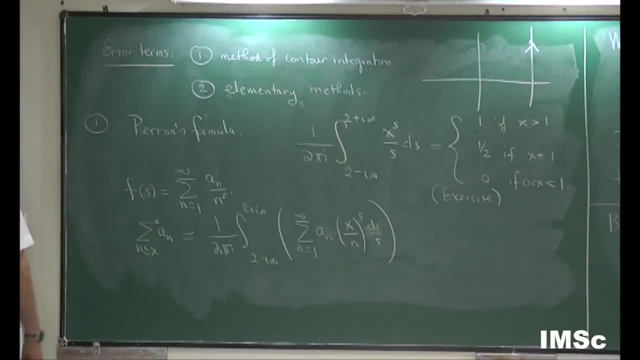 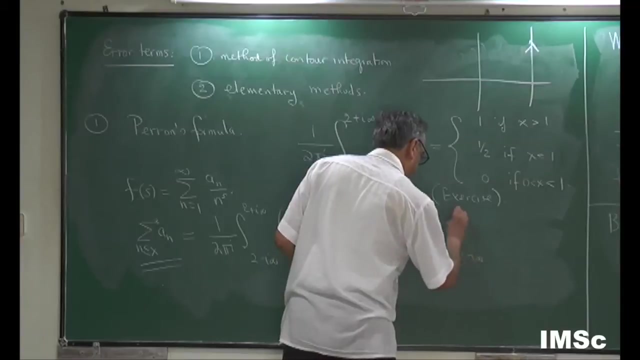 It's going to pick out a n over 2, so it's a small, but that's a minor issue. So here I've expressed the sum that I'm interested in as some sort of complex line integral which is 1 over 2 pi i right. 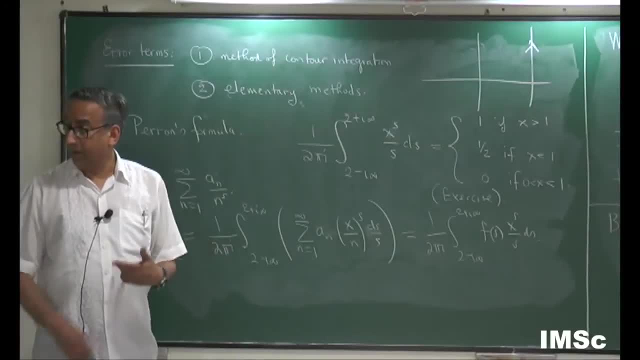 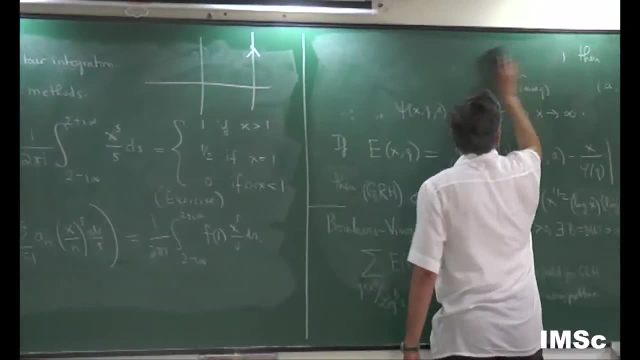 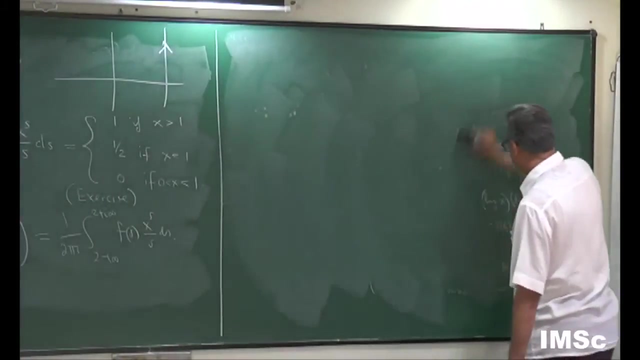 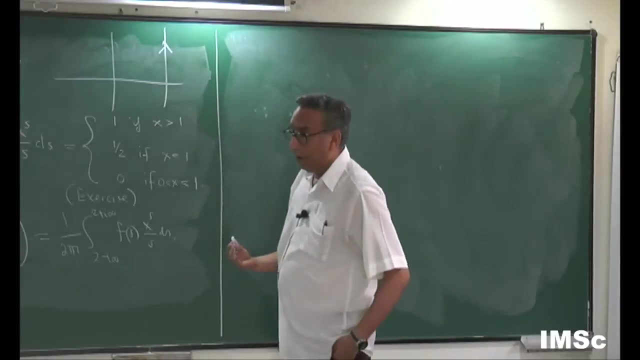 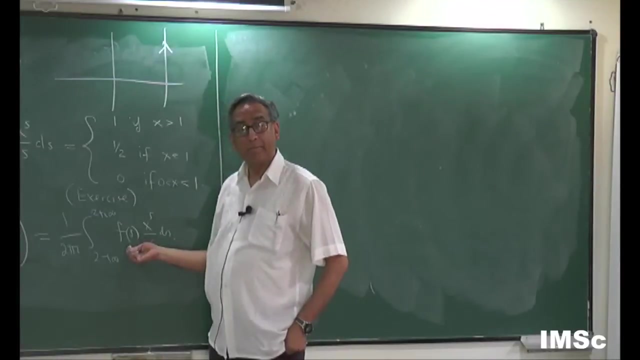 And the Dirichlet series F of S makes sense for real part of S, let's say bigger than 1.. Now here's where the power of complex analysis comes in, Supposing F of S admits an analytic continuation to a larger region. 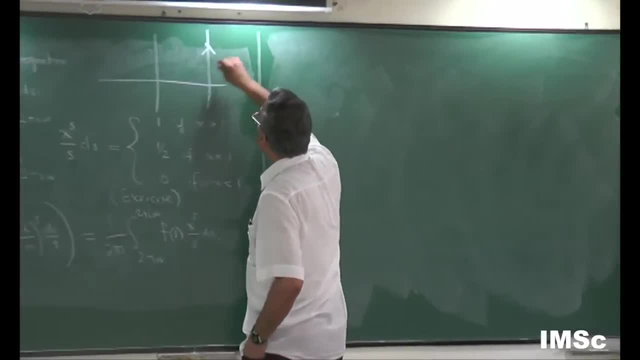 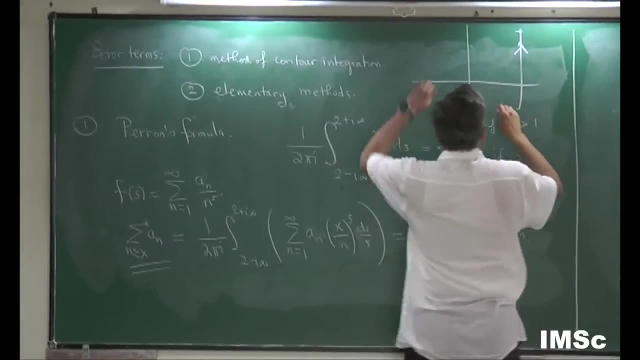 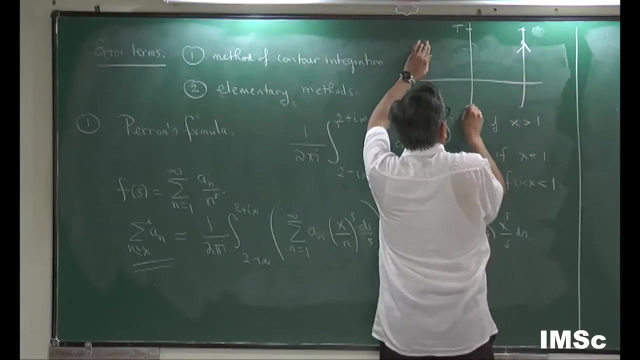 then I can now repeat, I can now replace this contour, so I can first start by truncating this thing. So there's a truncated version of the Perron formula which you have to use. Let's say you truncate it at some height- t minus t. 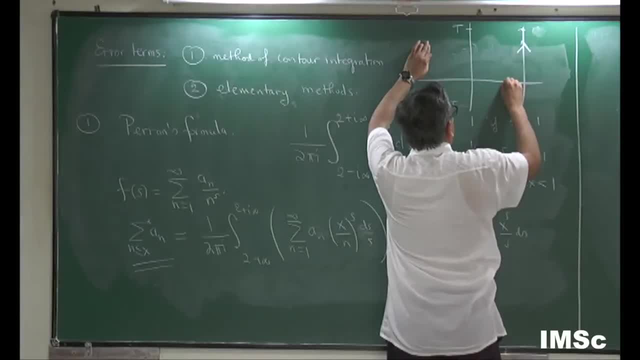 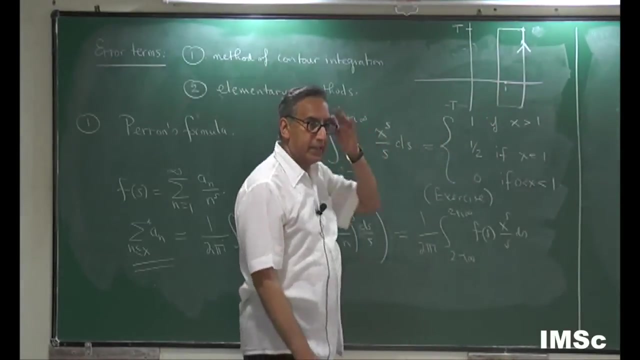 And you can, let's say at S equals 1, it's got a simple pole, so you would kind of deform the contour and replace this so thinking of this integral here from minus infinity to infinity as a limit, from minus t to capital T. 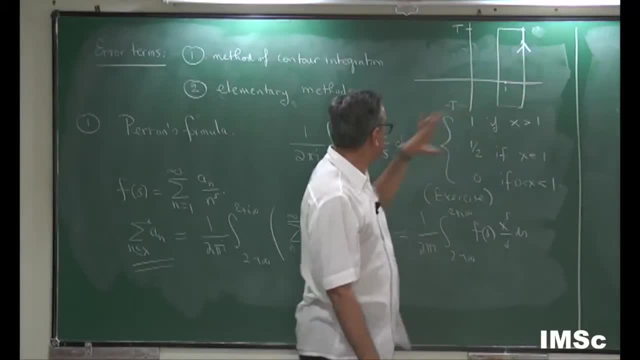 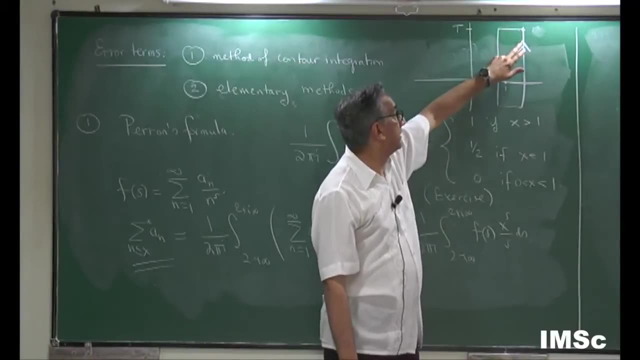 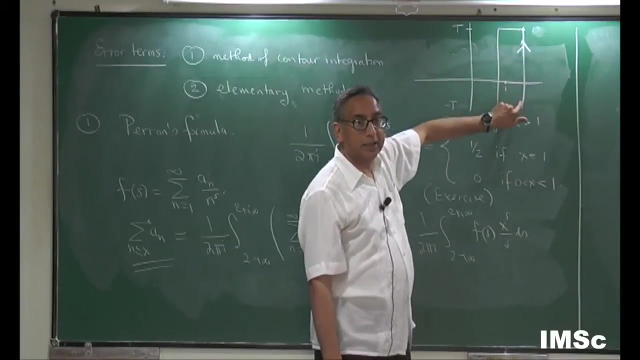 thinking of it like that: okay, We're replacing this vertical line integral by this kind of segment, and then we'll use Cauchy's theorem to say that this integral, or this vertical line here, is equal to the sum of these other three integrals plus, and you pick up the residue. 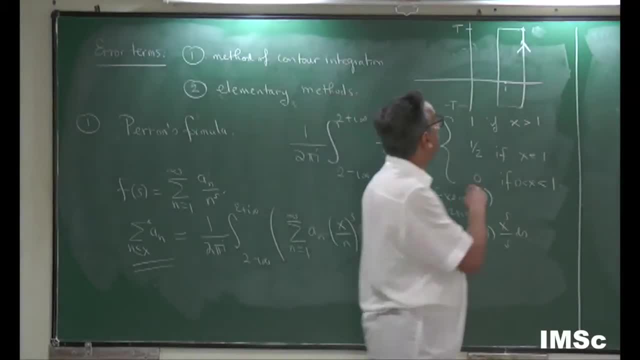 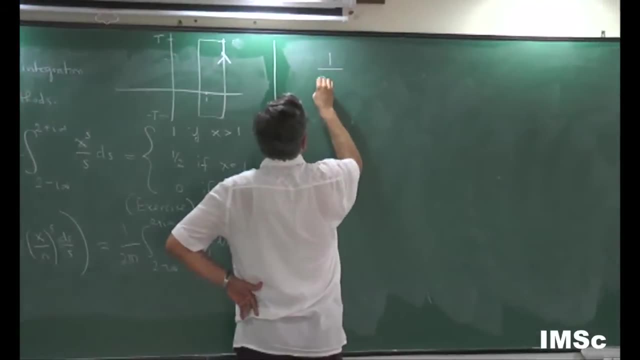 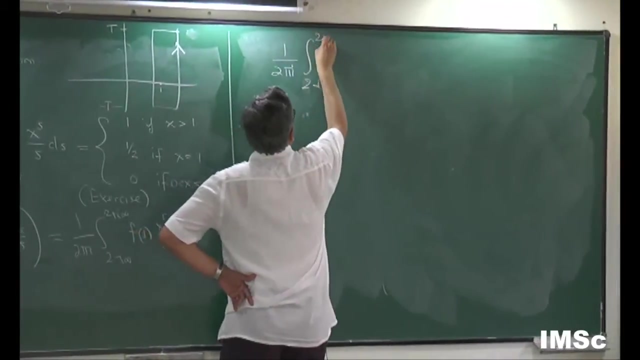 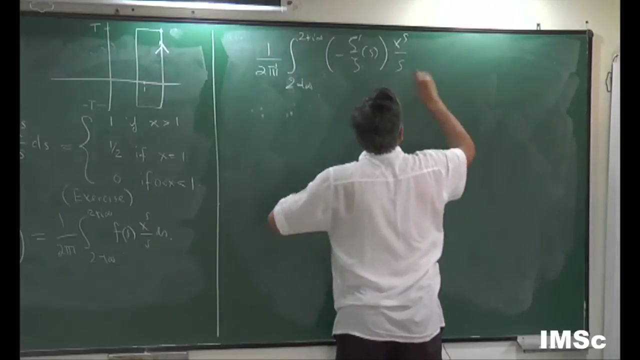 So the main term is going to come out from the residue, and this is exactly the calculation that Riemann did, without actually any of the theory. What he did was this: 2 pi i- Okay- Is equal to summation n less than x. 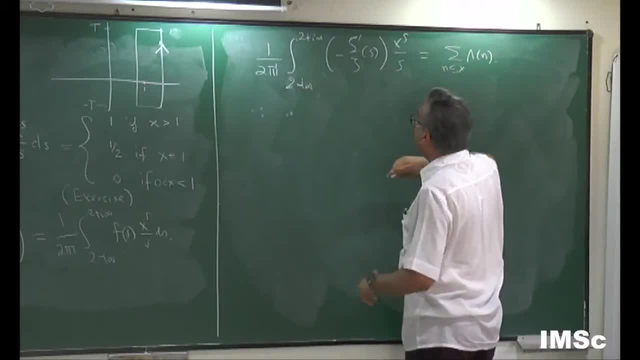 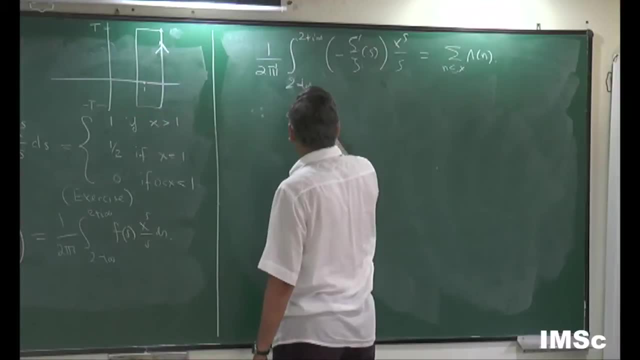 That's the formula. and then now you would you know that it has a simple pole at S equals 1, so he picks up the residue there, so that's x. And then now he has to worry about what are the other singularities. 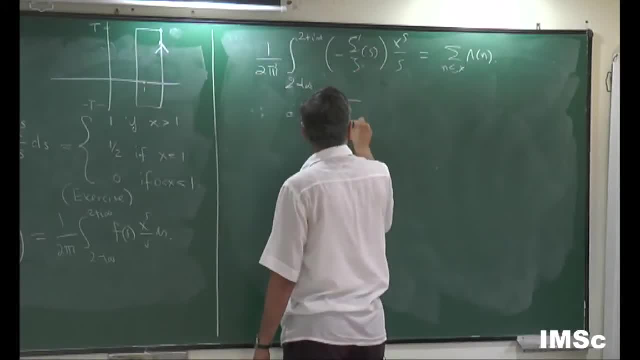 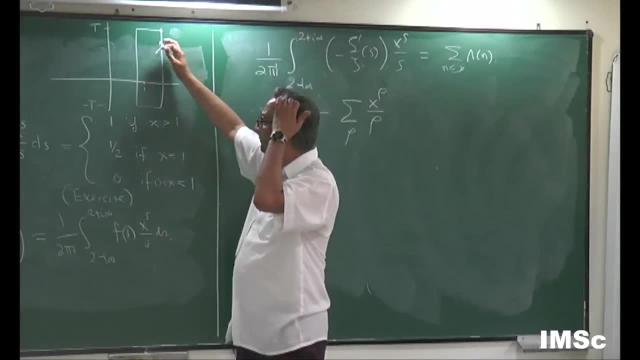 Well, the singularities will be coming from the zeros of the zeta function. so he writes down x to the rho over rho, for all the zeros, And then, at S equals 0, there's a, the contribution that's going to come. 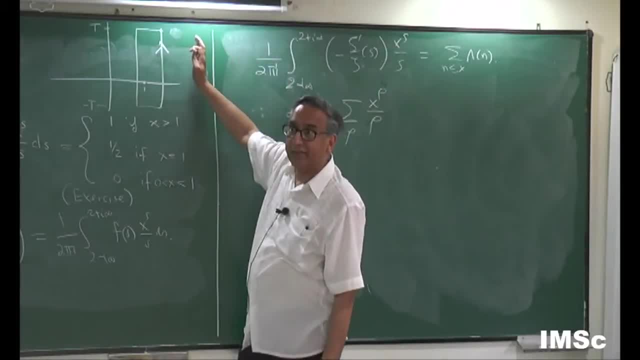 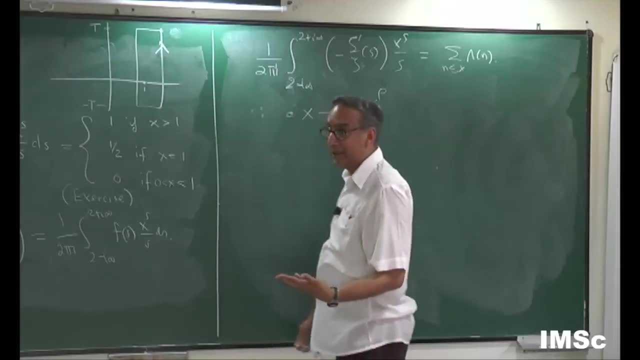 So the fact is that Riemann analytically continued the zeta function of the entire complex plane and that's how he was thinking about it. So he used that analytic continuation and realizes that I could go to the left as far as I want. 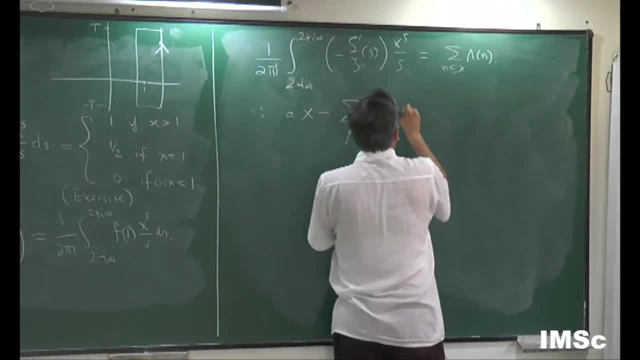 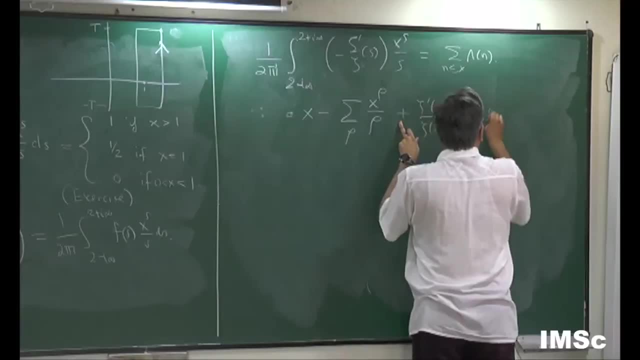 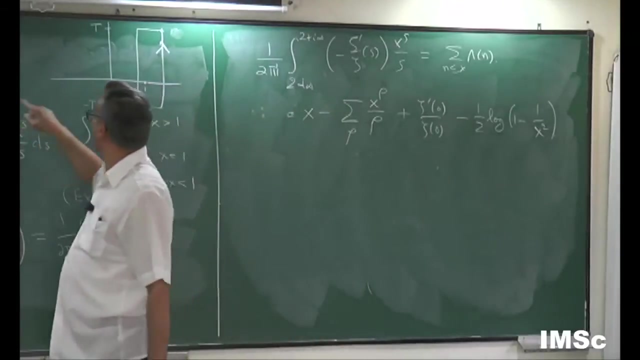 which he does. okay, And he ends up getting- now don't maybe I got these numbers wrong, but more or less 1 half log 1.. And I'm getting 1 over x squared, So he just keeps going. There's some, there's a, there's a singularity. a S equals zero. 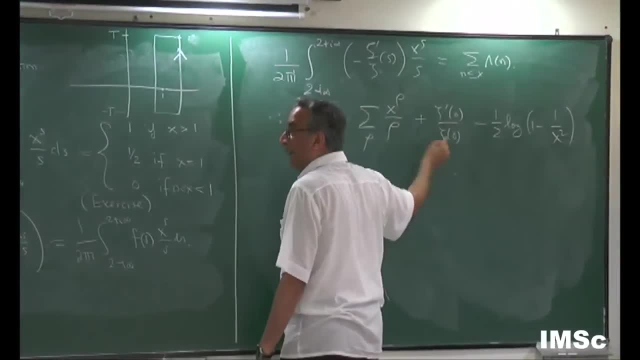 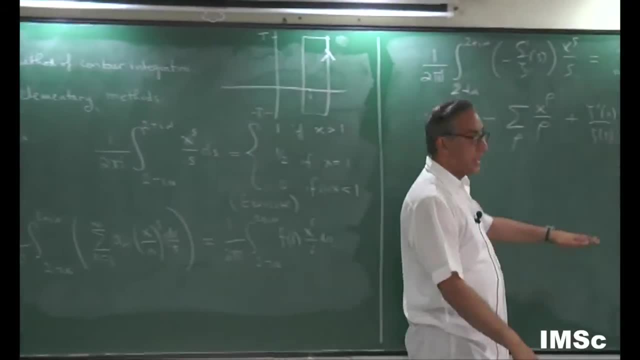 That's coming from here. So he picks up that residue and then he keeps going, and then there are trivial, so-called trivial zeros at negative, even integers, And so when he adds up all those contributions he ends up getting this, and he actually gets an explicit formula. 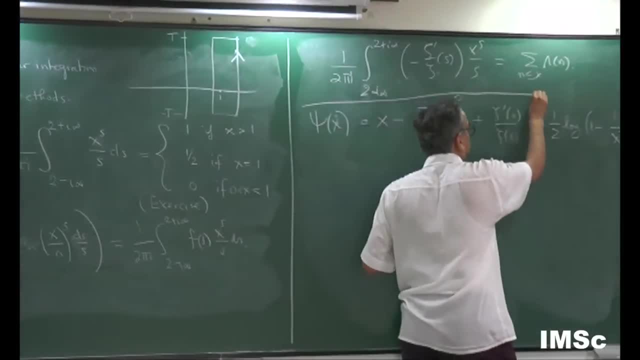 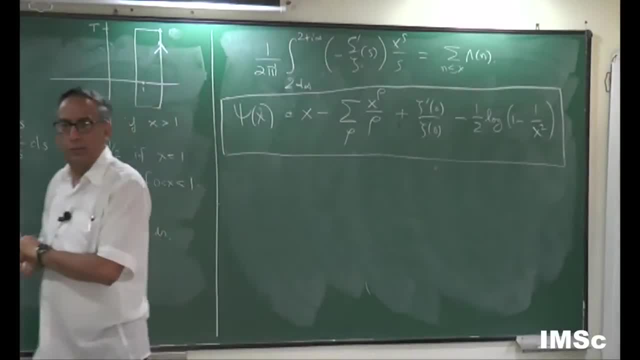 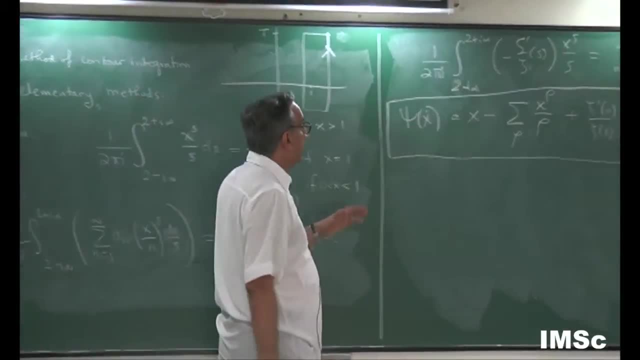 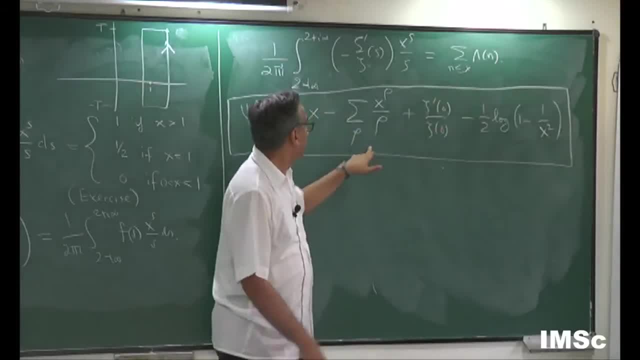 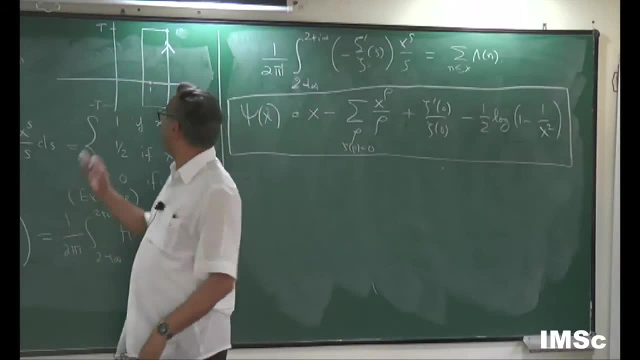 connection between prime numbers and these are the zeros of the zeta function in the critical region, so-called critical region. That means we showed there are no zeros to the right of one and one can show by the, by what's called a functional equation, that there are no. 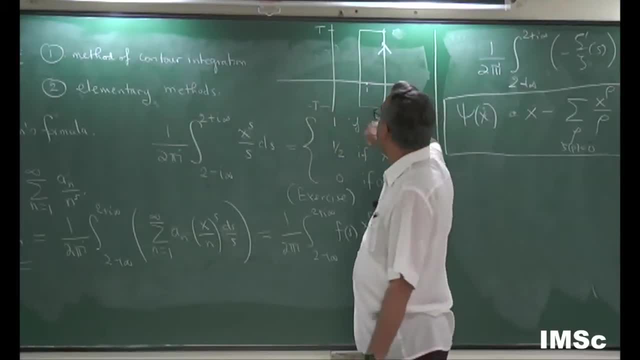 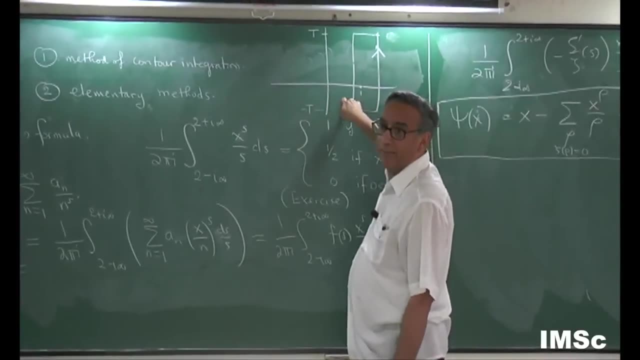 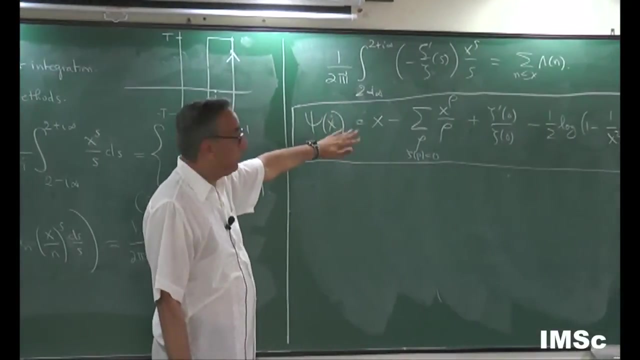 zeros to the left of one, except the trivial zeros, and once you have that, all the action is taking place between real part s equals zero and real part s equals one, and so those zeros give rise to that. So contour integration can actually show you this rigorously, but however, you need to know. 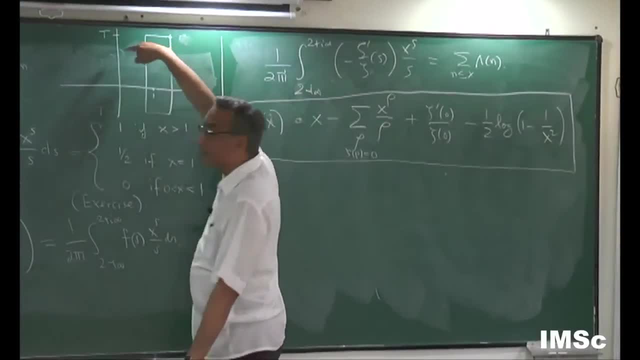 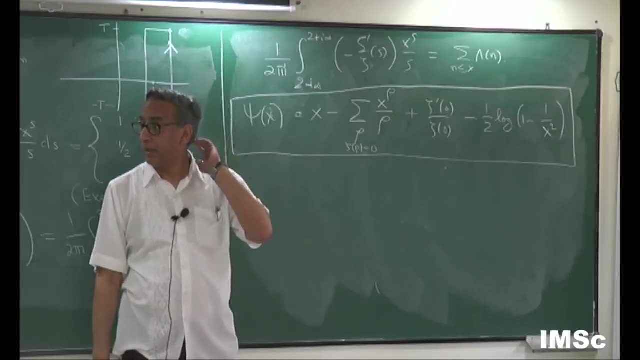 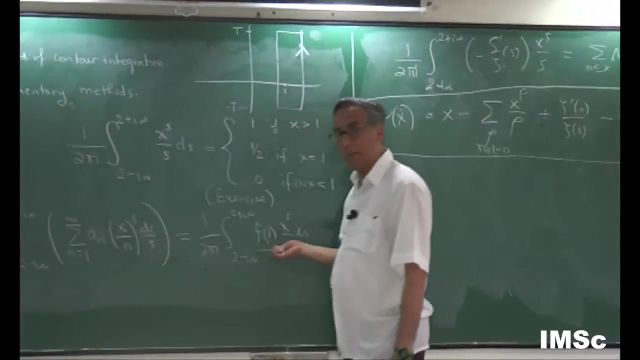 you need to estimate these things on the horizontal contour and justify these limit processes, and for that you need to study the zeta function more in a more detailed form. So this is the general method of contour integration using Perron's formula, using analytic properties deforming the 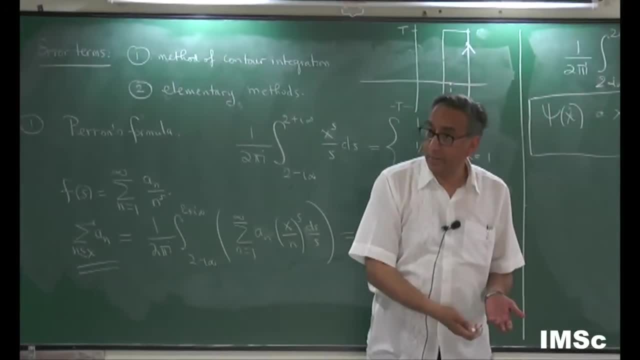 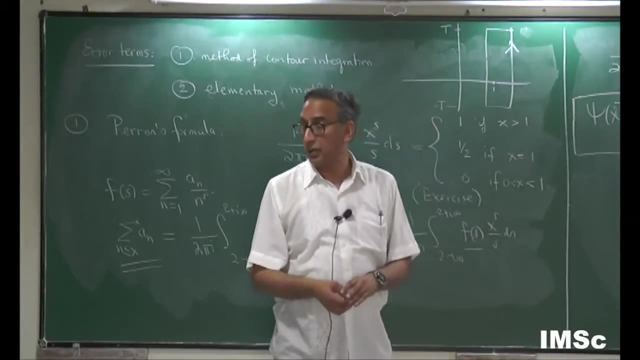 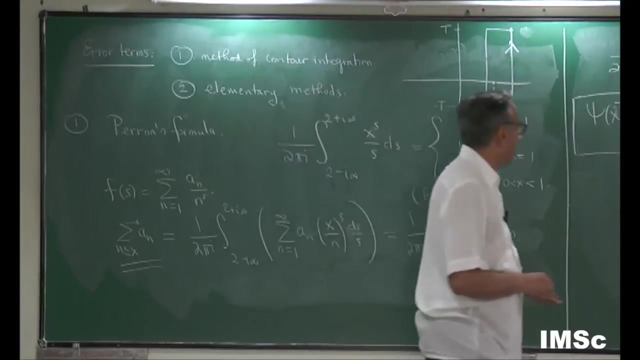 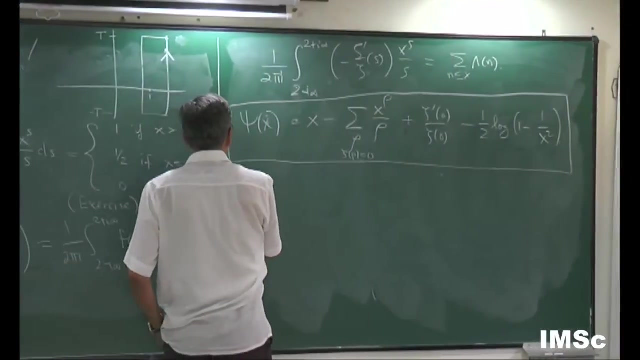 contour into the region where you pick up the singularities and then estimating the function on these other lines and then getting an error term. So that method of contour integration usually leads to very good error terms. That's the method of contour integration, okay. The second method is elementary methods. These are: 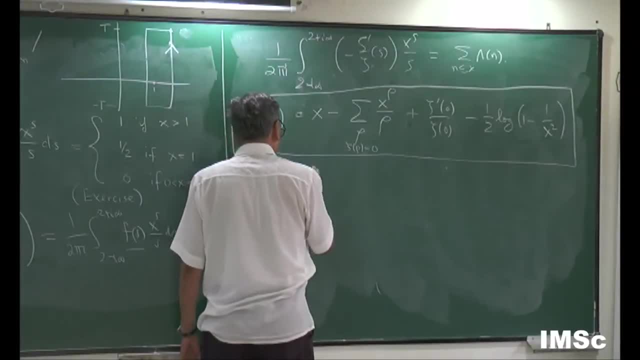 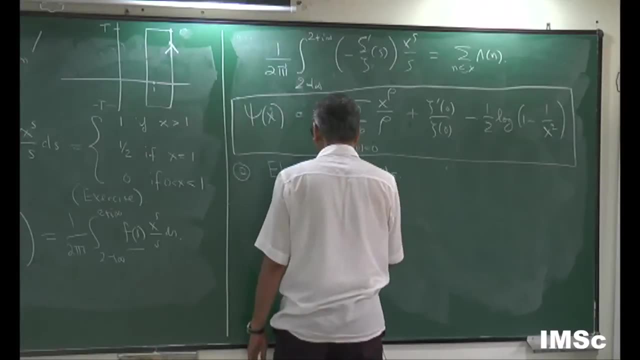 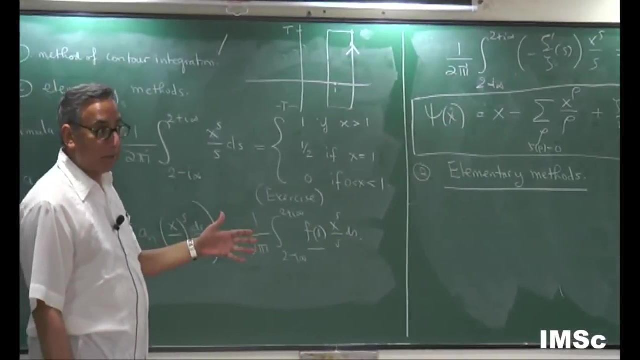 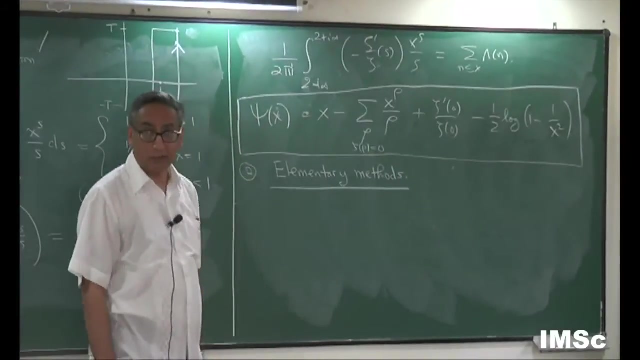 more difficult, of course, but sometimes not. These are just basically bare hands and estimations And so forth, and sometimes elementary methods may lead to better error terms. sometimes, For example, in the problem that I gave you as homework assignment that you asked about counting- 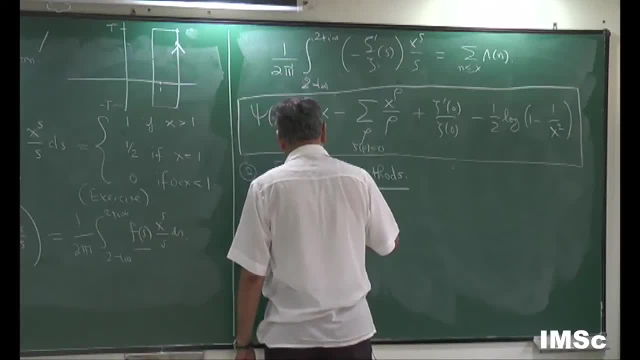 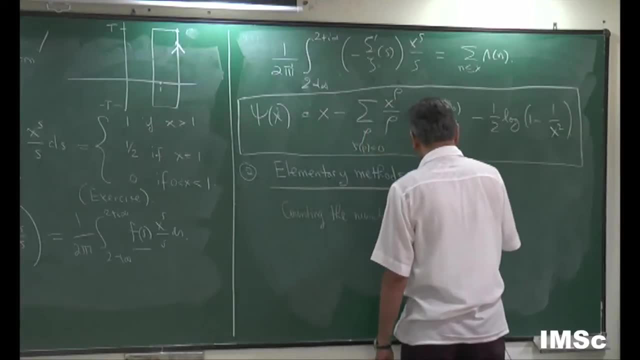 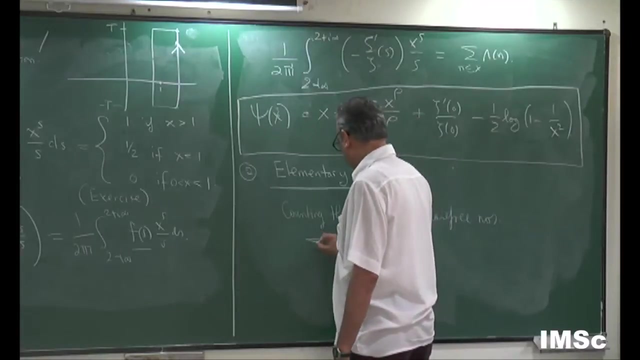 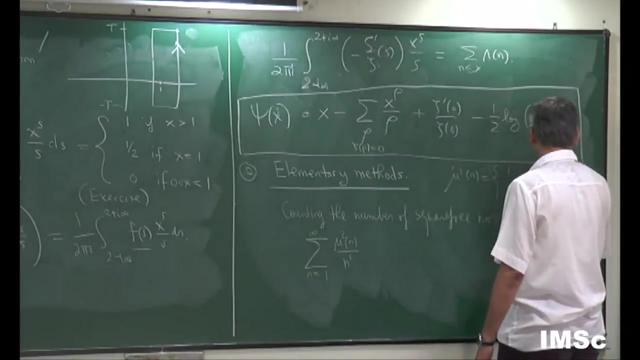 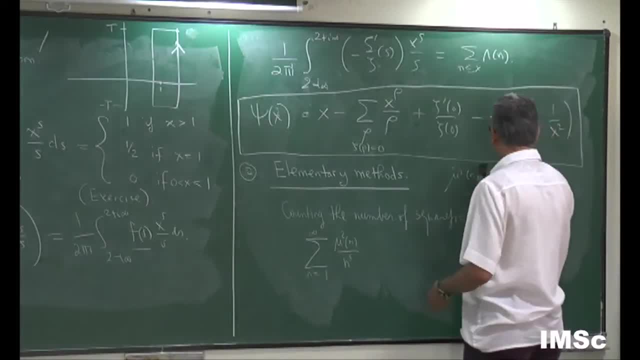 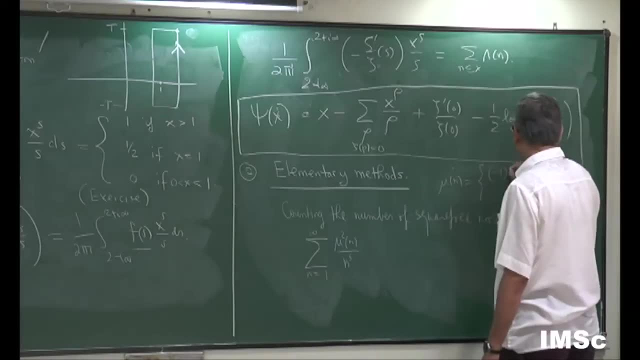 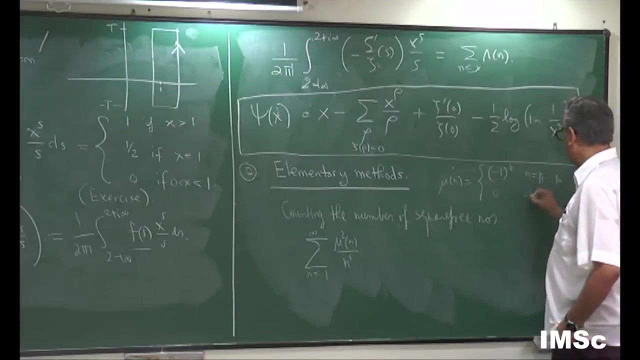 Yeah, why do we do that? Let's define mu of n. Let's define mu of n. Yes, sir. So b minus 1 to the power k if n is a product of distinct prime numbers and 0 otherwise. Okay, so this is a Mobius function. 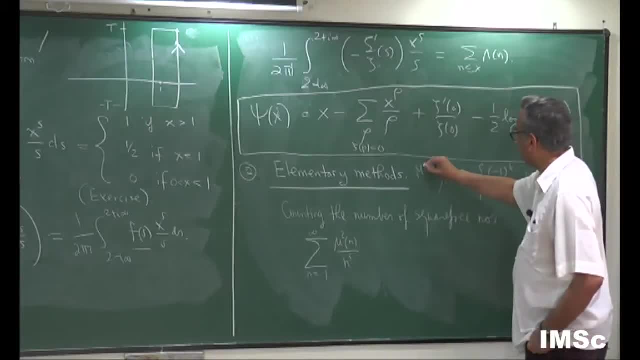 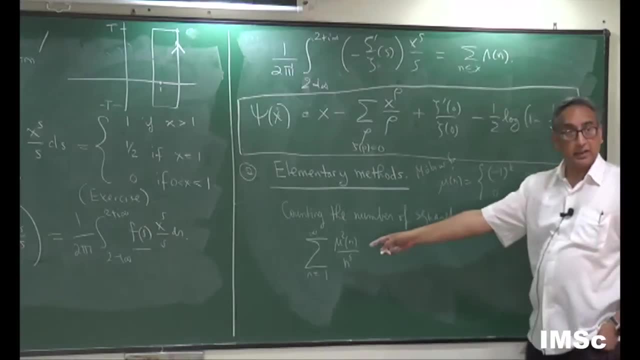 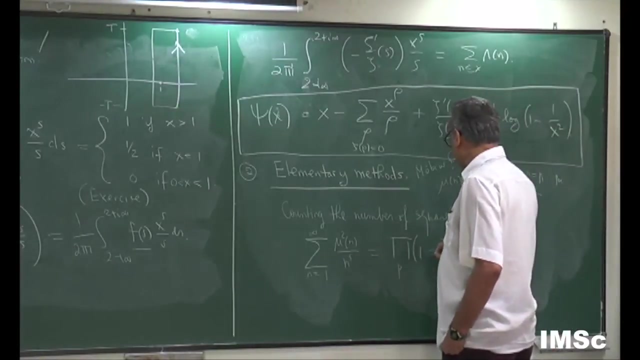 I think most of you probably have seen this already- Mobius function, So it's supported only on square free numbers. So if I square it I can use the characteristic function for square free numbers. And now it's a multiplicative function, so I can write this as 1 plus 1 over p to the s right. 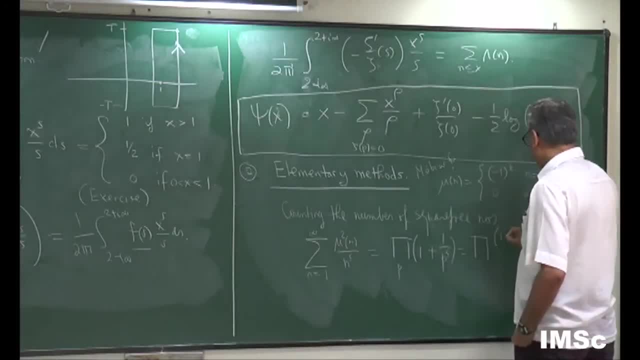 So that can be written as 1 minus 1 over p to the 2s over. 1 minus 1 over p to the s right. That's like so right. So this is zeta s divided by zeta 2s. 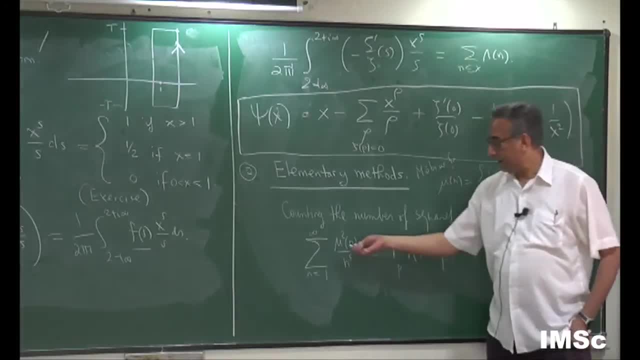 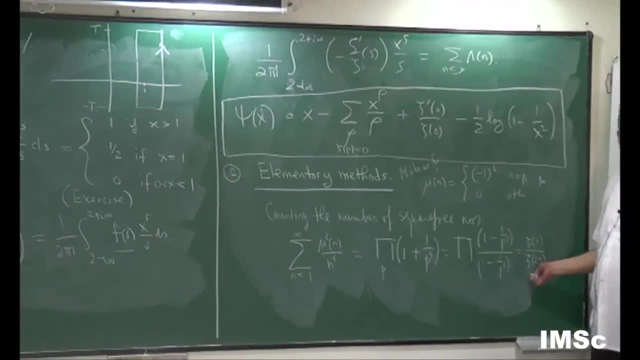 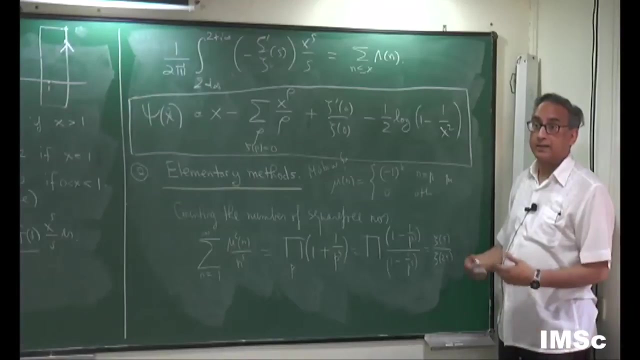 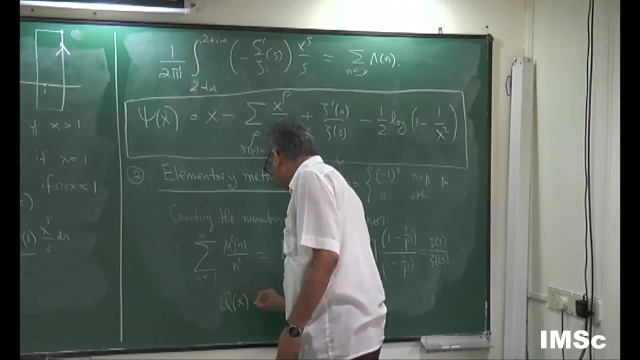 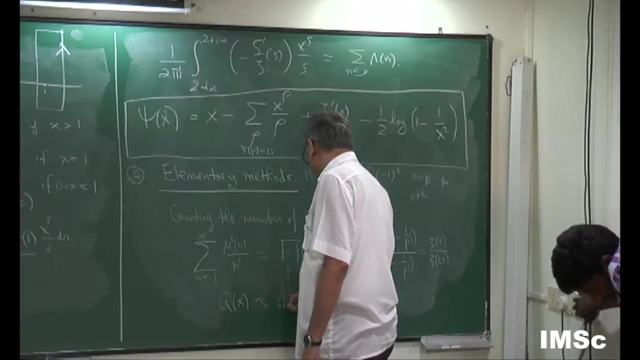 So. So, in other words, if I look at the Dirichlet series associated with the characteristic function of the square free numbers- I have a nice expression for it in terms of Riemann zeta. I have a nice expression for it in terms of the characteristic function of the square free numbers. 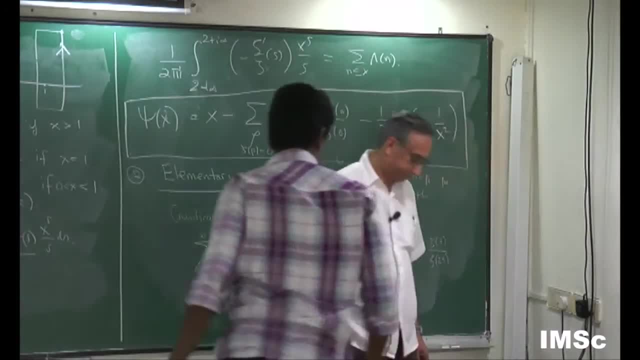 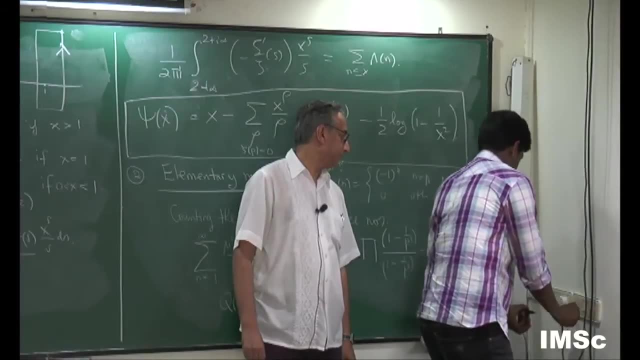 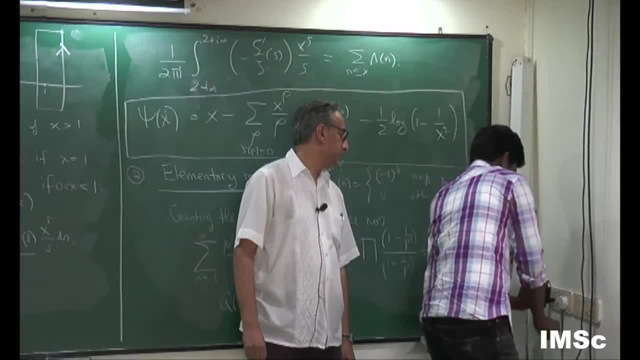 So, if I have some of these, the second set of endpoints is going to be x plus 2 over x plus 3 over x plus 2 over x plus 2 over x plus 2.. I could show you some here, Oh, okay. 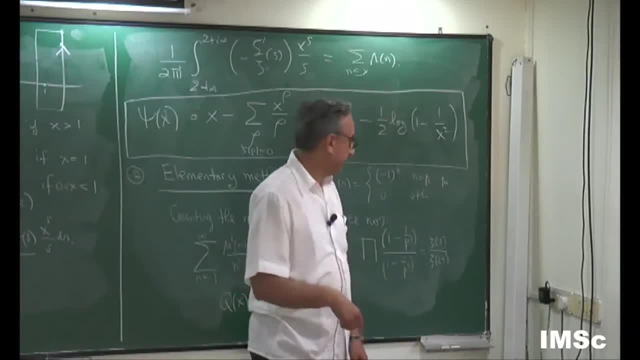 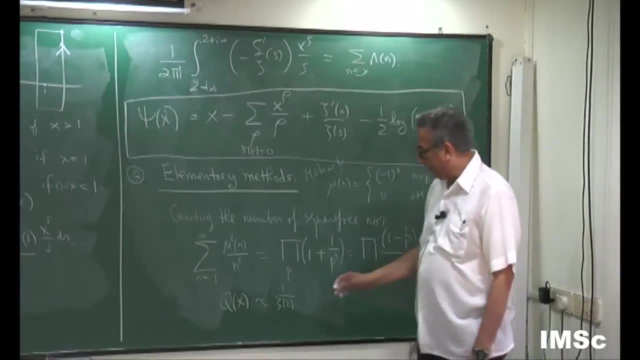 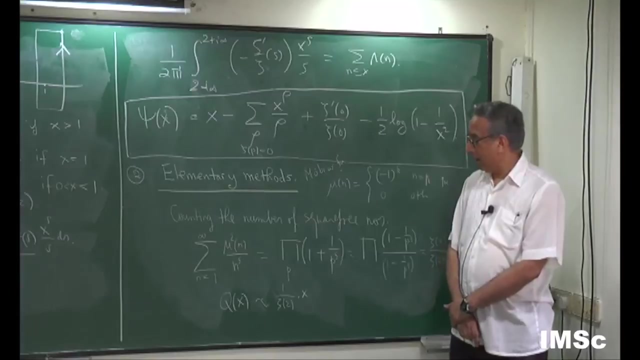 Okay, Was it working before? Okay, so you have a simple pole at s equals 1, residue 1 over zeta 2, so automatically, the Tauberian theorem tells you that this is asymptotic 2, because that's what it is right, However, you're. 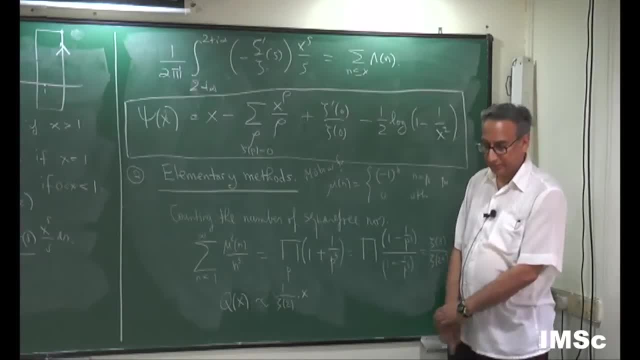 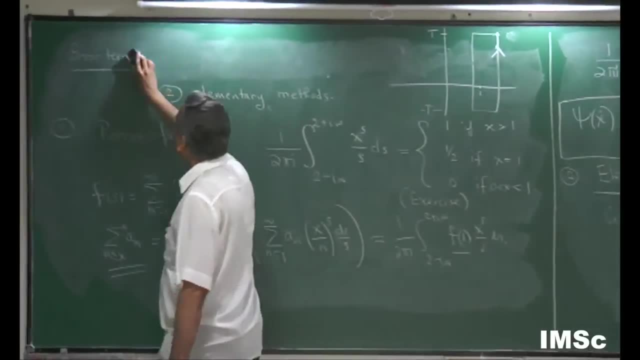 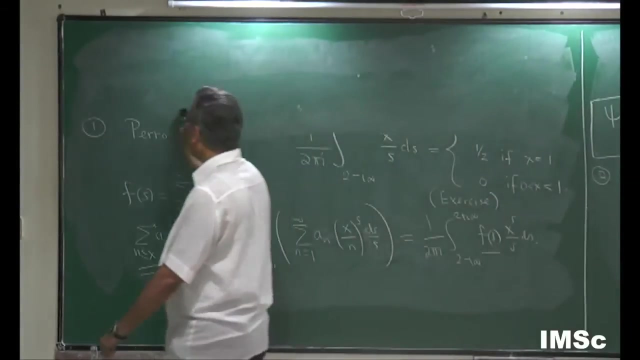 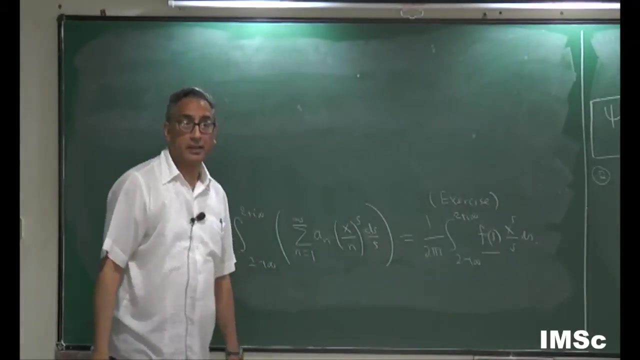 not going to get error terms this way, and if you want to get error terms, you can apply a more direct approach. The value of the Tauberian theorem is that it's extremely general. The elementary methods can exploit the special nature of the problem and get better, better error terms. 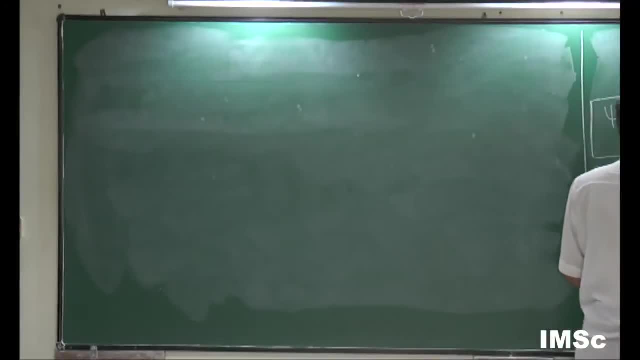 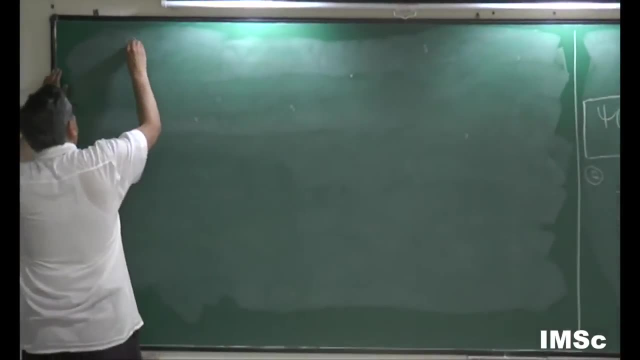 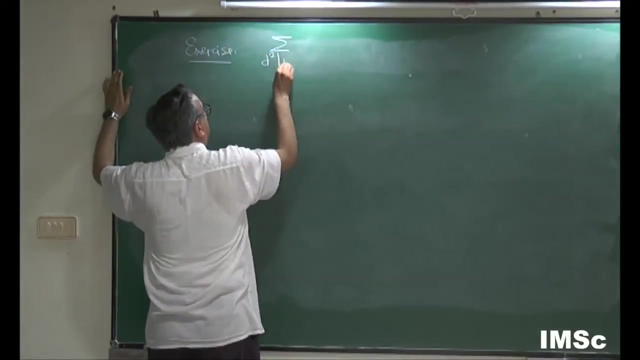 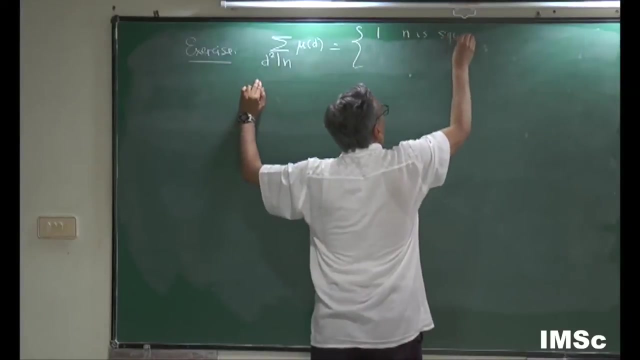 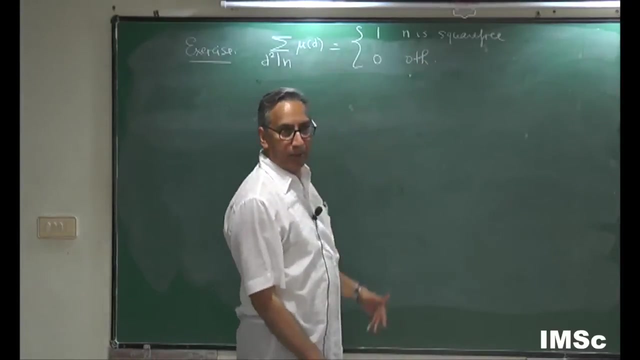 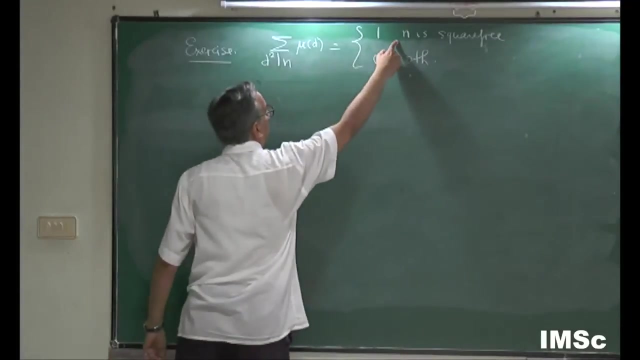 This is a particular case in point. So here, small exercise, Okay. so I'll let you try and prove that more or less It's there, but I'll prove it, okay. So if that's the case, this is the characteristic function of the 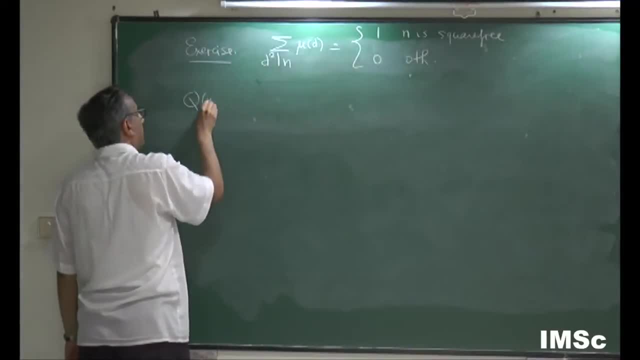 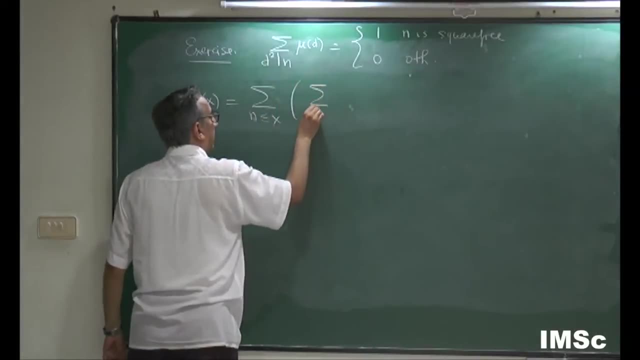 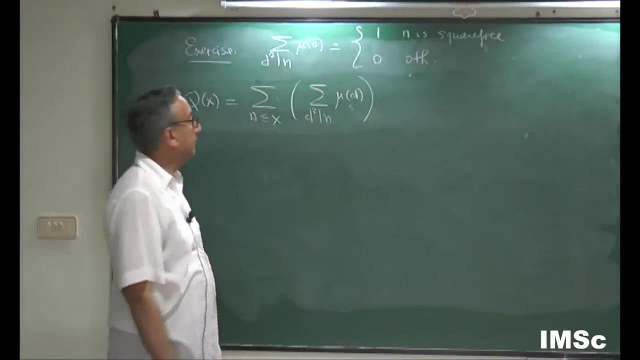 square-free numbers, then Q of X is just simply n less than x. d squared divides n mu d, right? I mean, that's what you have, Plug it in, right? And now you do, obviously, the interchange of summation: d squared less than x mu d. 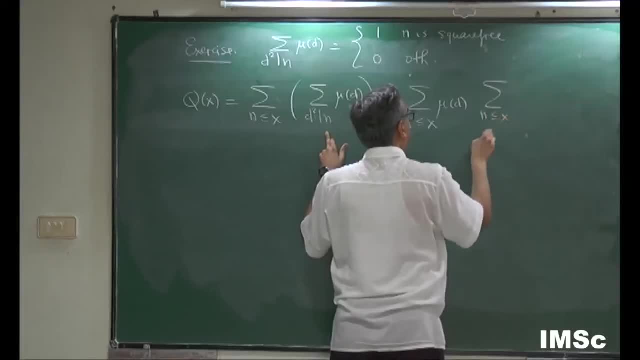 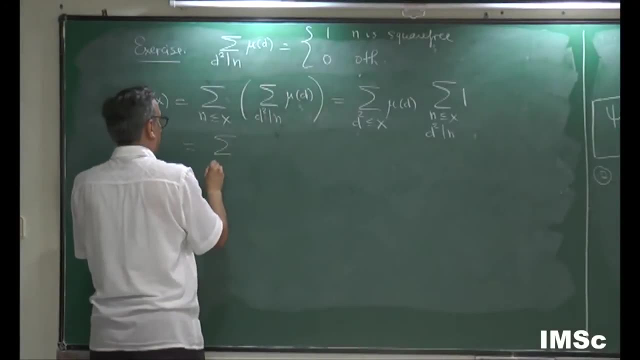 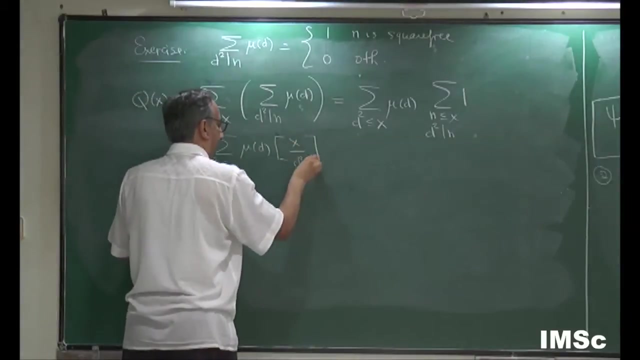 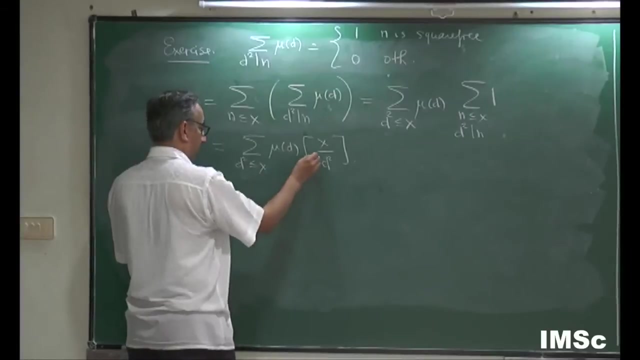 inside you have to count n. less than x d squared divides n One, So this becomes d squared less than x, mu of d x over d squared. And now you can see that I can remove the square brackets here. d squared less than x, mu of d x over d squared. okay, 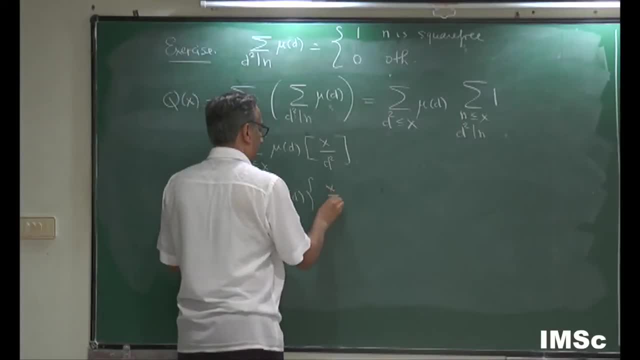 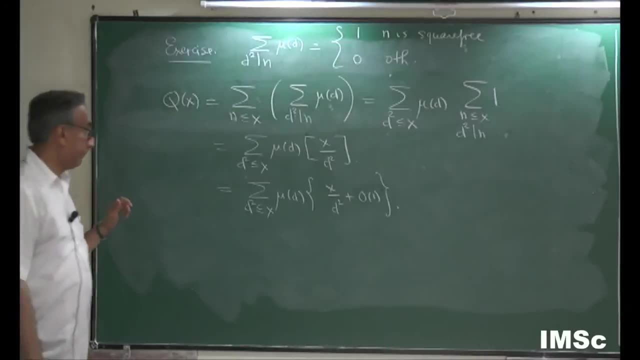 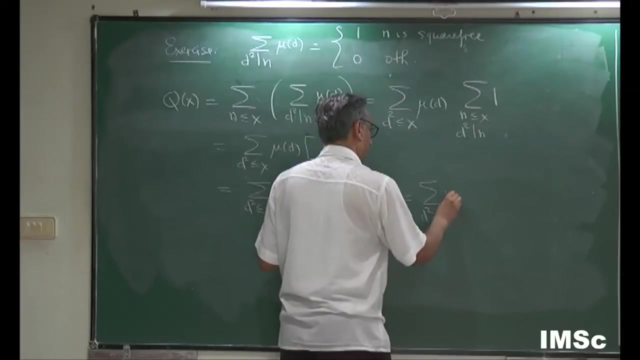 x over d squared plus o of 1, and now you get d squared less than x, mu d. well, x comes outside mu d over d squared plus o of well. the Mobius function is at most 1 and I've got at most root x sum n. 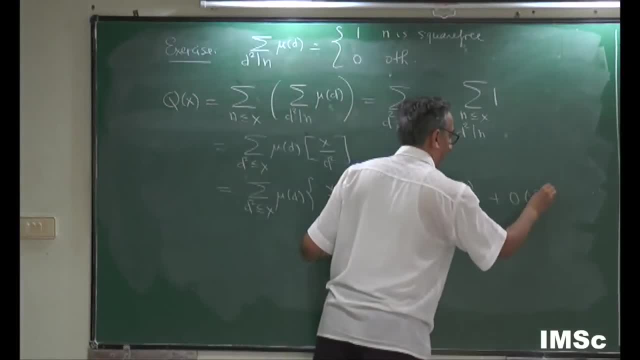 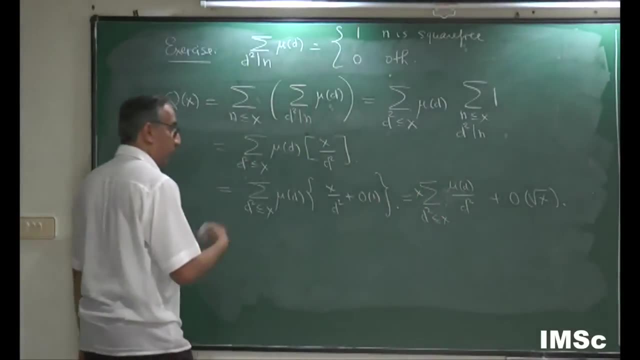 so it's o of root x and this is a convergent series. so don't replace that by 1 plus little o of 1, then you'll get back your Tauberian business and that's not a very good error term right. So what you should do 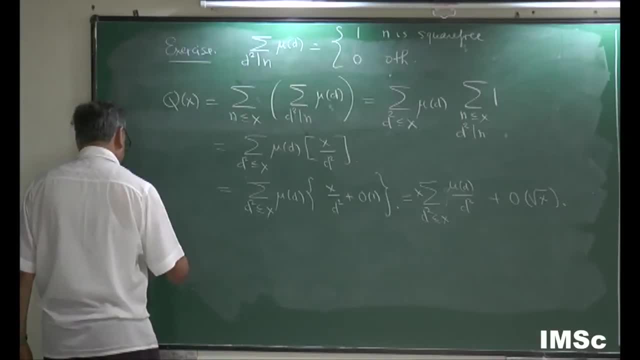 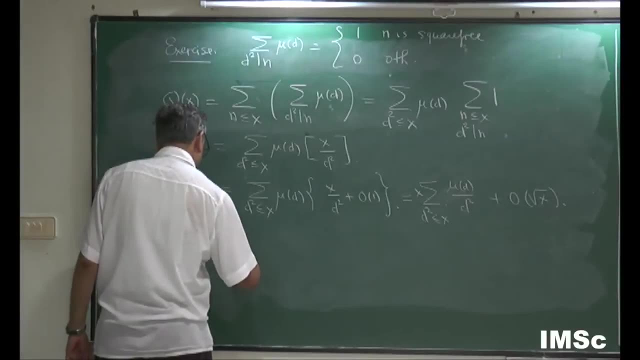 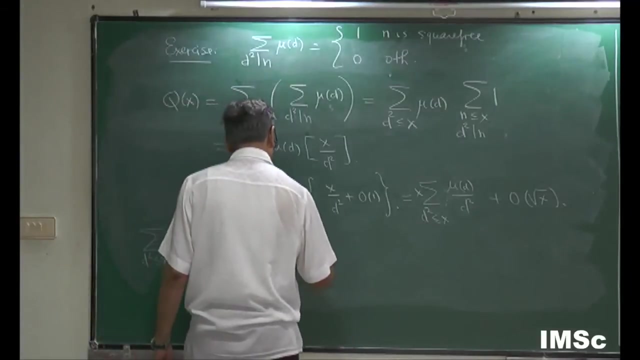 is, you should say, d squared less than x. mu d over d squared is the full series d going from 1 to infinity. mu of d over d squared minus d squared bigger than x. in other words, d is bigger than root x. mu d over d squared right. 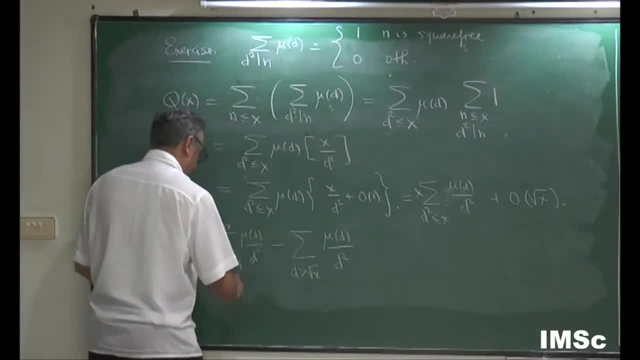 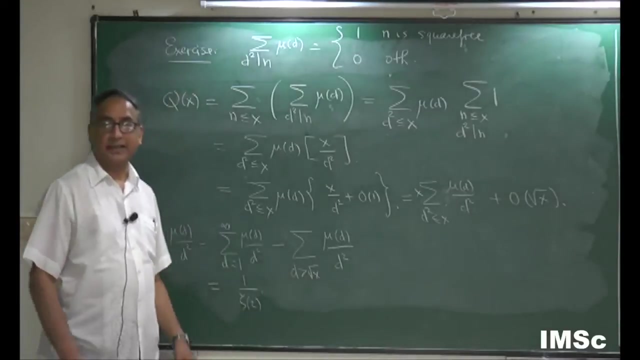 And now you can see that this is a constant which we will write as 1 over zeta, 2 right, And then this: you just put absolute values on the Mobius function, so it's summation 1 over d squared. it's a tail of the. 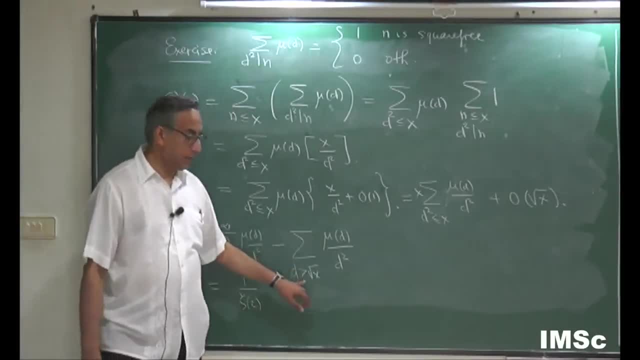 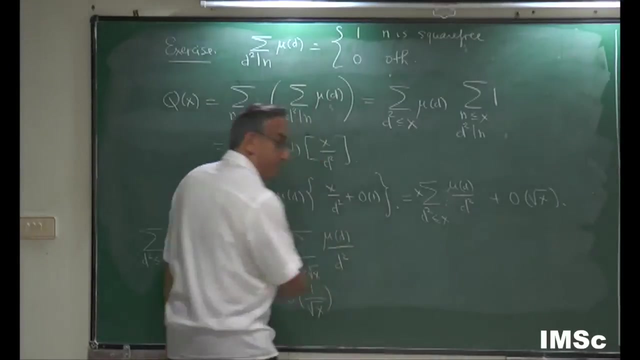 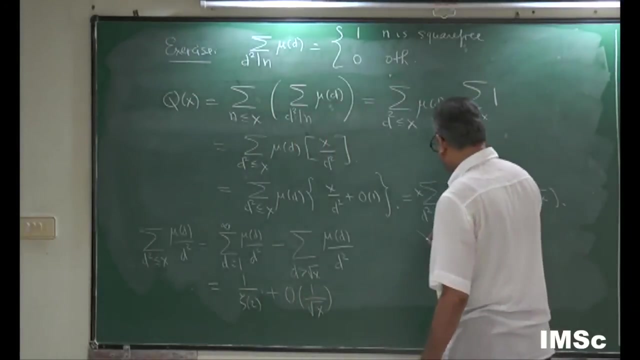 convergent series. the tail can be estimated by the integral dt over t, squared, going from root x to infinity, and when you do that, it's all 1 over root x, right, Okay? And so I go back here and plug it in. and so what do you finally get? 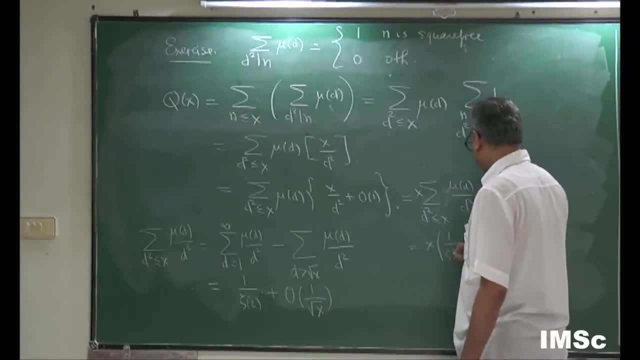 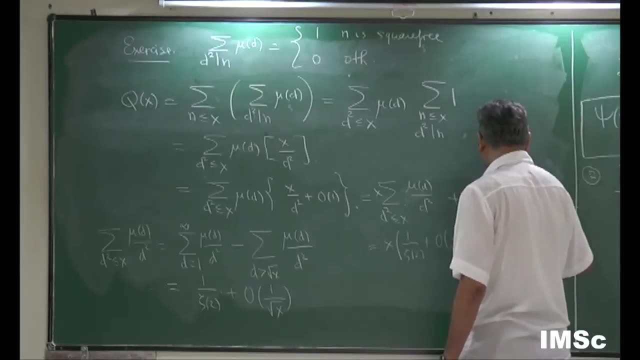 You get x times 1 over zeta 2 plus O of 1 over root x plus O of root x, and so this is x over zeta 2 plus O of root x. so you get this very good error term square root of the main term. 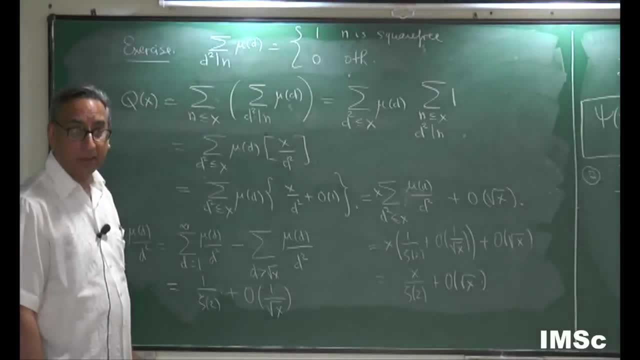 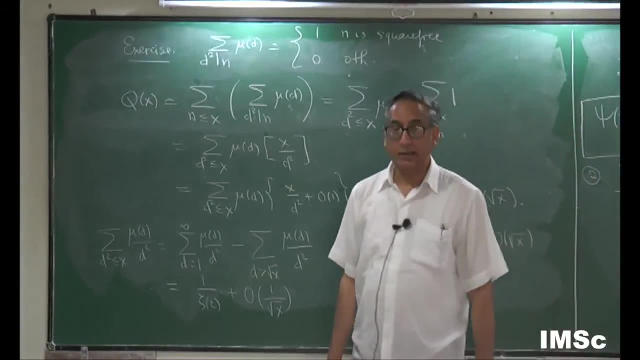 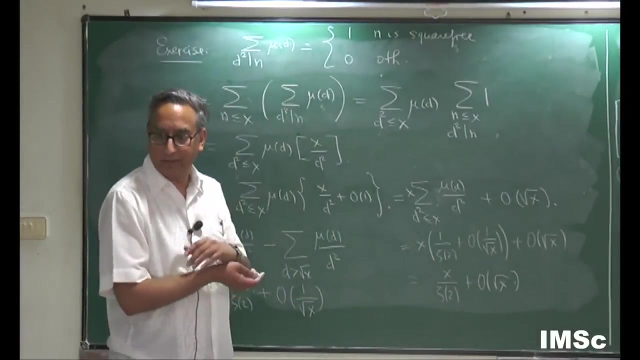 by an elementary method, without any complex analysis. the complex analysis method gave you just the first term but doesn't give you anything else. but that's a more powerful theorem, very general, too general, that it's not going to give you error terms. but if you want to get error, 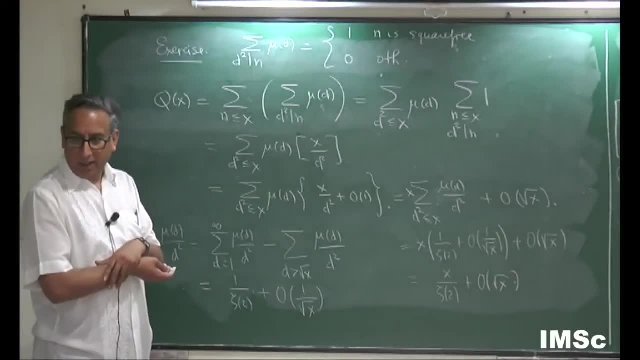 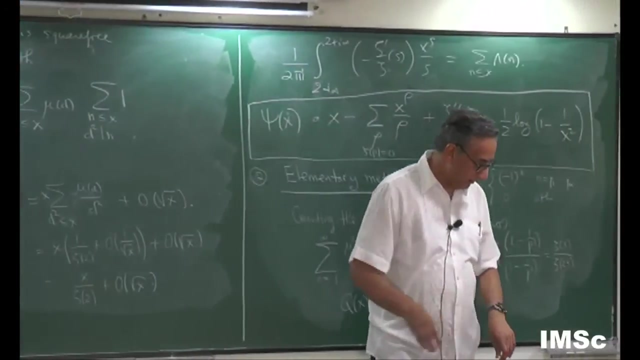 so that's why you shouldn't downplay. I mean, there's nothing high or low about anything. this is an elementary method. it has its value and it can be used to get good error terms. Okay, Now there's one more comment, if I may take a little bit of time. 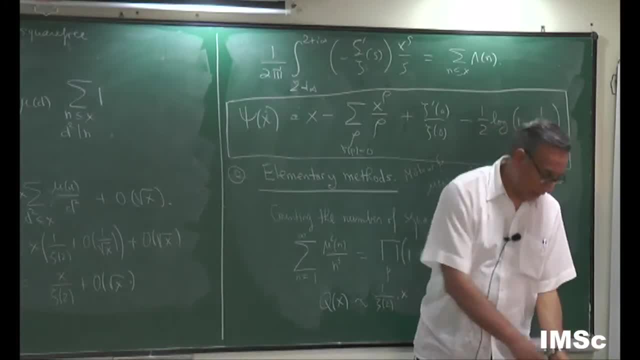 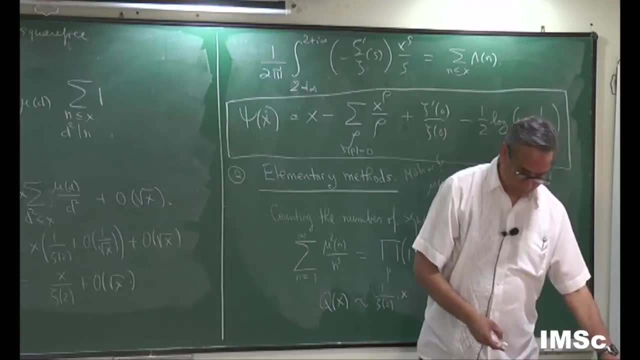 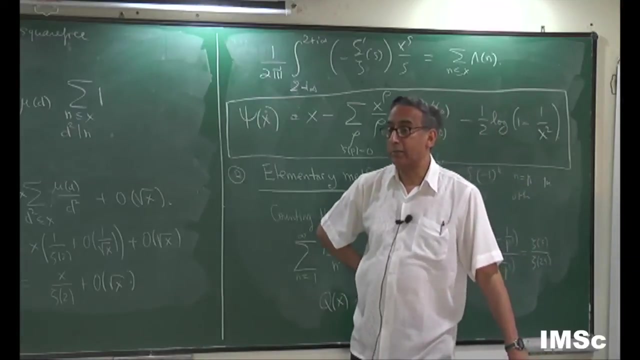 to discuss. that has to do with the question that Sumit asked last time about higher order poles. if you had more poles, could the TAR thirst theorem be used to get as the formulas? then the answer is yes, but you need a little trick to do that, and so I want to show that. 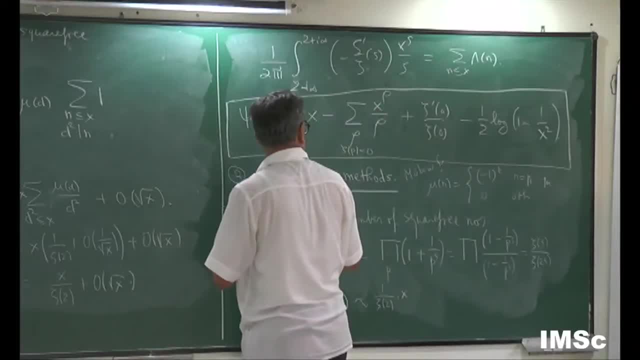 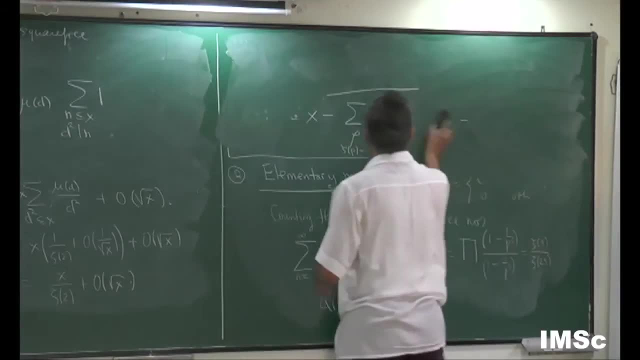 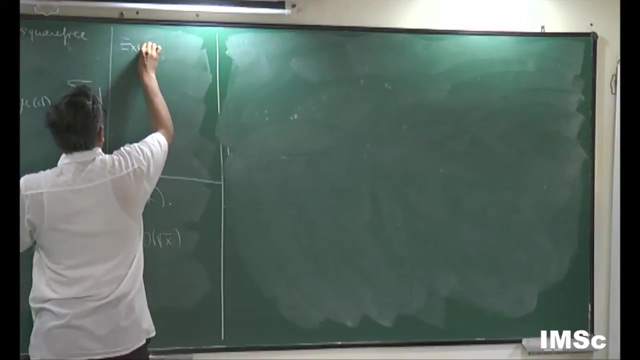 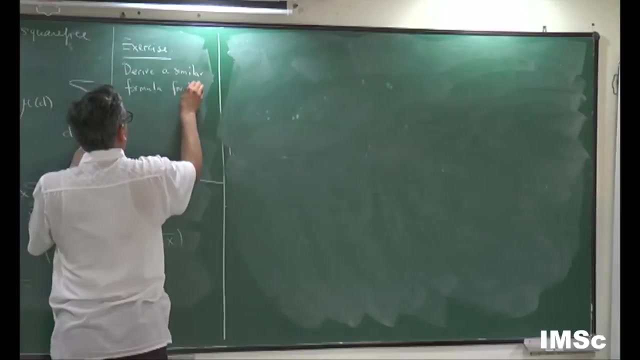 trick to you. maybe do that now. so let me just say question. oh, by the way, you may. since I did this example, let me just give you an exercise. homework problem. exercise: derive a similar formula for the number of square full numbers by using elementary methods. 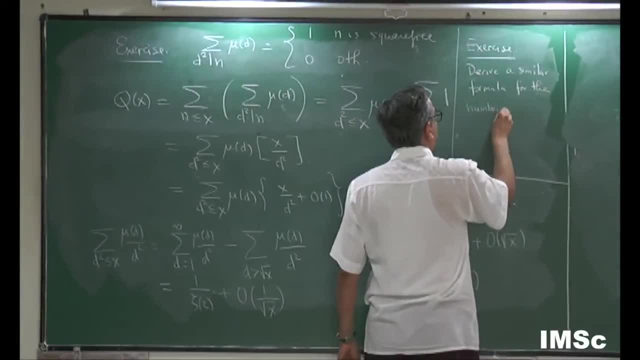 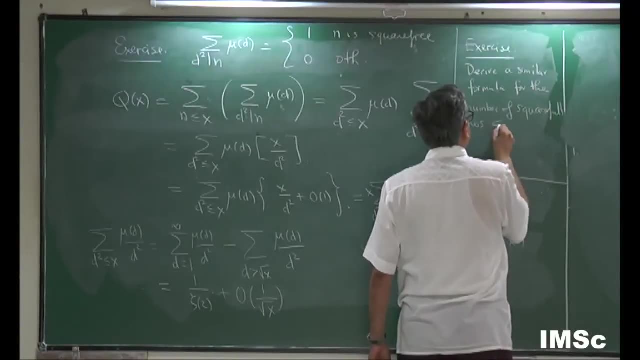 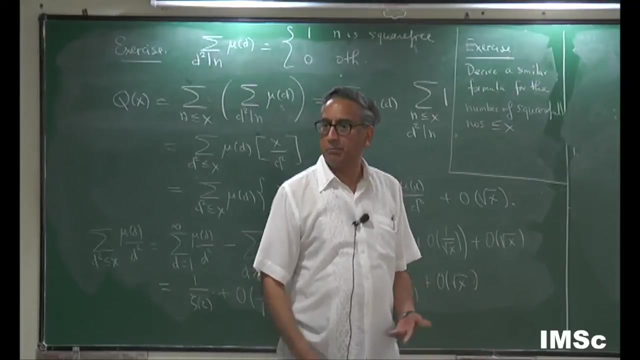 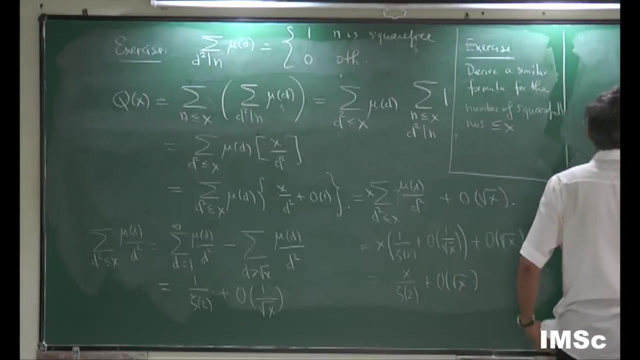 number of square full, So do the square full case. remember, last time I showed you how the Tauberian theorem can be used to give the main term. but now try and do it by elementary methods. you will get a better error term actually. alright, that's a good exercise now. so the question: 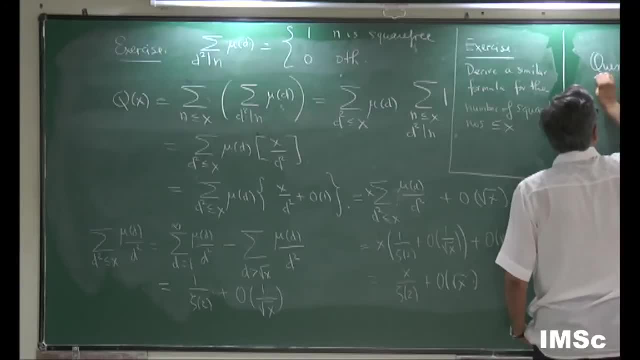 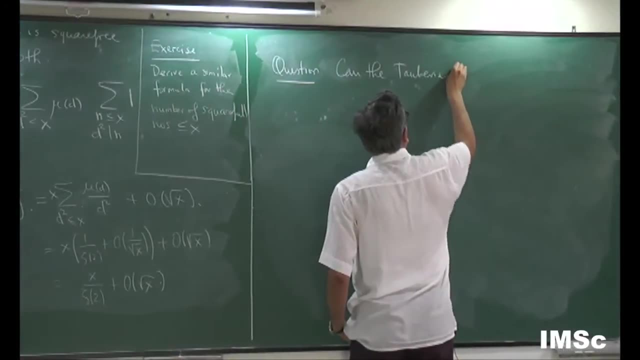 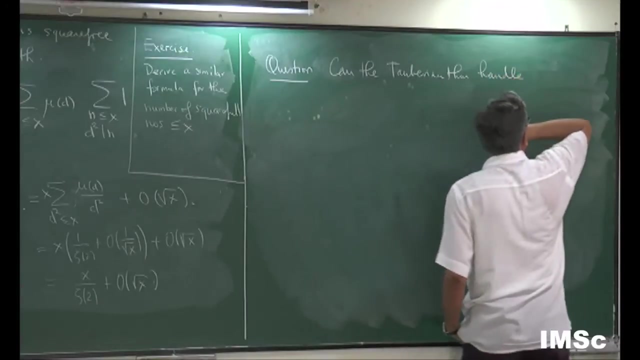 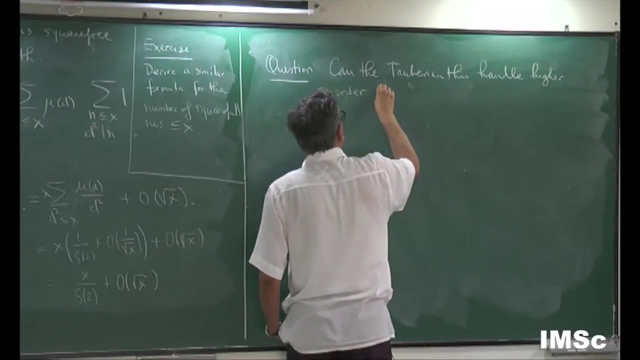 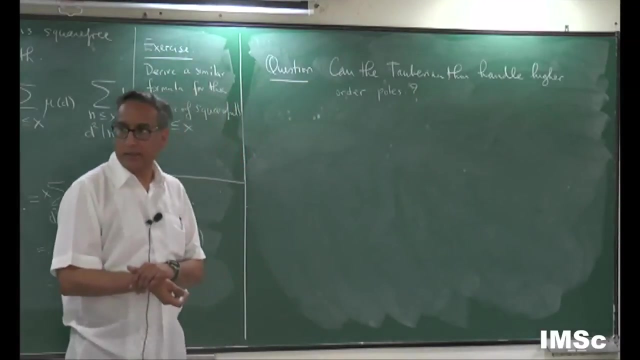 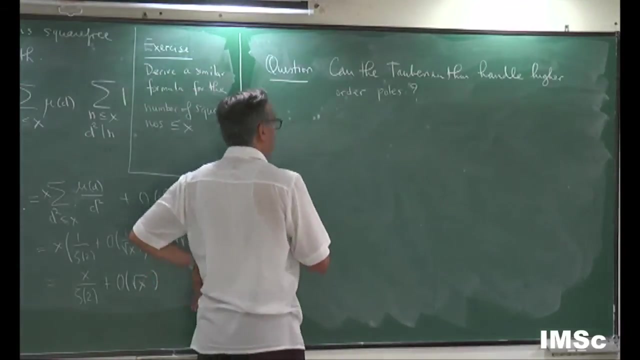 is: can the Tauberian theorem handle higher order poles? well, I, I am going to say that it can, and you have to understand how to do it, that's all. So remember, there are these conditions about the application of the Tauberian theorem. 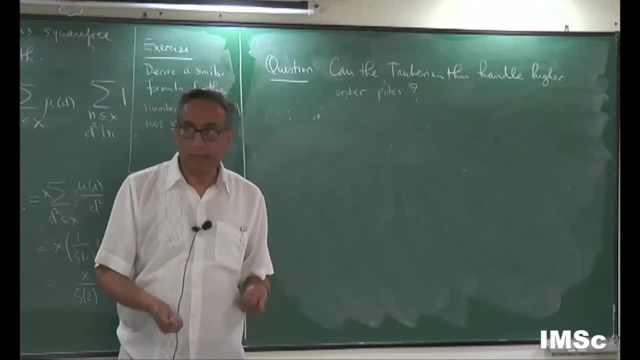 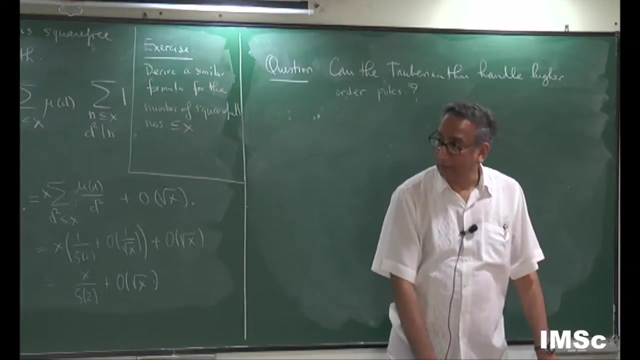 So what did we prove so far? You give me a Dirichlet series bn over nvs. okay, Suppose it has analytic continuation for real part s bigger than or equal to 1, bigger than or equal to 1, with, except for a simple pole of s equals 1, then summation bn is asymptotic. 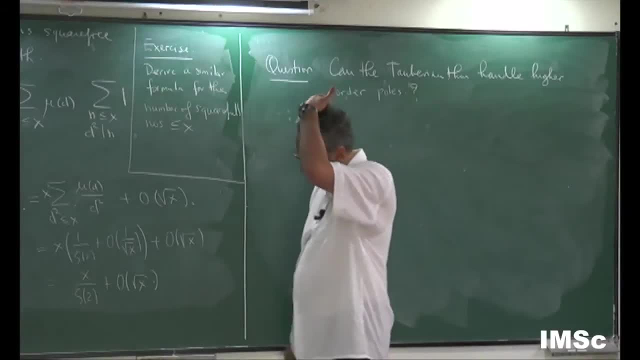 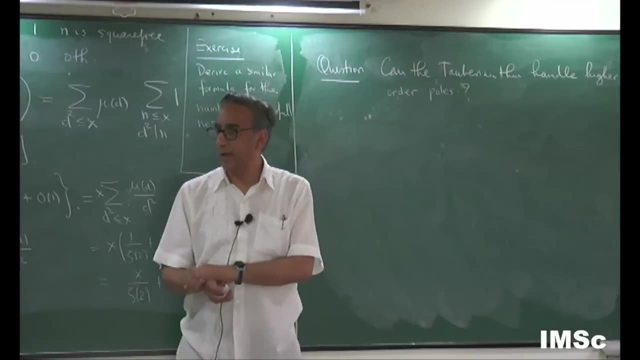 too. That's what we proved so far. okay, But remember, the bn has to be dominated by some an, which was again an, was supposed to have non-negative things and for which the Tauberian theorem was true. So you have to check the conditions of the Tauberian theorem. 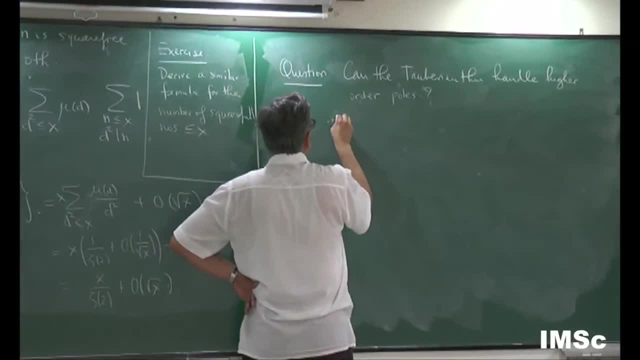 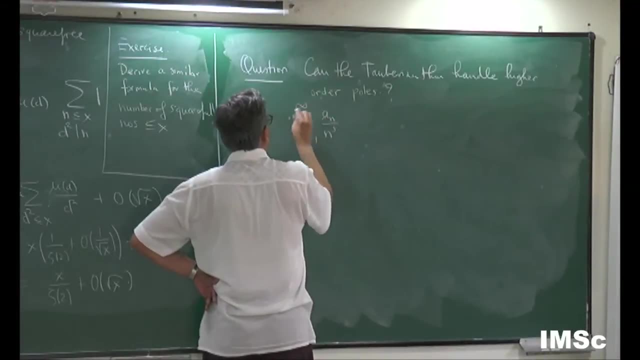 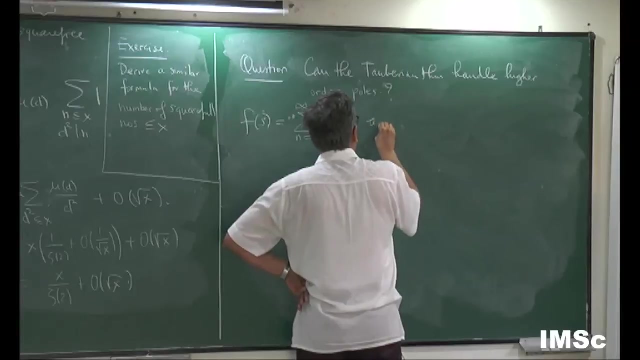 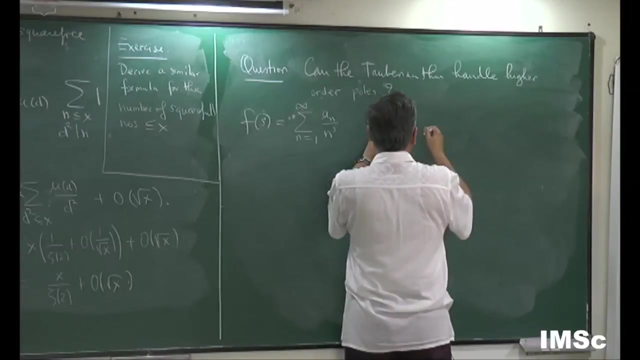 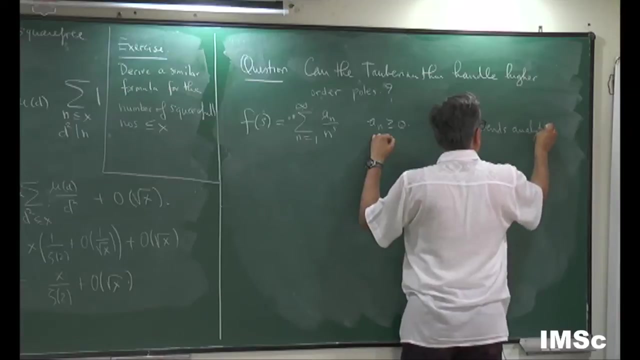 So, supposing I have a situation where I have an over nvs like so And ans equal to 1.. Of course, our non-negative and f of s extends analytically for real part s bigger than or equal to 1.. 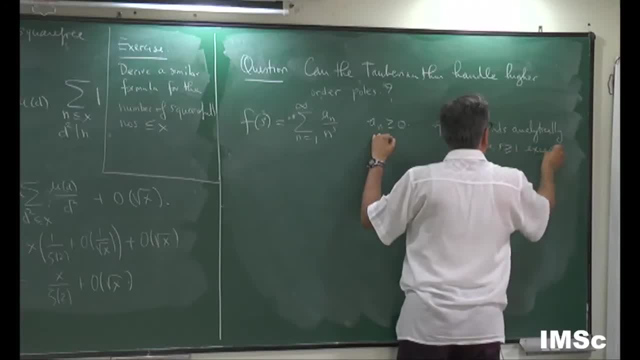 Except for a simple pole of s equal to 1.. So you have to check the conditions of the Tauberian theorem. So you have to check the conditions of the Tauberian theorem And s equals 1 where it has a double order pole. 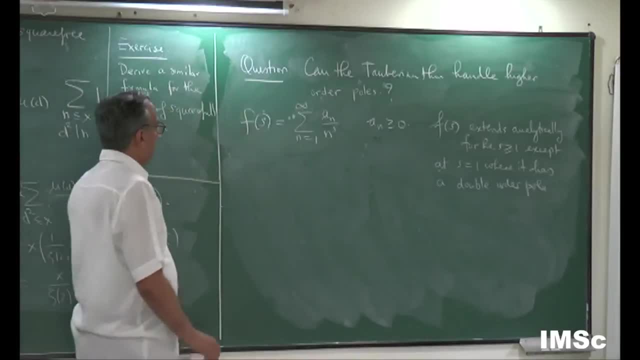 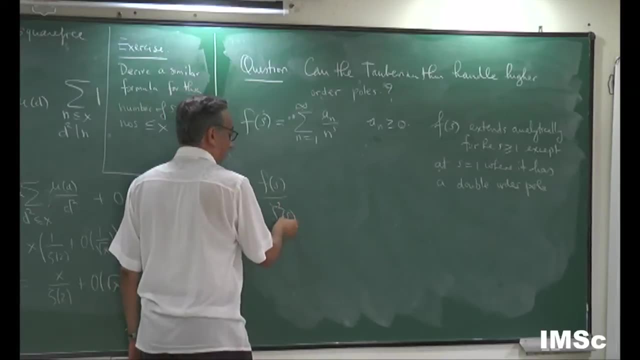 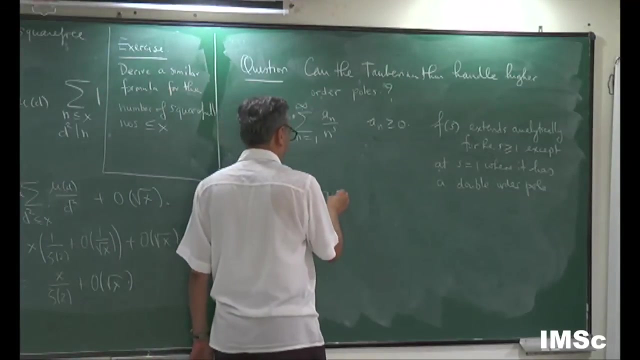 Double pole. Then what I do is I take f of x and I divide by g the Riemann's zeta function squared so that I cancel the pole and I get another Dirichlet, series g of s call it. and so let's say that's bn over mds or something. 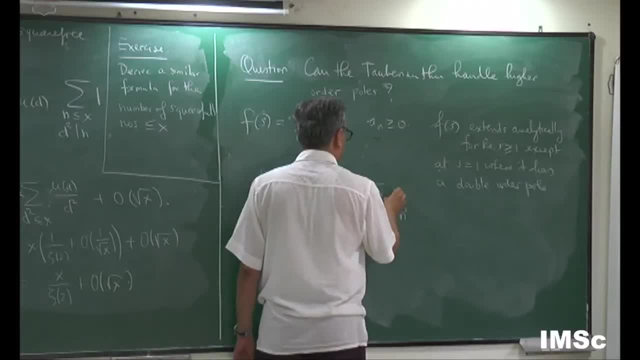 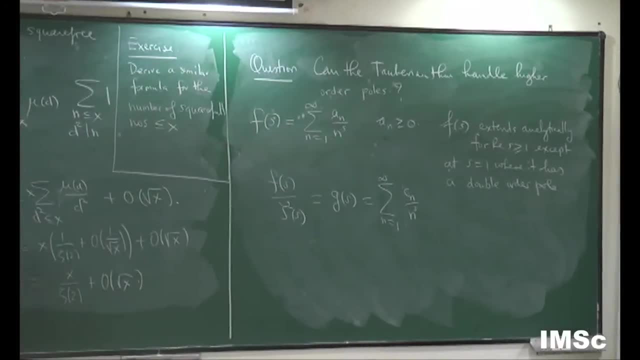 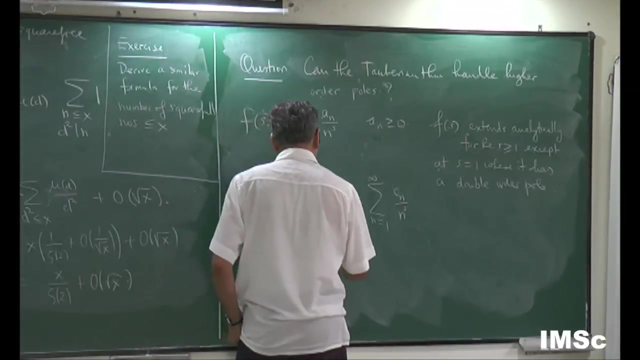 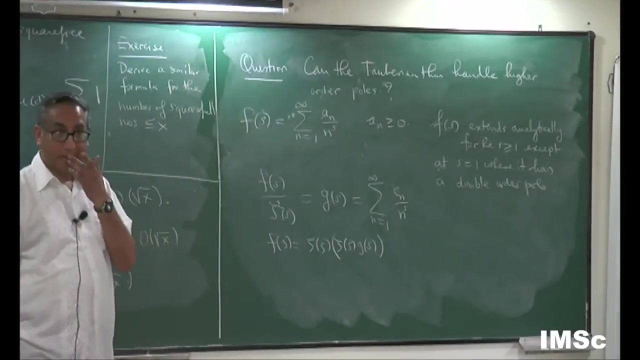 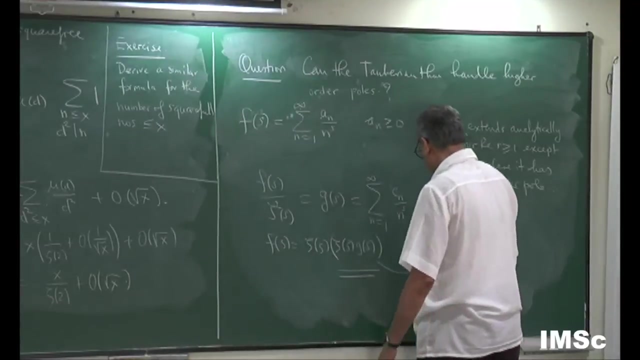 Let me. let me say it's cn, cn over mds, Okay, And what you could do is you could tech check. let's see, F is equal to zeta s, zeta sgs, and you can check. so you write this guy as summation: bn over mds g, remember? 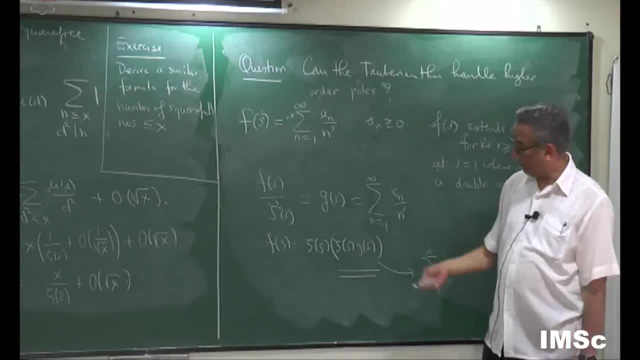 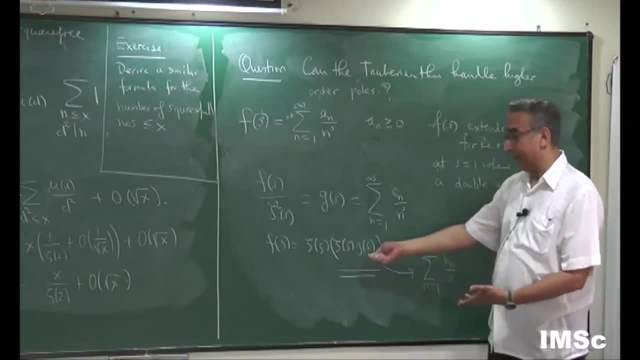 is analytic now for all of them over the place. real part is bigger than or equal to one. Zeta S now only has a polar S equals one. This guy is now analytic, except for that pole And it looks like this part of the thing. 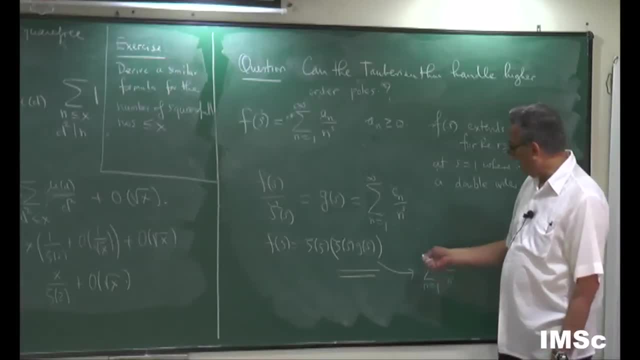 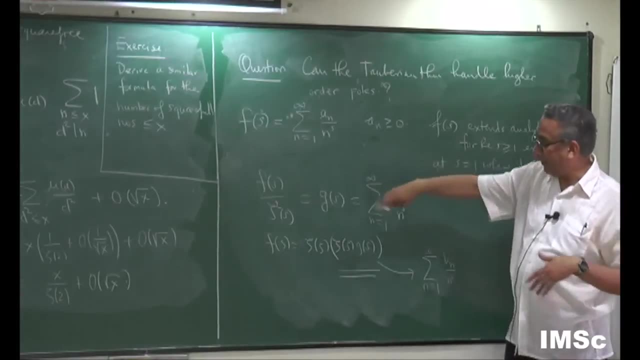 is perfectly poised for the Tauberian theorem. So, but you just have to check the BN satisfy the conditions that we want, that it's dominated by some ANs, not that AN but some other. you know that it satisfies. 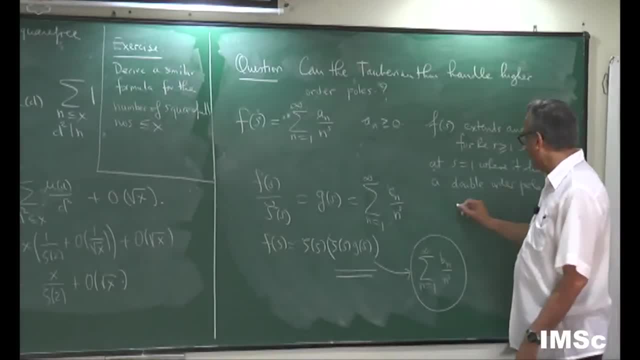 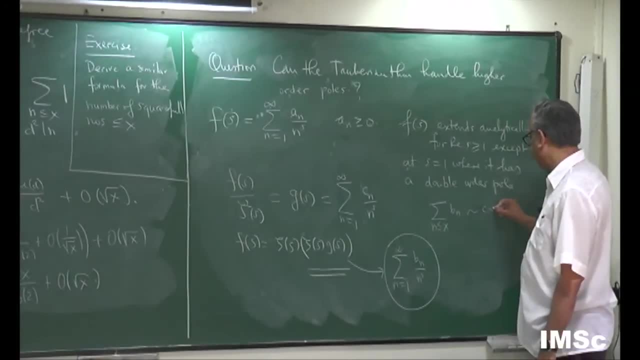 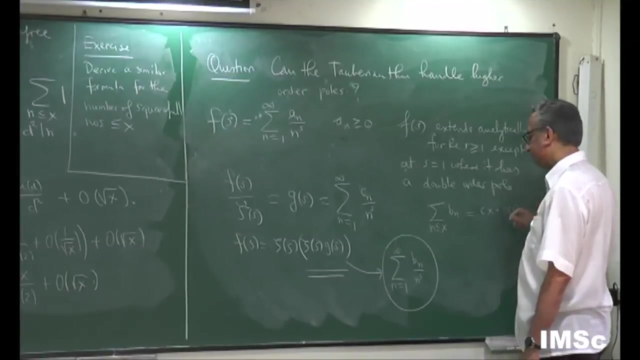 So you could try to apply the Tauberian theorem on this and you would get summation BN. N less than X is asymptotic to some constant X or, written differently, little o of X. Okay, But you're really after summation AN. 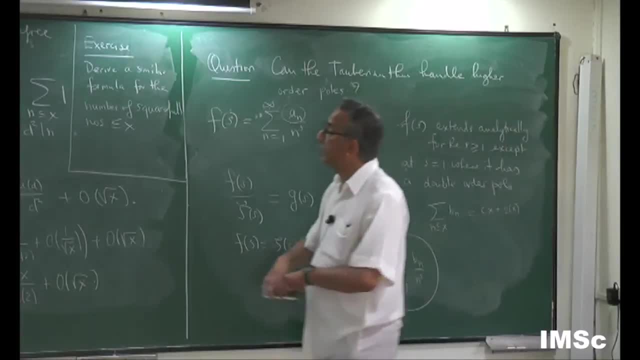 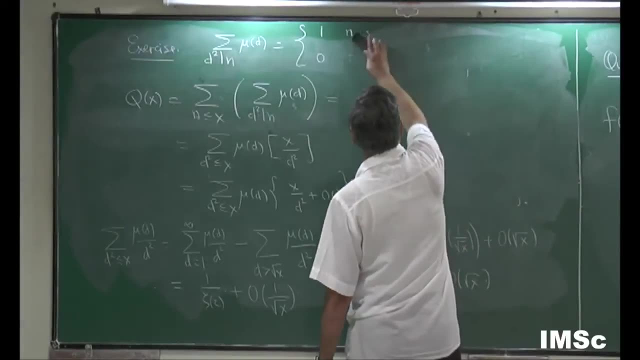 You're really after those guys. So what you do is you you think that the A and B are notски systolic? We don't know how they work. It's just that you can't explain what we know. Well, let's write out the histograms. 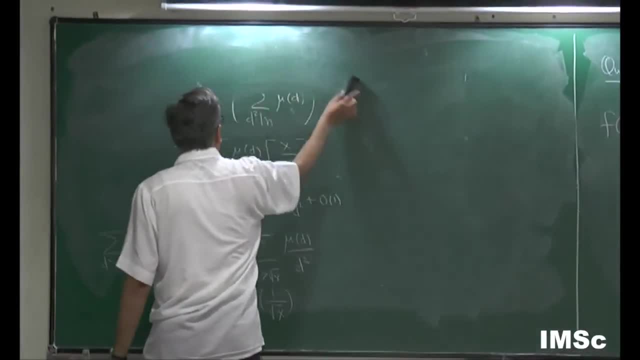 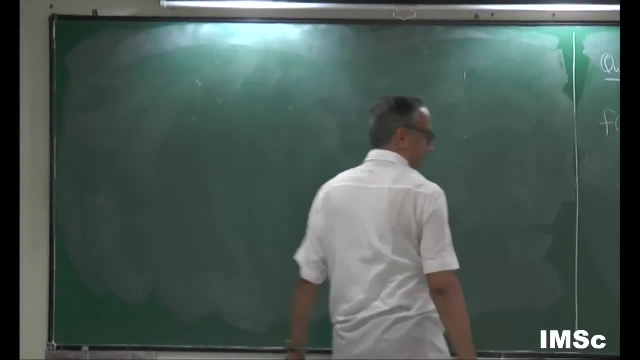 and then if you just write them down and you'll just do the same thing again, Just say: here is what you have, So this is the vector for N, Then we can write down the second vector for B. So we're going to write down the third vector for B. 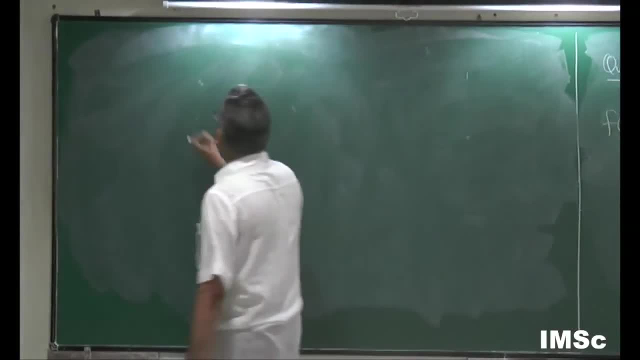 And then write down the last one. and then let's write down N. I'm just going to write down the last one because I want you to keep that in mind when you're doing these. So if you do this, you'll get like: 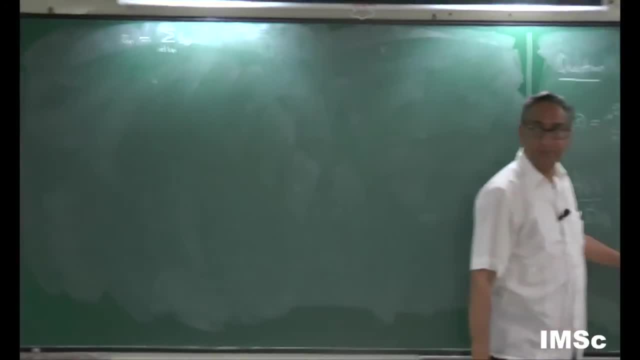 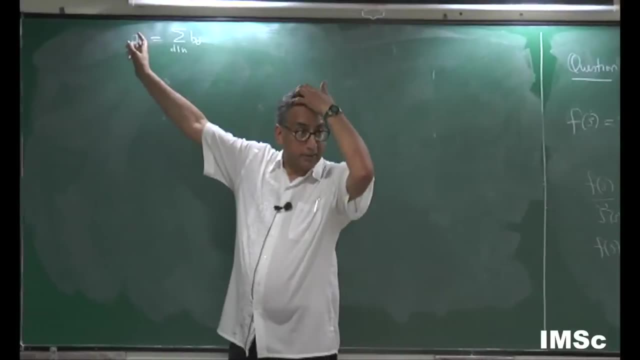 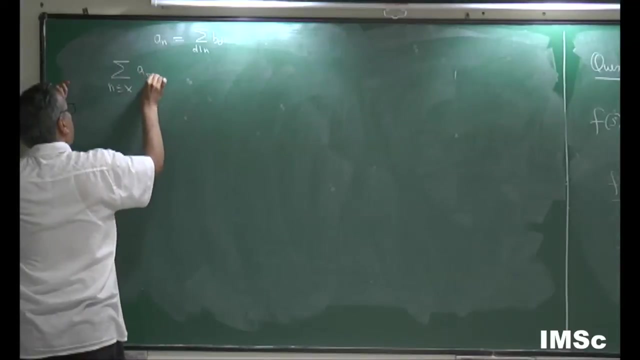 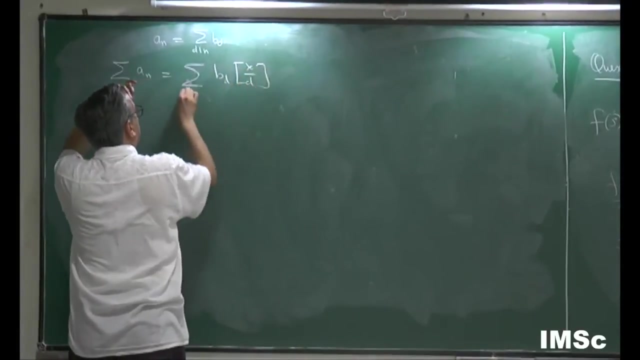 that's coming from this product, zeta s times. this guy can be translated as: an is equal to summation d divides n, b sub d. So therefore, summation an n less than x. summation an is now equal to summation bd x over d by, just by doing the, just putting that thing in. 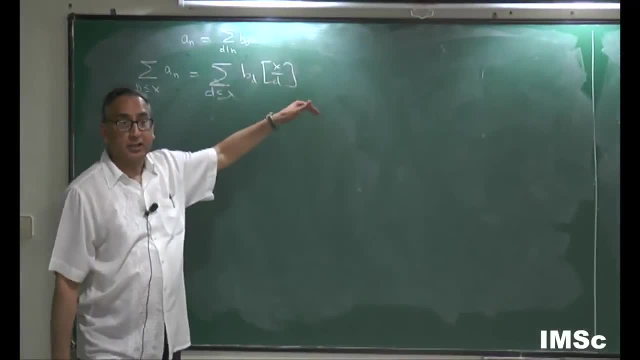 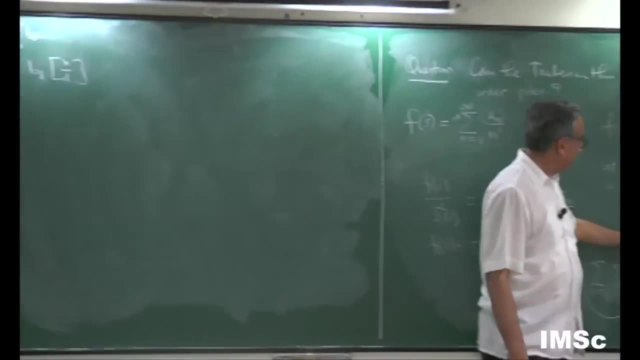 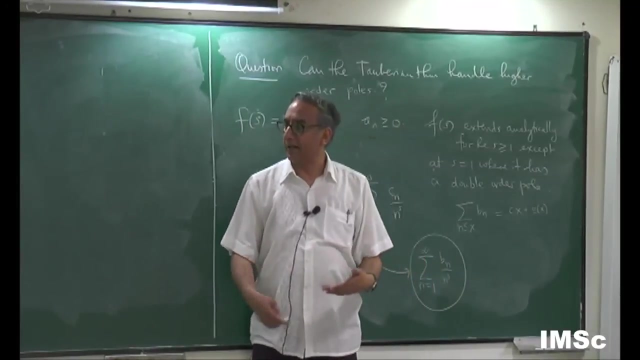 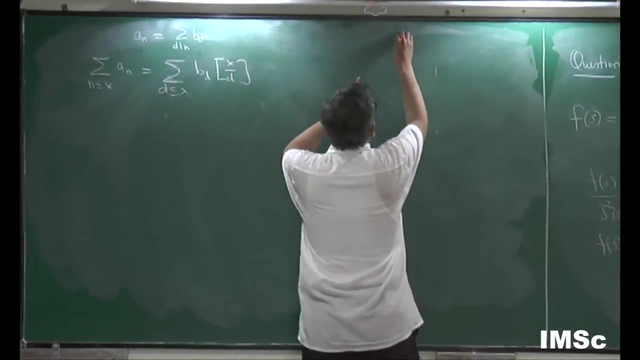 so writing this an here and then interchanging summation, you get this. okay Now, because you know that summation bn is a constant x plus little o of x. this is more or less saying that bn is like a constant on average. So by partial summation you can deduce from that that summation bn over n, n less than. 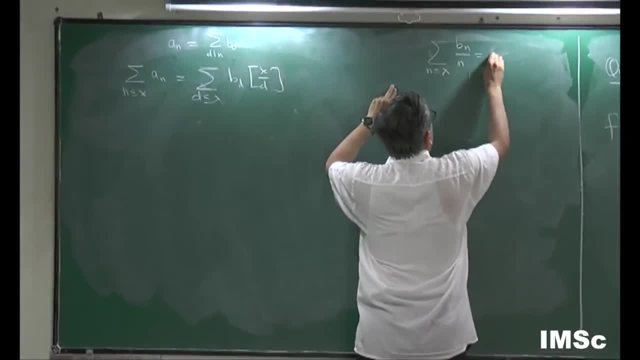 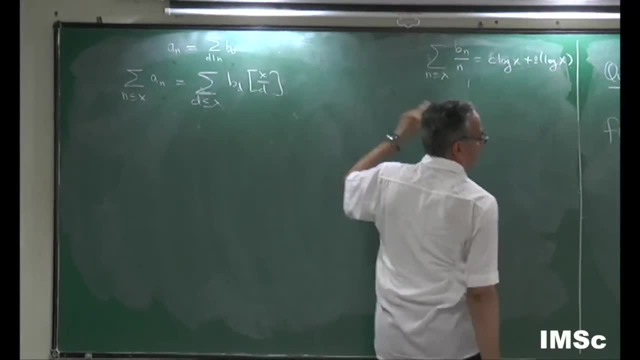 x is equal to summation bn. So this is equal to constant log x, same constant plus little o of log x. So I will leave that once you have this fact, you can deduce this fact by partial summation. 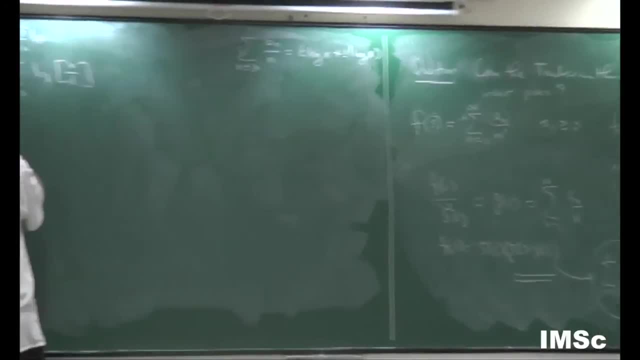 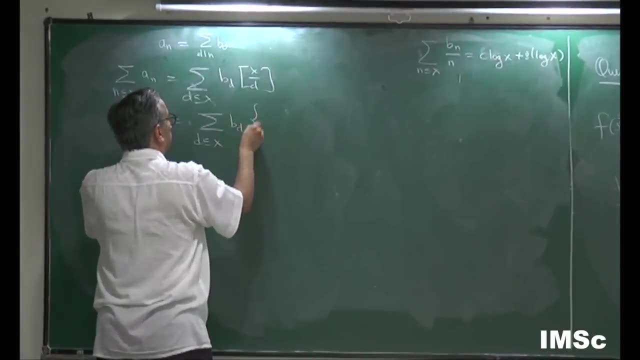 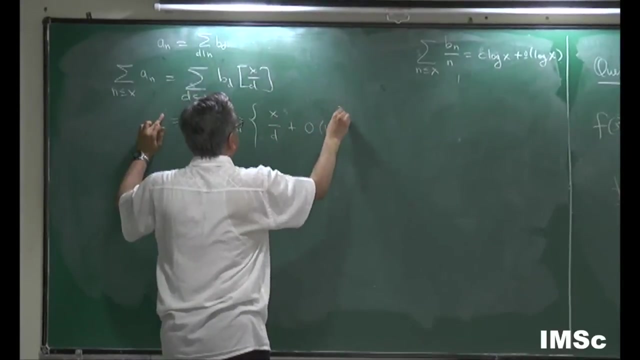 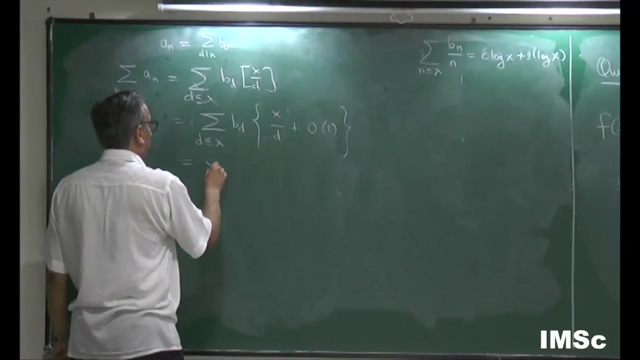 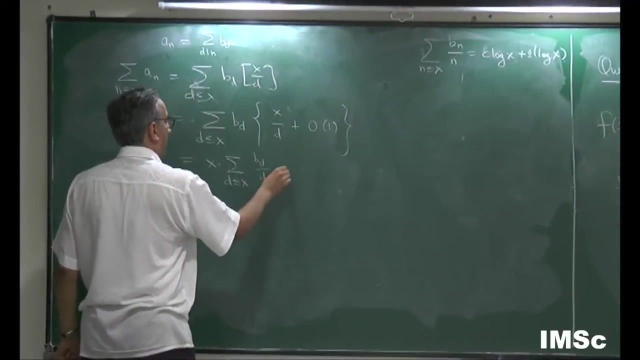 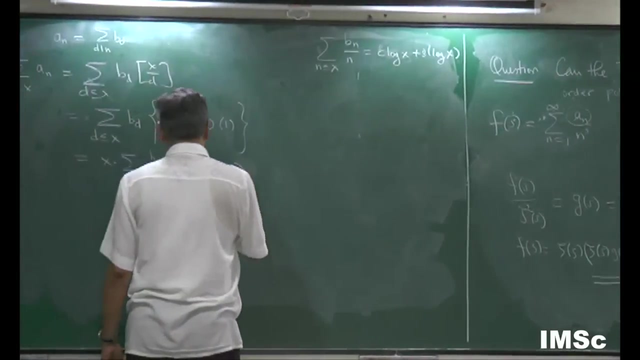 I will leave that to you, So that now it looks as if I take away I will leave that to you And then this becomes d less than x bd over d plus o of summation bd. but summation bd is like o of x, so it is an o of x there. 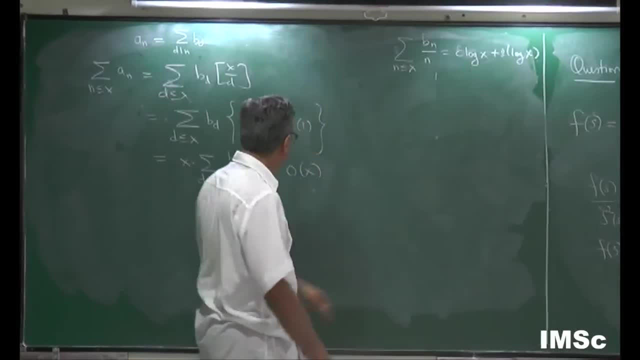 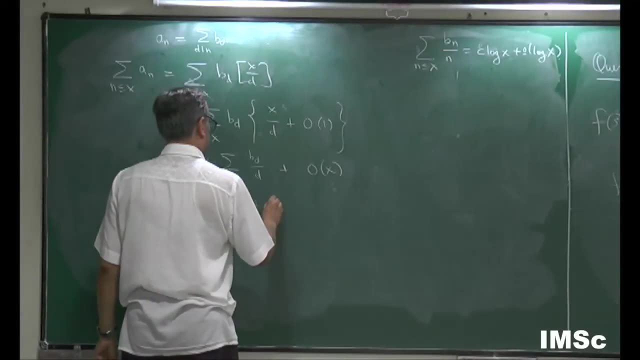 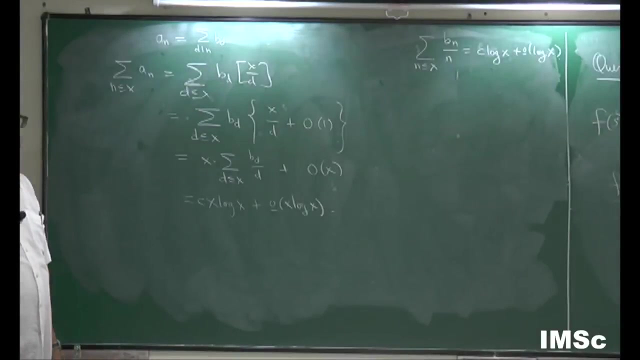 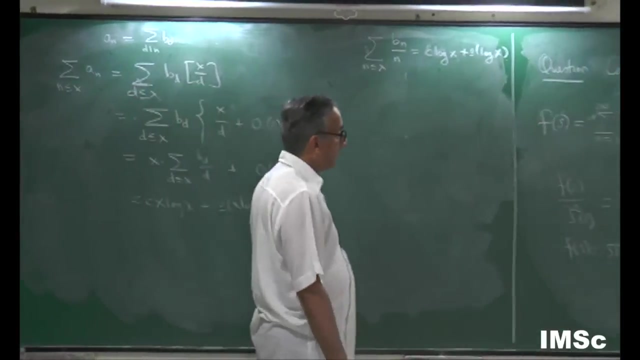 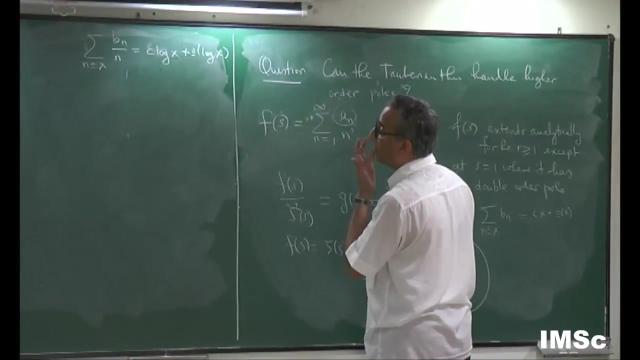 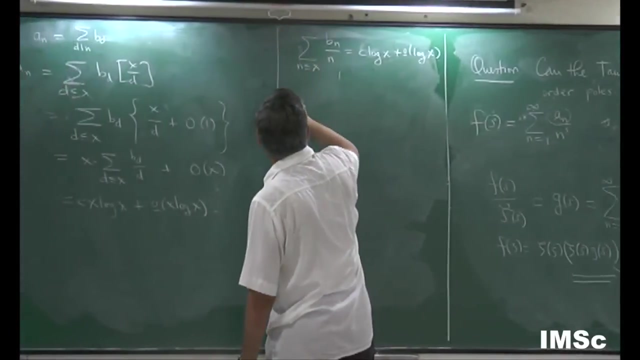 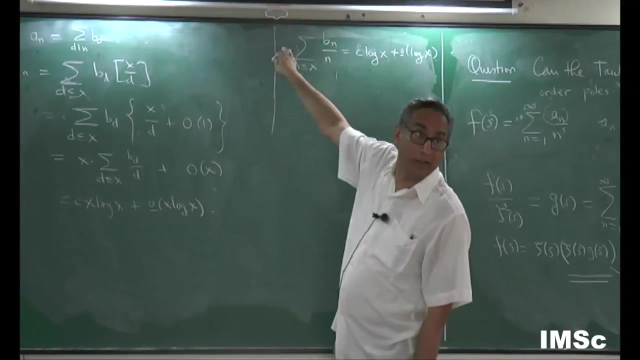 And then by partial summation you have this. There is a small issue here if you try to prove this by your partial summation trick. there is a small little trick there in this question, but I am sure you will figure it. 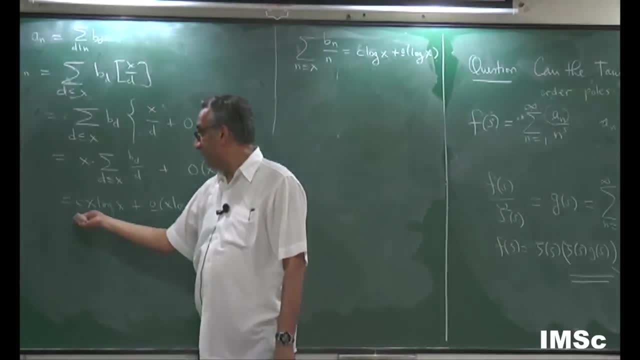 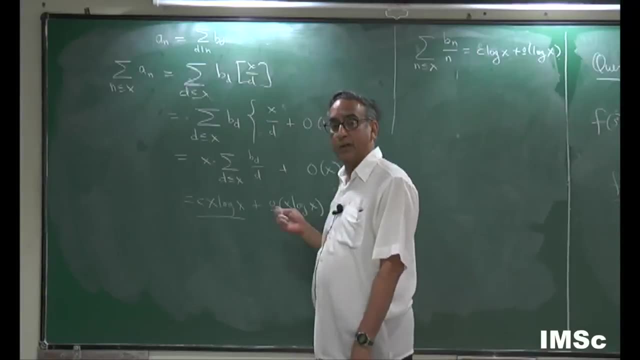 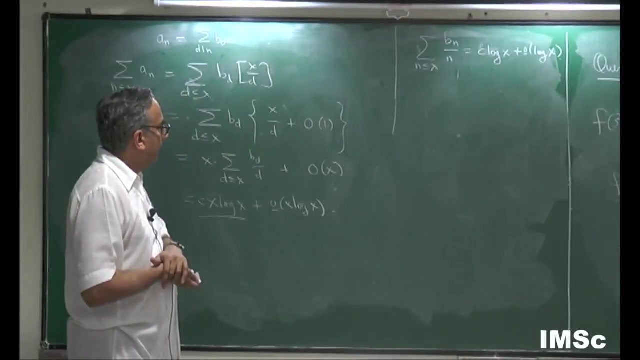 out okay. So that is basically how you could get, but notice that it only gives you x, log x, and it does not give you the next term. It gives you a very crude error term. All right, And of course you can continue this procedure for higher order poles.